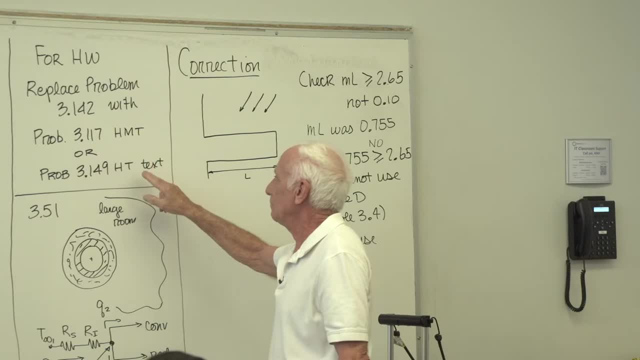 it's problem 3-117.. If you're using what's called the heat transfer introduction to heat transfer textbook, that's problem 3-149.. If you're using the introduction to heat mass transfer textbook, it's the same problem but it's called problem 3-117.. 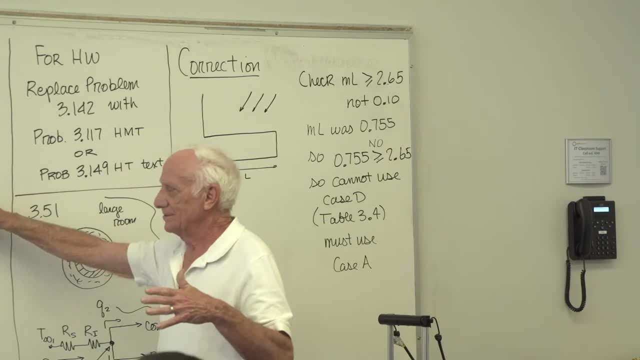 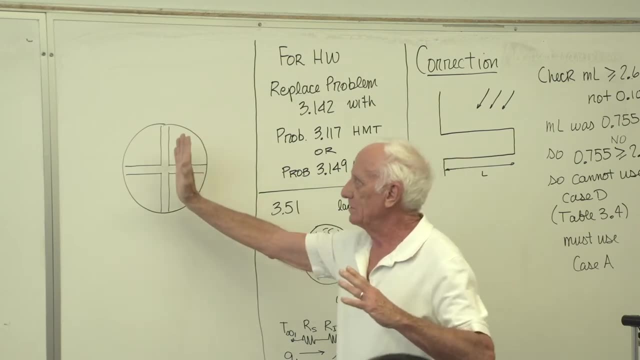 The picture for that problem looks like this. So just to make sure you're working the right one, it looks like this: It's a tube with baffles in the tube. Come out this way, come out this way baffles. This separates, so the flow goes in four channels along the tube. 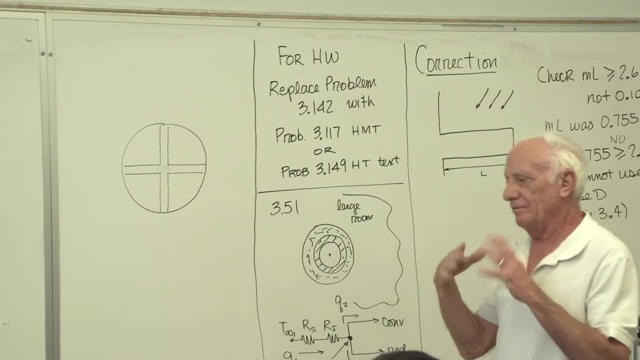 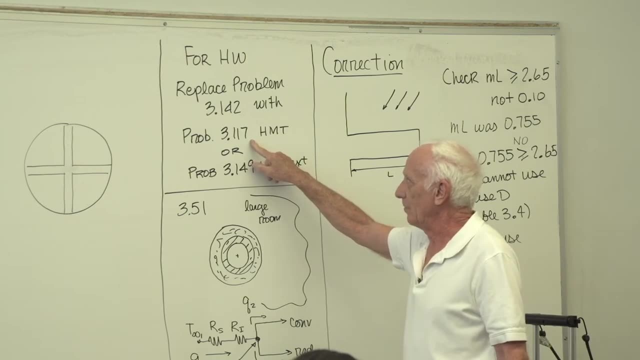 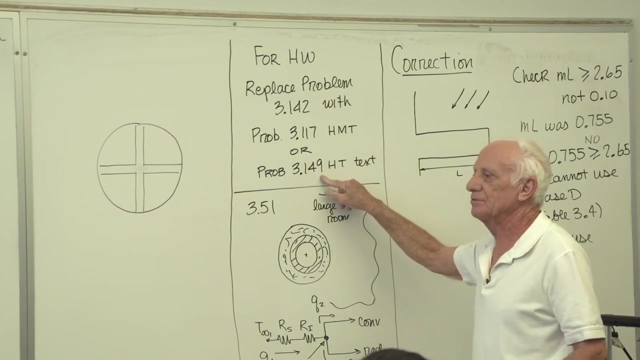 four separate channels. So if you're confused about that, go to that picture and you'll find it at the end of Chapter 3 for homework. One textbook has a problem 3-117, the other one has 3-149.. They're the same problem, just renumbered for different textbooks. 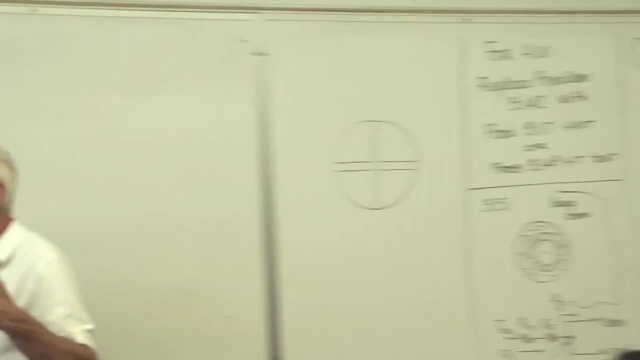 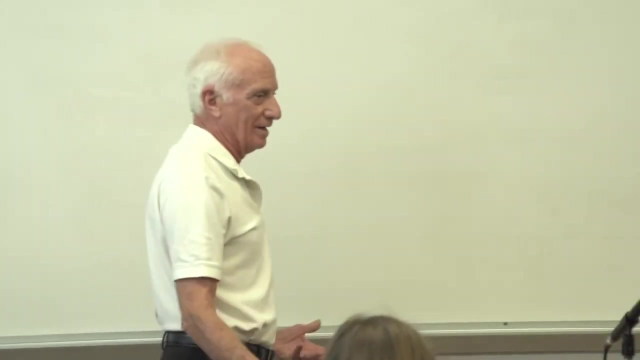 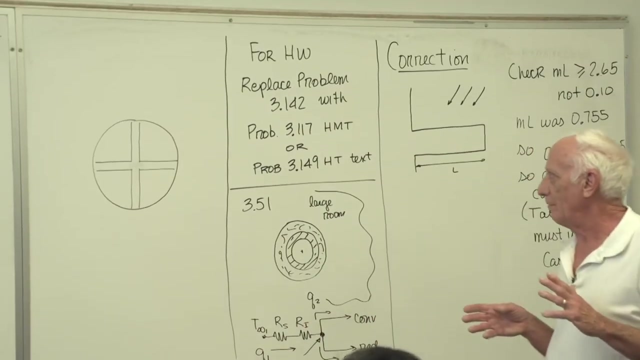 If you don't have a textbook and you want that problem, take out your cell phone, take a picture after class in my textbook and you can get it. that way I'll show you exactly which one it is in my textbook. Just a hint for problem 3.51.. 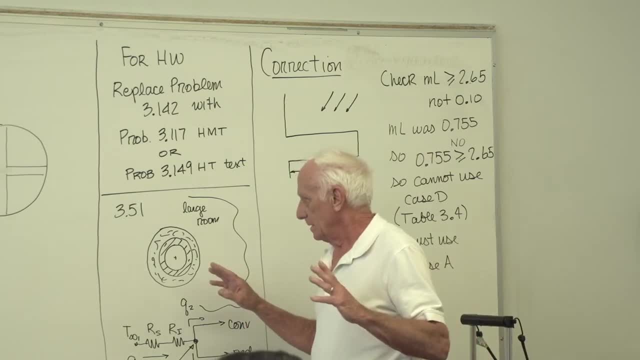 It's a steam pipe in a power plant. The steam pipe is steel, surrounded by insulation, carrying steam, of course, in a large room where the air temperature is given and the room wall temperatures are given. So you know what's going to happen. 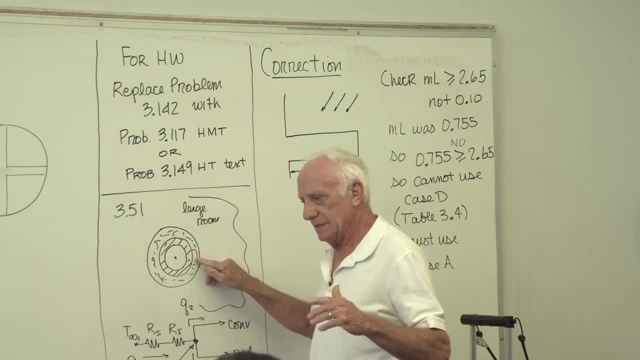 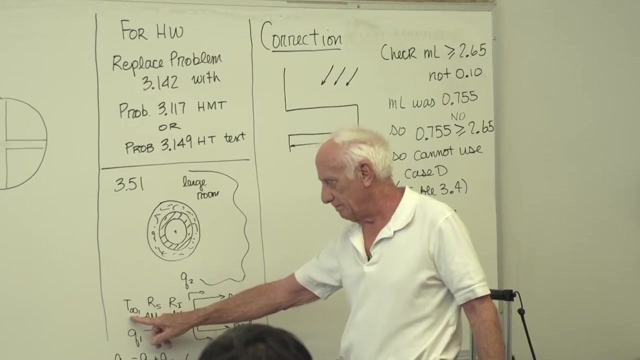 The heat goes through the steel, it goes through the insulation, it goes out either to the room walls by radiation or to the room air by convection. So here's your picture of what's happening. Steam in the pipe, T-infinity one. The heat goes through the steel resistance, it goes through the insulation resistance. When it gets to the outside of the insulation it splits. Some goes to the room air by convection, some goes to the walls of the room by radiation. You don't need to use resistors there because they're difficult to use for radiation. 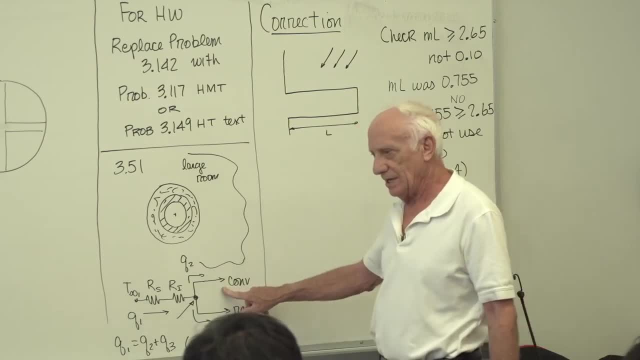 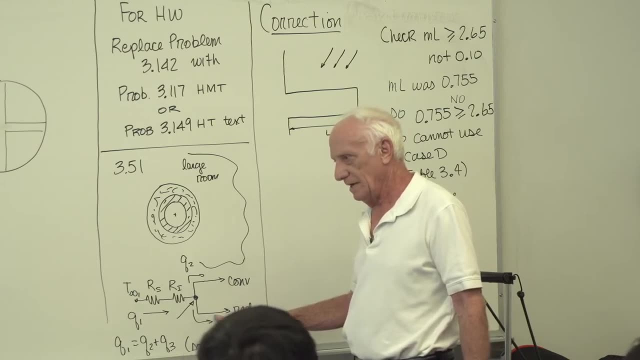 So just show them as this: You know what this is. This is HA delta T. You know what this is, Chapter 1.. It's Epsilon, Sigma A, T surface to the fourth minus T walls to the fourth. So now you write an energy balance on this big black node. 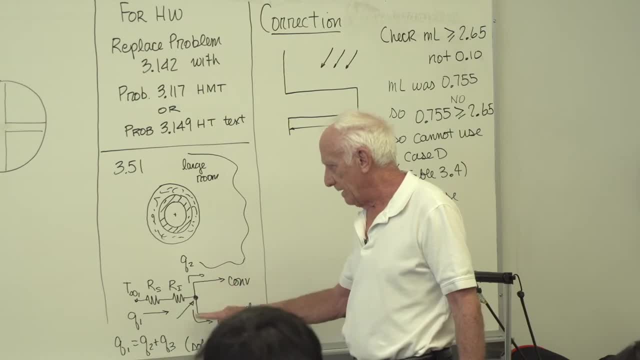 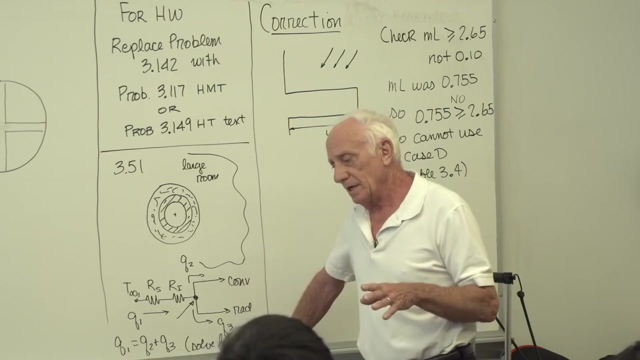 The heat that comes in by conduction is carried away by either convection or radiation. The only unknown in that equation is going to be R3. The outside radius of the insulation. Now you can try and solve it analytically. It's a little bit tough because there's a natural log of R3 in here. 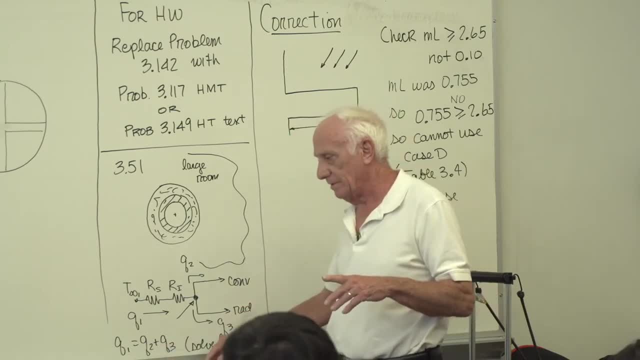 and there's also R3 on the area for convection and radiation. So it's a little tough. What you can do if you want to avoid that is you play the iteration game, the guessing game. Now, first of all, make a reasonable first guess. 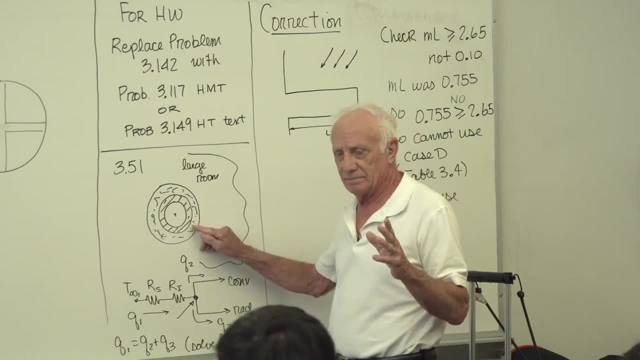 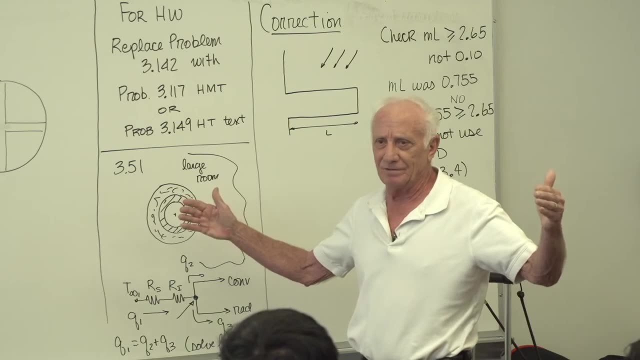 Well, they tell you the radius of the steel pipe. They tell you that. So okay, you're going to add insulation to it. How much? Three feet? I don't think so. No, no, no, Half an inch. 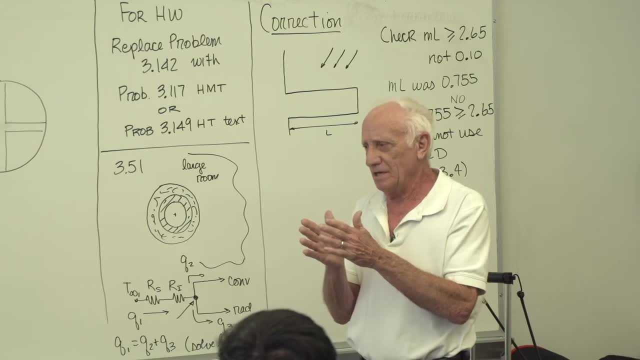 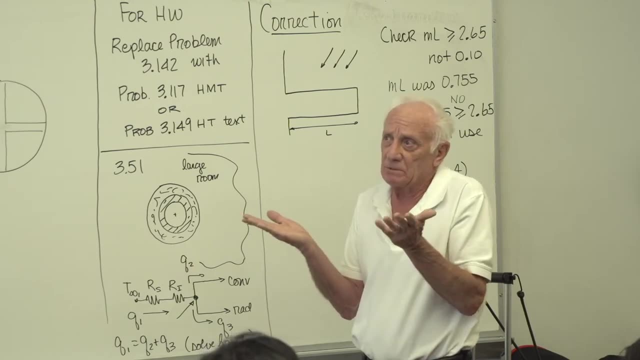 I doubt it. No, I don't think so. My first guess is going to be maybe an inch or two. An inch is two centimeters, So maybe I don't know. I'll guess between two, four, five, something like that. 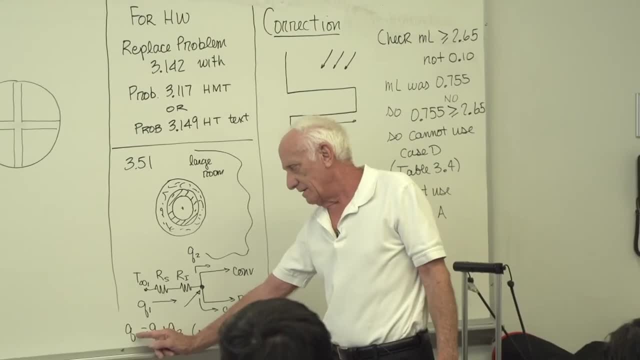 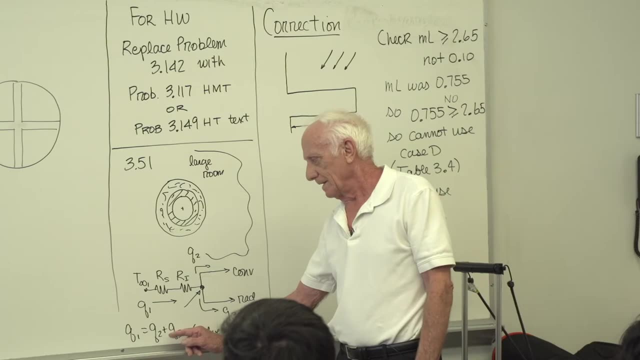 I'll put that R3 in that equation If the left-hand side comes out to be R3.. If the right-hand side comes out to be different than the right-hand side, try, try again. New guess. I guess now R3 is this. 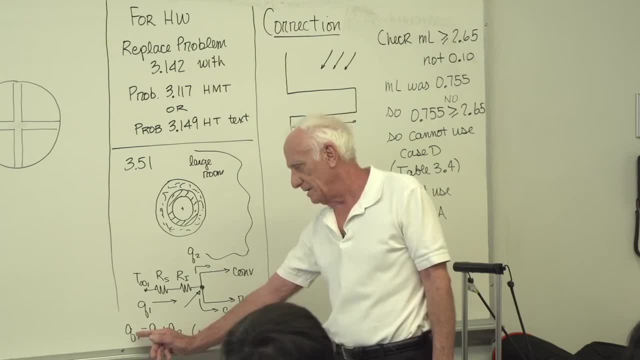 So you might put an R3 value in here and get Q1, 53. And this side Q2 plus Q3, 48. Say, oh, that didn't work. I'll make a new guess for R3. Okay. 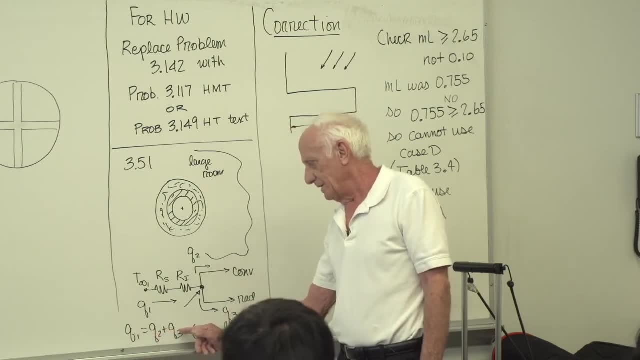 Now you get Q1 equal 51, and Q2 and Q3 still 48.. Say, I'm getting closer. Make a new guess for R3. Usually after about three iterations You get right in there and the left-hand side is 51 and a half. right-hand side is: 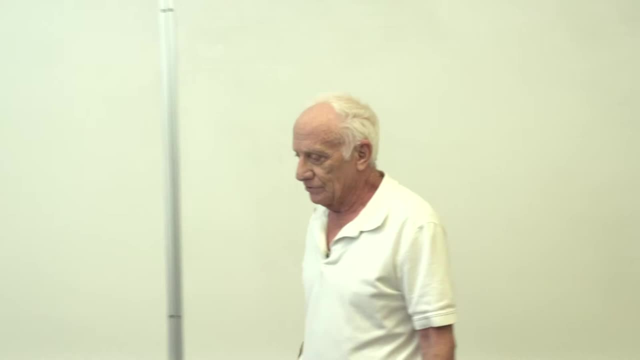 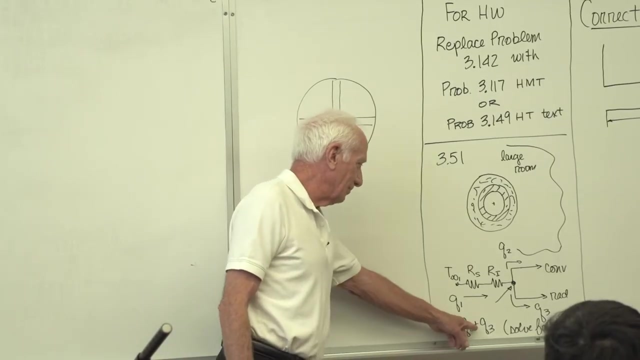 51.4.. Stop, You're done. That's close enough. So that's one way to solve that problem: by iteration, Guess an R3 and see if left-hand side equals the right-hand side. Okay, Any question on those guys then? 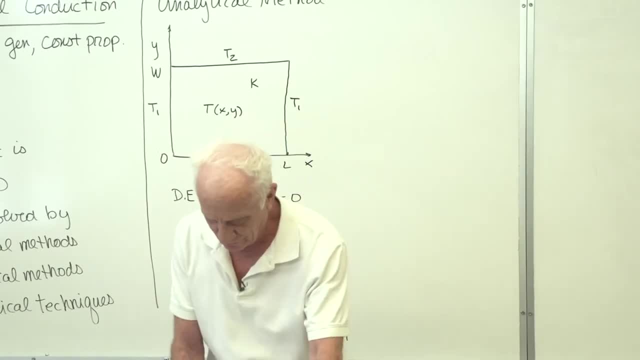 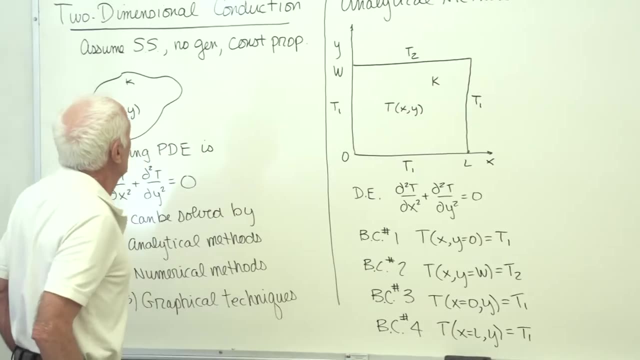 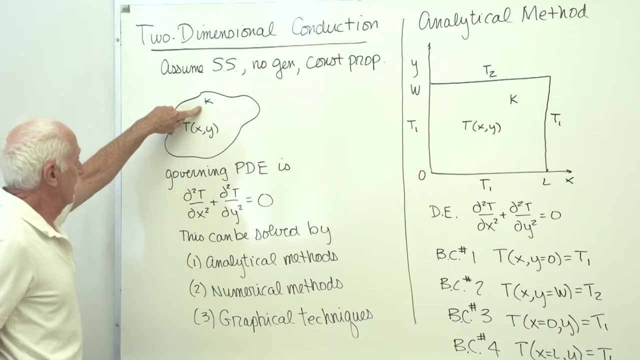 All right, Good, That gets us to chapter four. Now, All right, All right, So we're going to look at two-dimensional conduction. So here's a solid material conductivity: K temperature as a function of X and Y. First, 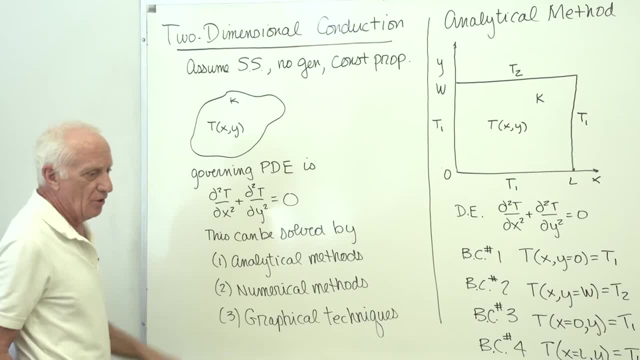 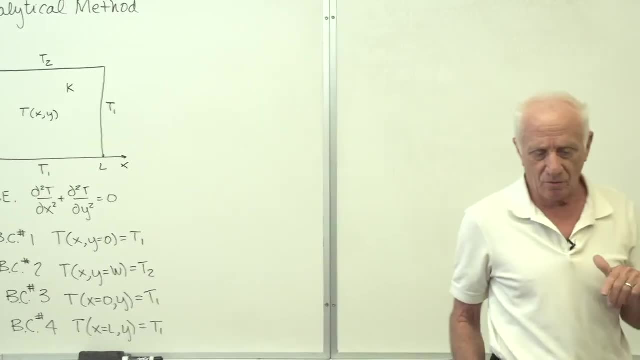 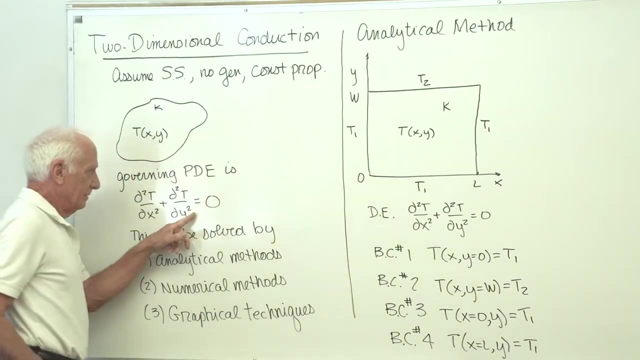 of all, we want to find the governing partial differential equation. We go back to chapter two, the heat diffusion equation in rectangular coordinates. Okay, It's two-dimensional, So get rid of that. All right, Get rid of the Z. There's a second partial T with respect to Z. That's zero. 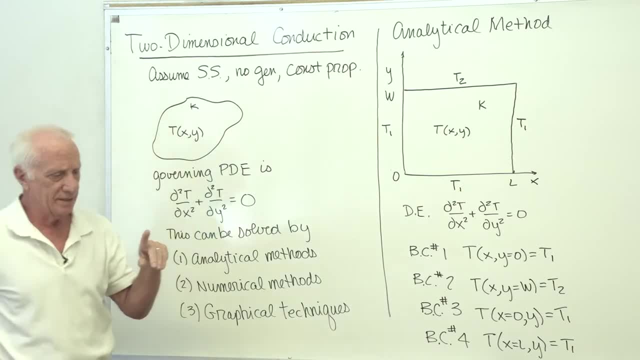 We're assuming steady state. Get rid of the partial with respect to T of temperature. Okay, It's gone. There's no generation. Get rid of the Q dot term in chapter two, heat diffusion equation- It's gone. Assume constant properties. 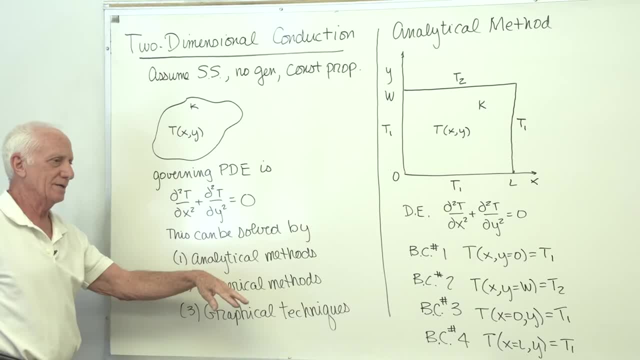 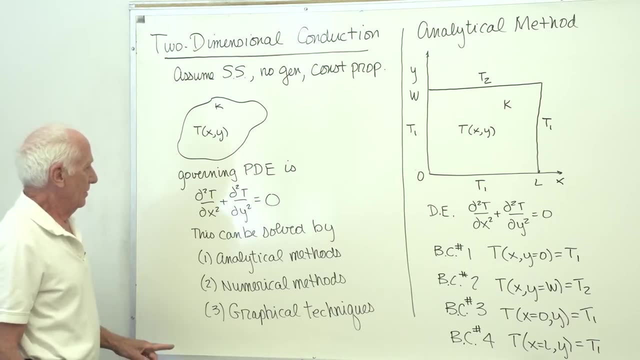 The K comes out, the partial sign You divide through by K- K disappears. We're left with the Laplace equation. All right, So you can solve this by a number of methods. The first one maybe, analytically, the exact solution. 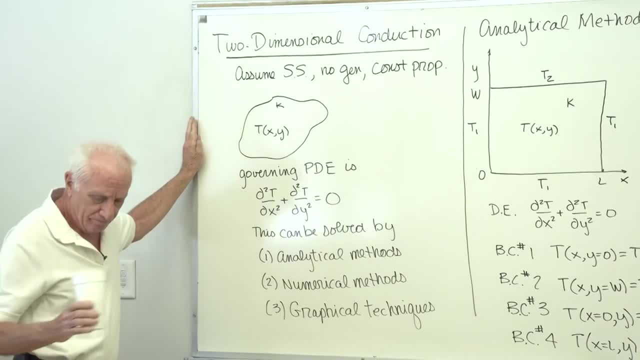 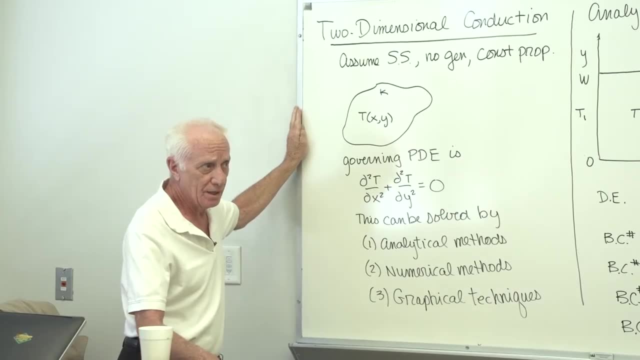 Okay, Maybe numerically, Sure, Sure, numerically, We'll do that on probably the last part of Friday and then Monday. Finally, we can get some good intuition and maybe some numbers for Q and temperature. Okay, From graphical techniques. 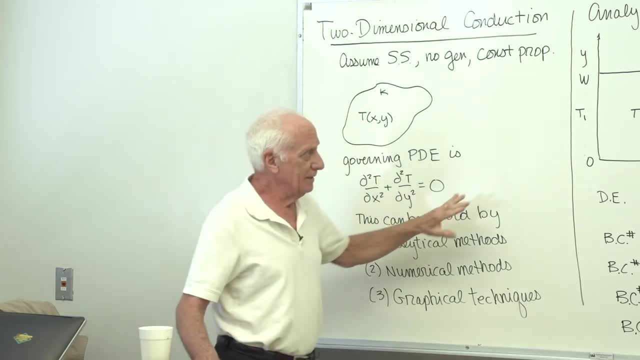 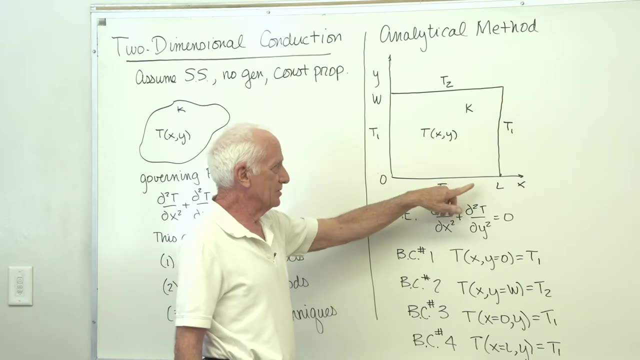 So three possibilities. The analytical technique is described by this. Here is a rectangular plate, The length X direction L, The height in the Y direction W. Maybe it's two centimeters thick. The thickness is out from the board. 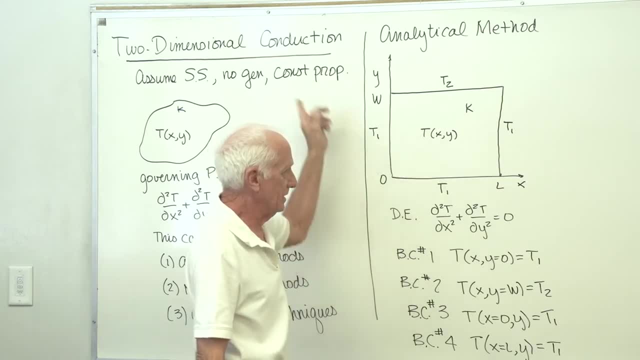 Okay, But we're looking at only two dimensions, X and Y two-D conduction. Okay, We're looking at only two dimensions, X and Y two-D conduction. Okay, In this equation, second partial T with respect to X, we need two boundary conditions relating. 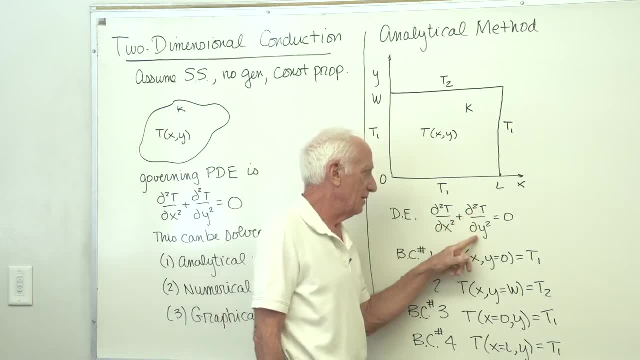 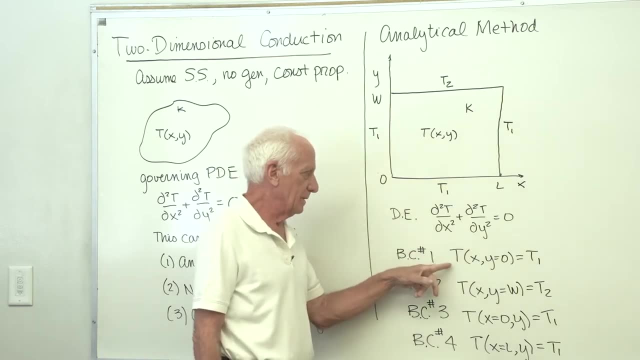 T to X. Second partial T with respect to Y. we need two boundary conditions relating T to Y. Here they are: BC number one, If I go to, Y, equals zero. the bottom, no matter what the X value is the temperature, is T1.. 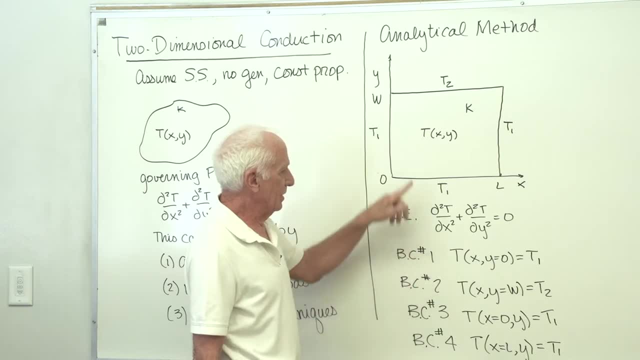 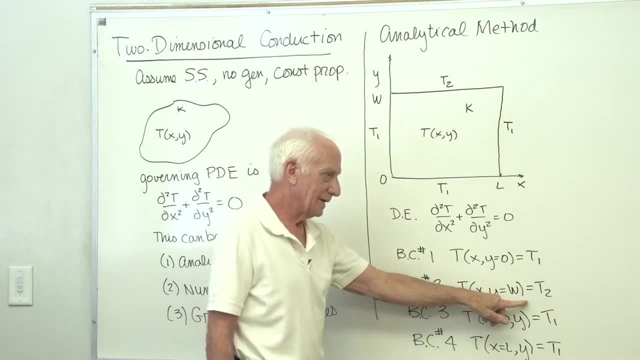 Okay, That's this one, BC, number two At the top. When Y equals W, No matter what X is, T equals T2.. Got it The left-hand side. When X equals zero, for any Y value, the temperature is T1.. 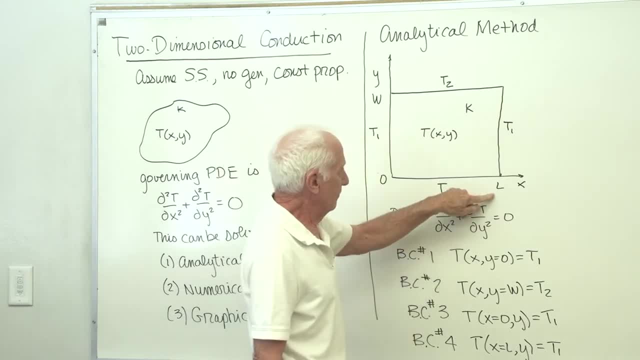 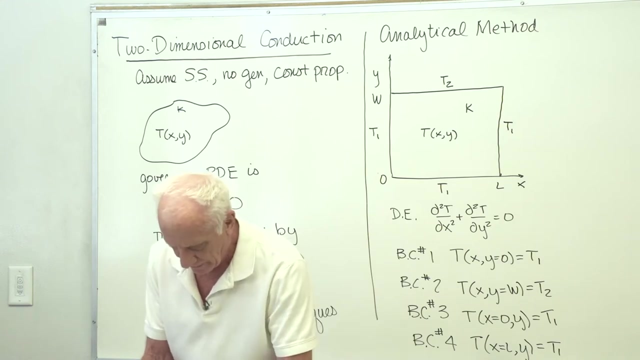 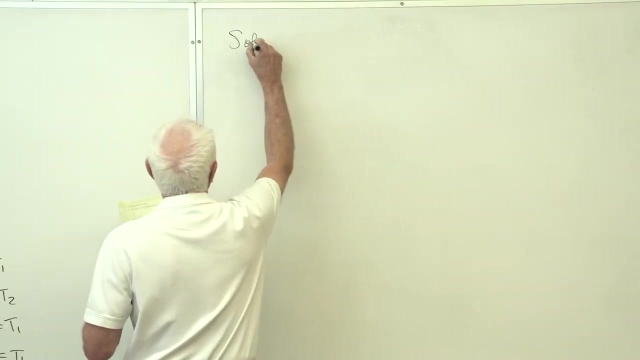 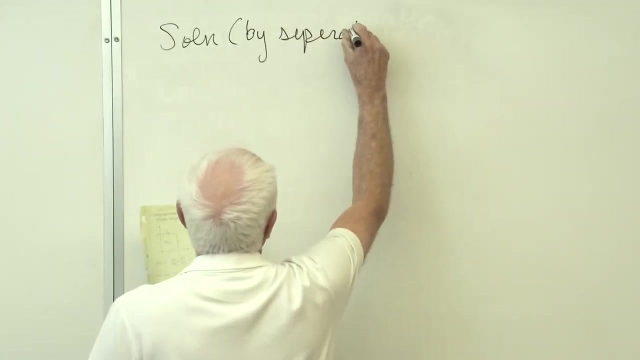 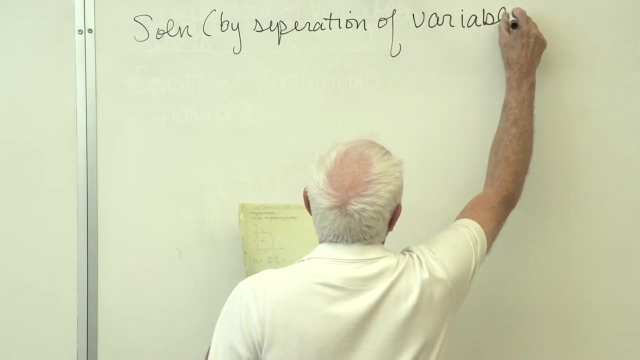 The right-hand side, X equals L. For any Y value, the temperature is T1.. Okay, There's our four boundary conditions. We then solve that equation with those boundary conditions. Okay, And we end up with this solution: T as a function of X and Y. 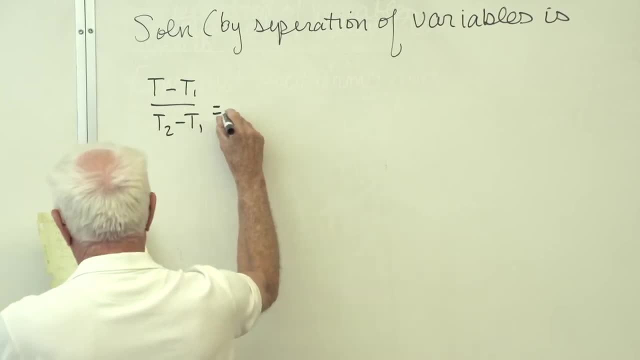 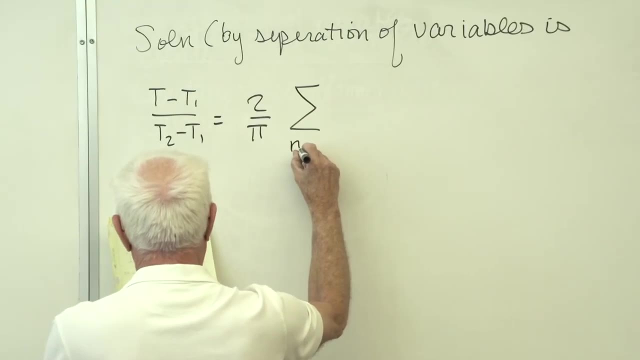 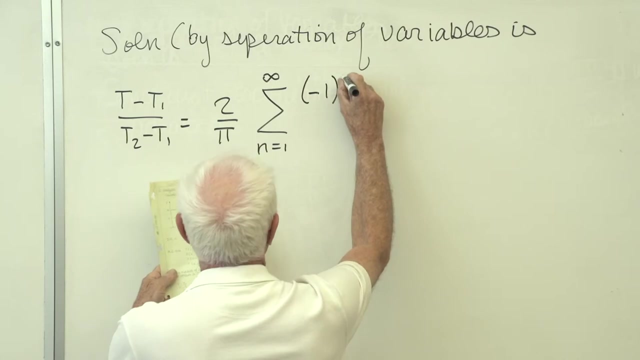 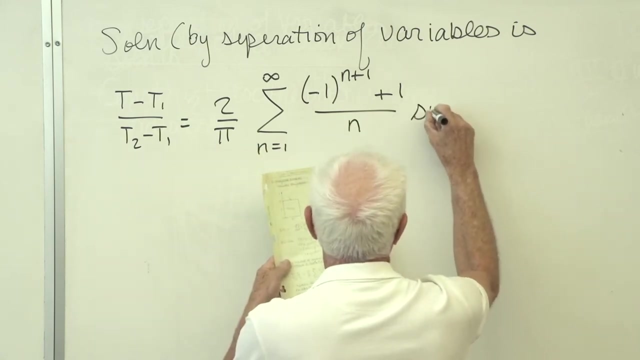 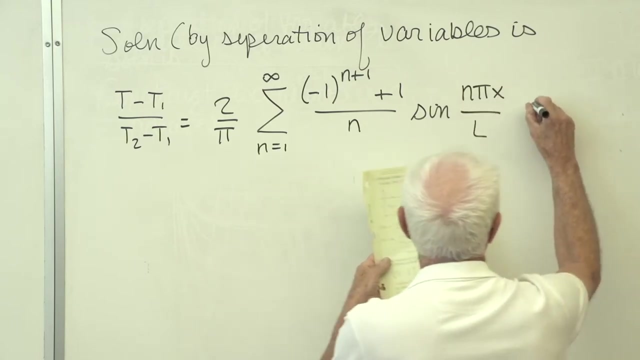 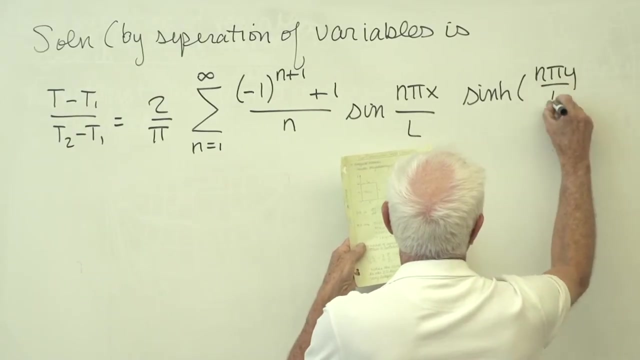 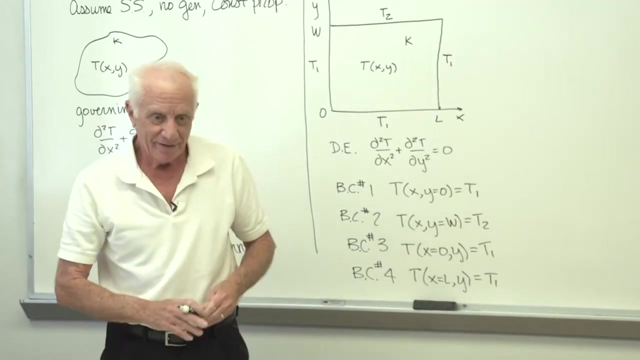 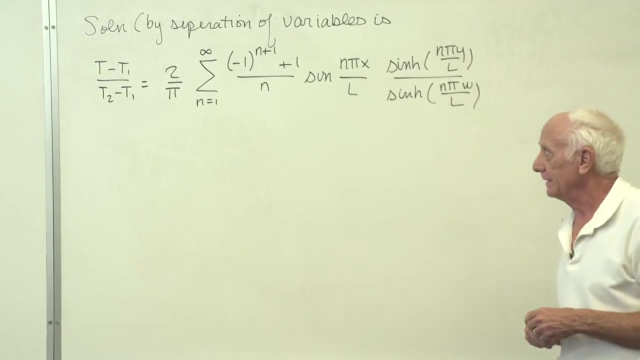 Okay, Okay, It's an infinite solution. How long does it take? I think six days. It's a quick solution. So when we solve that, we get a rather complex looking solution. It's signs, hyperbolic signs, infinite series. 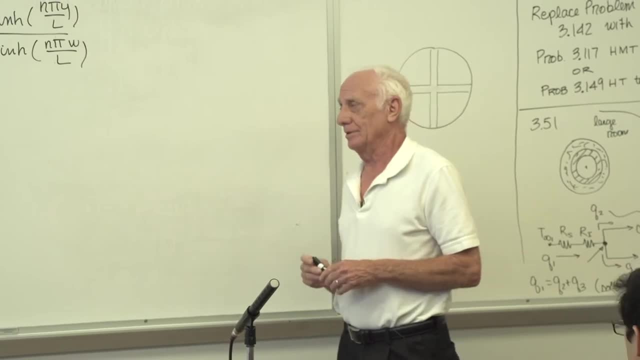 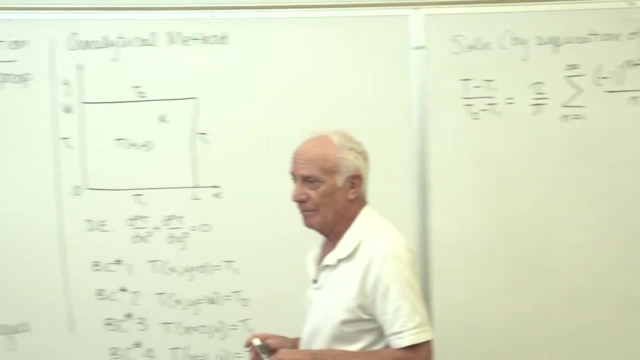 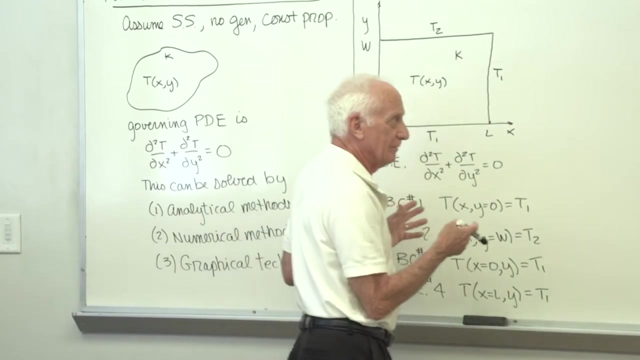 Yeah, it's rather complex looking. What solution is that for? That's for a very simple geometry: a rectangular plate. Nothing in the world is much simpler than a rectangular or a square plate. So for a simple geometry, we get a very, rather complex solution. 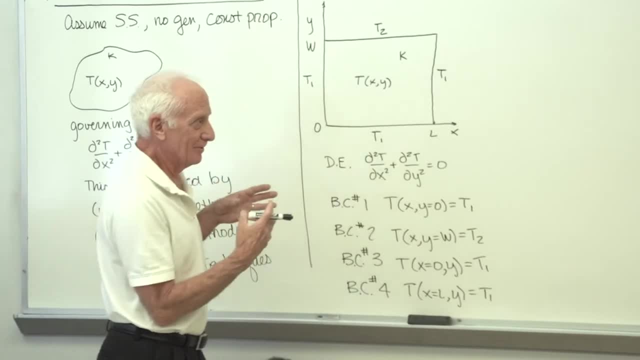 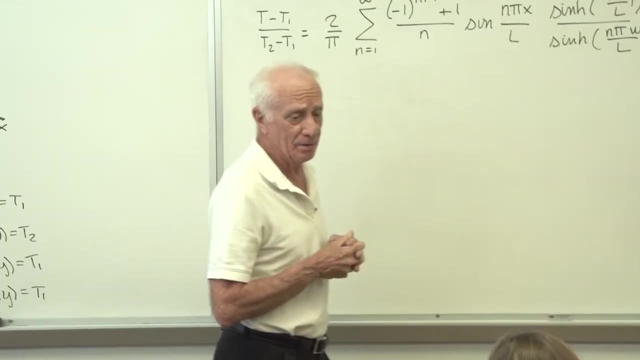 You can imagine, for a non-simple geometry, trying to find the exact analytical solution. Yeah, you do that, but not in this course. You take the graduate course in conduction here at Cal Poly and, yeah, you'll do some exact solutions. 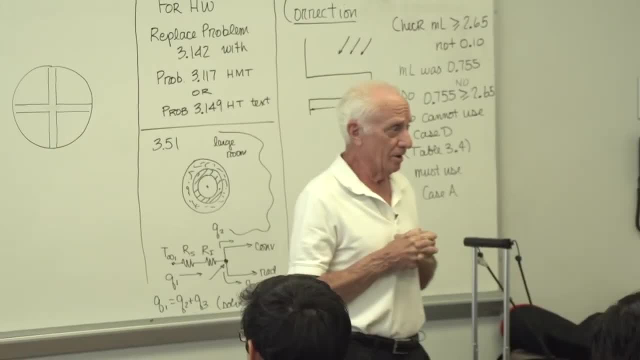 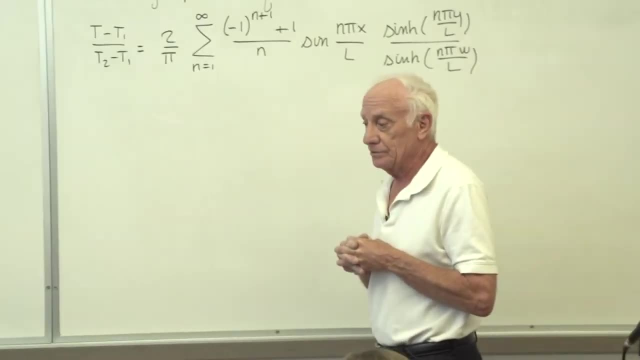 You'll go through all the blood, sweat and tears. Oh yeah, they'll make you work because they want you to see how difficult matters are and you get the exact analytical solution In this introduction class. no, we won't do that. 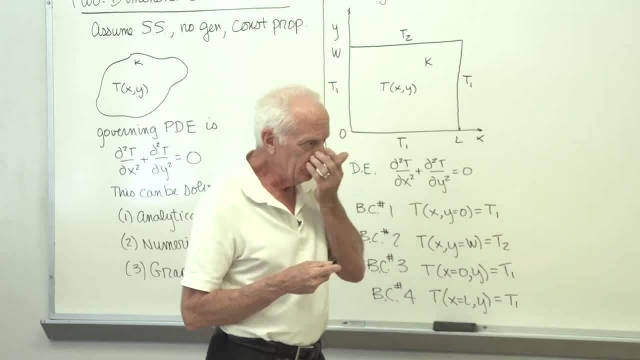 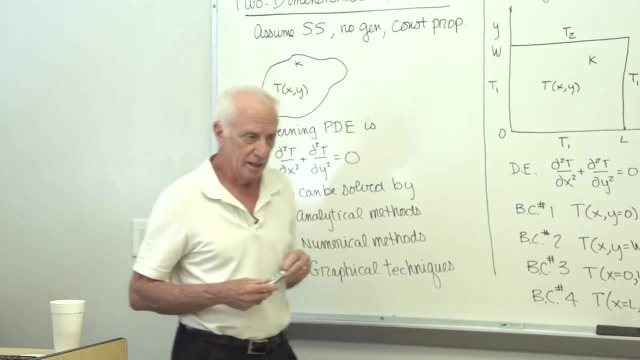 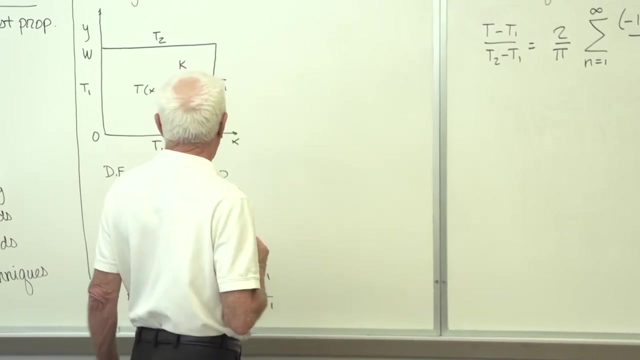 This was just an example of how complex things can get, So we'll pretty much do the second to what we'll do graphical today and we'll do numerical on Friday. So we're not going to use this. What we're going to do now is we're. 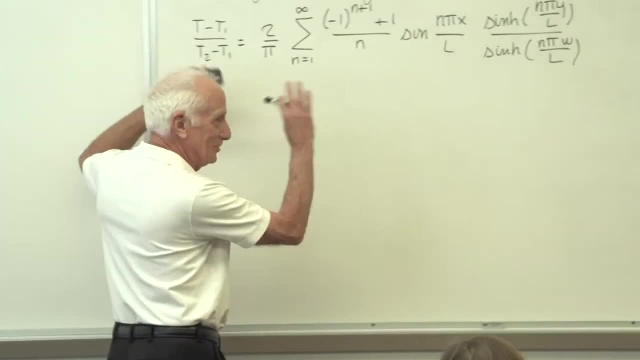 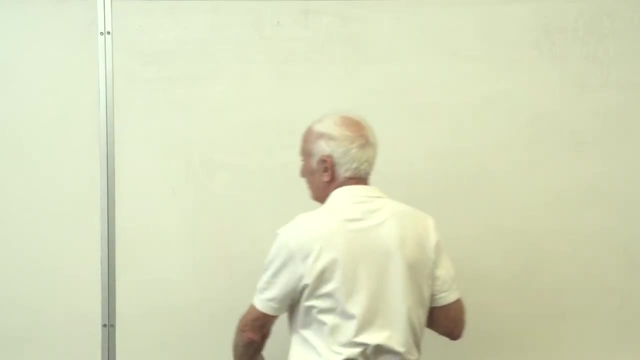 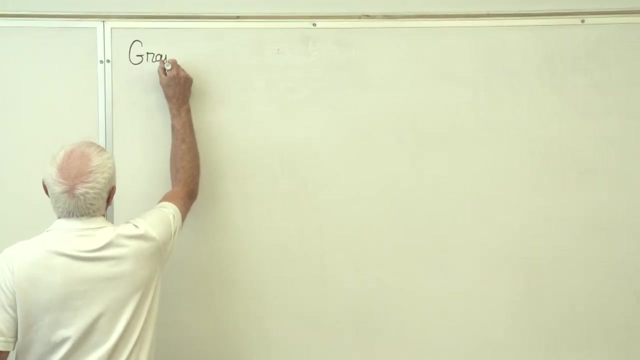 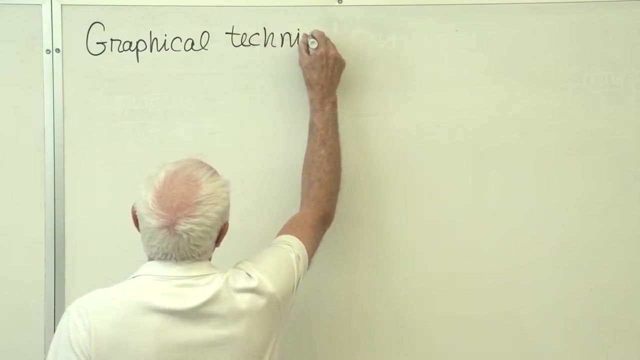 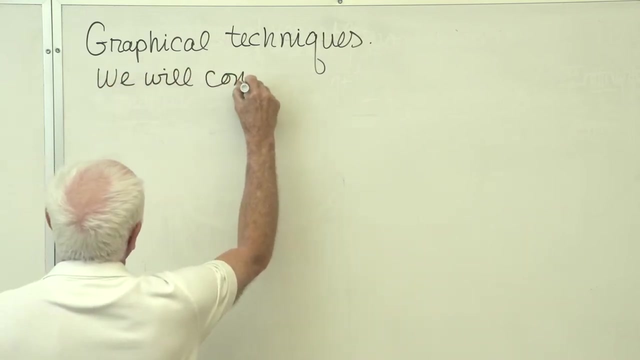 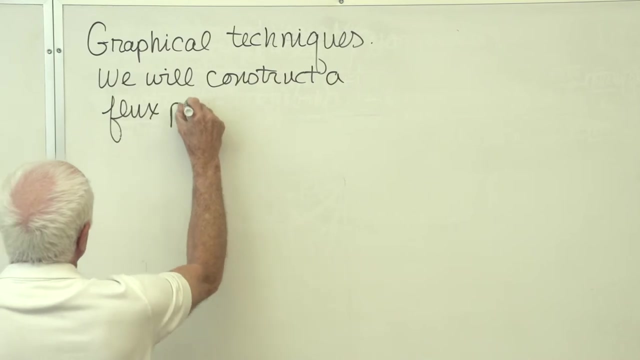 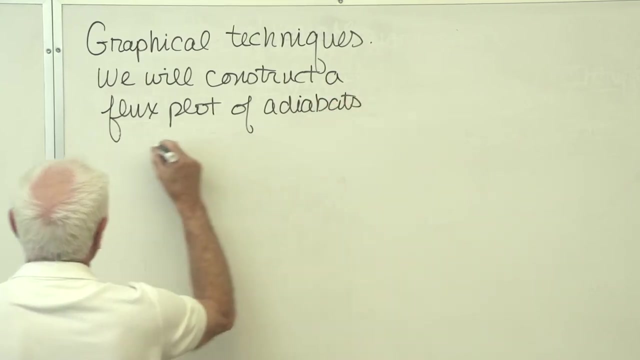 going to do the graphical technique. I need board space and this is not going to be used anymore, So we'll get rid of this. So we'll do graphical first and then, Friday, do numerical. Okay, so I'm going to pass this out to you. 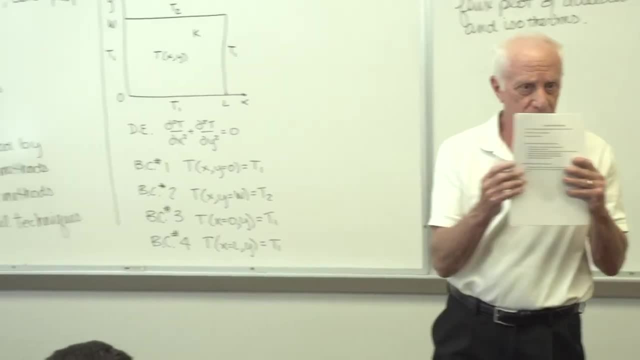 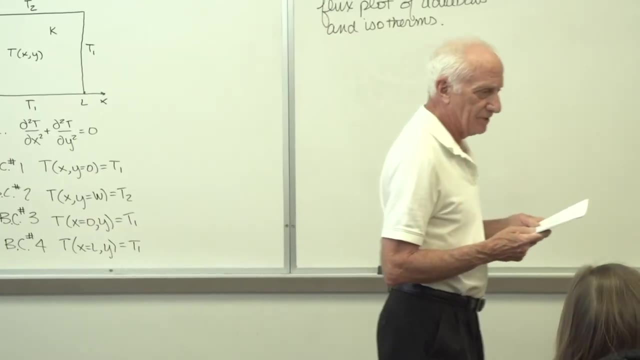 Okay, so anyway, top of the page, a text page, It says a flux plot is a graphical presentation of the isotherms and adiabats for a solid geometry. Okay, that's what I put on the board here. 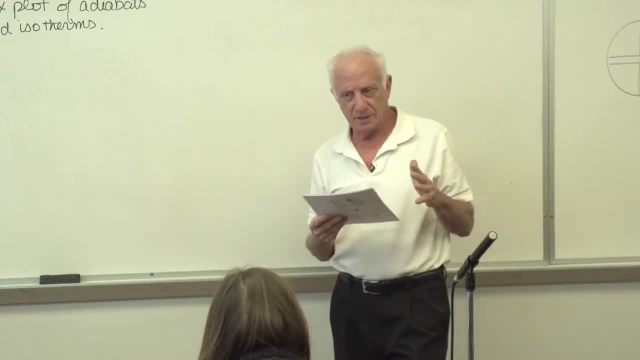 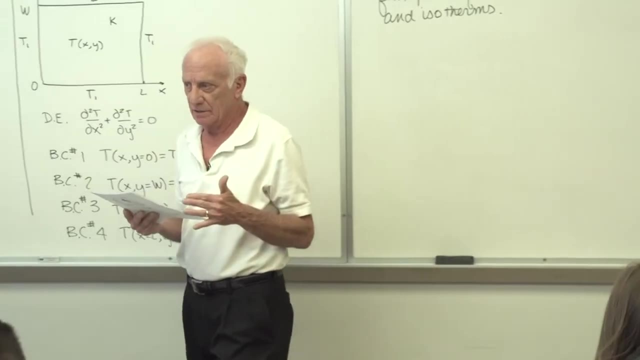 What is an isotherm? An isotherm is a constant temperature line. What is an adiabat? An adiabat is a heat flow line. So you're constructing a diagram of constant temperature lines and heat flow lines. 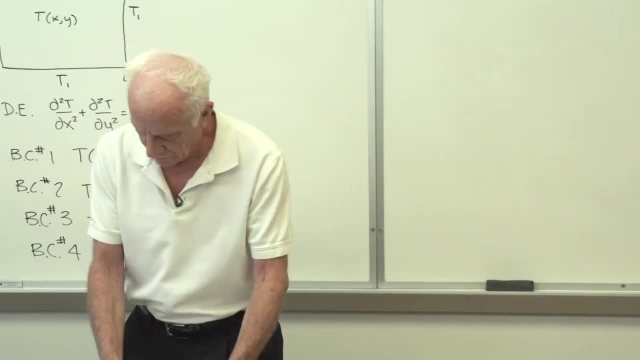 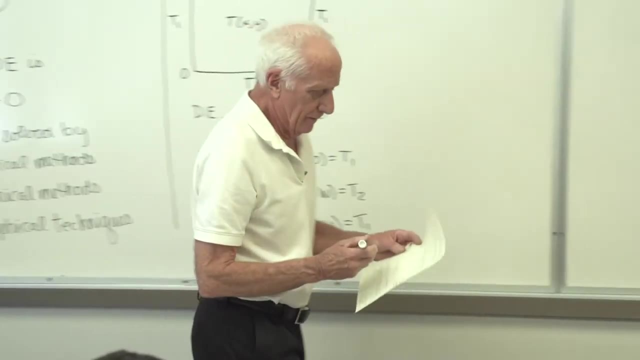 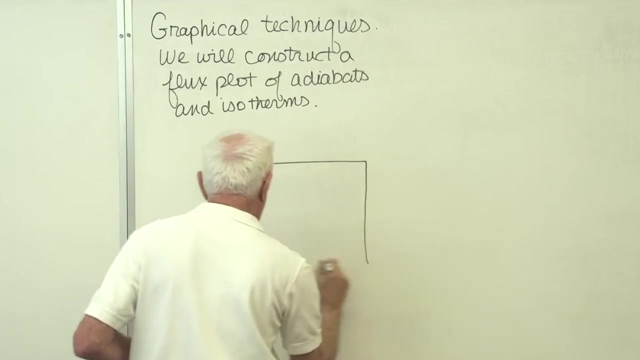 Then there's some basic rules given there. So let me go ahead and draw an example here. I'm going to take a rectangular plate and I'm going to assume the top surface is maintained at a constant temperature- T1,- the left-hand side T2,. 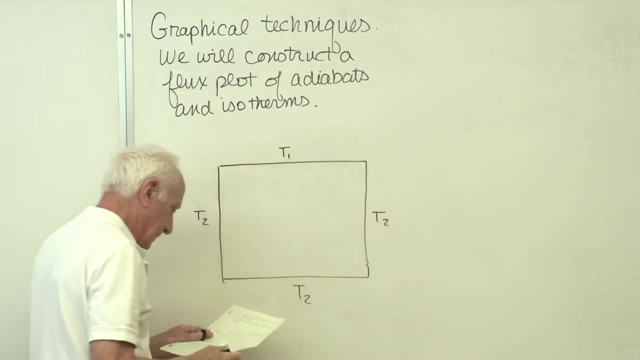 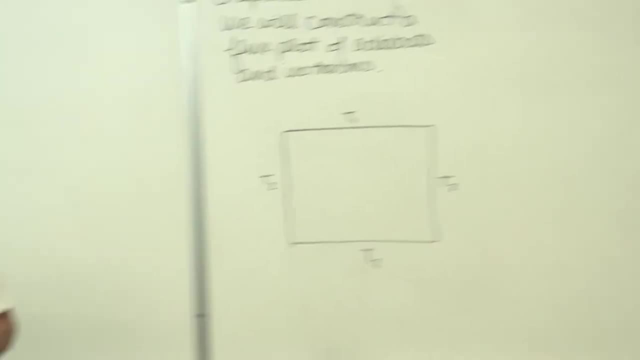 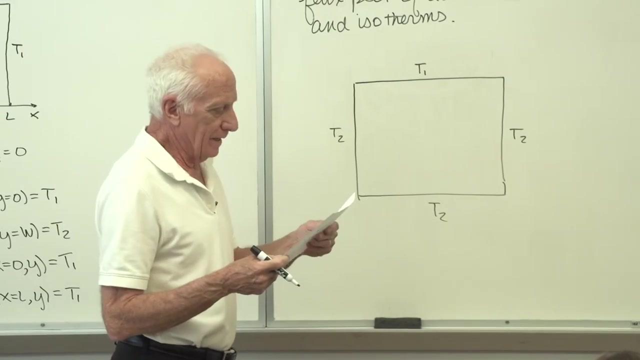 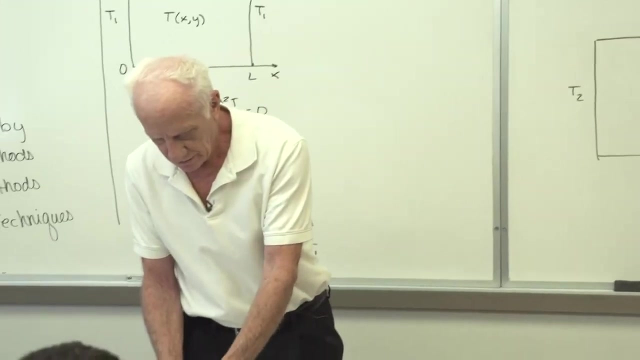 the right-hand side, T2, the bottom at temperature, T2.. I'm asked to construct a flux plot for that. Okay, so here's rule number 1.. Identify lines of symmetry: geometrical and thermal. Lines of symmetry, geometric and thermal. 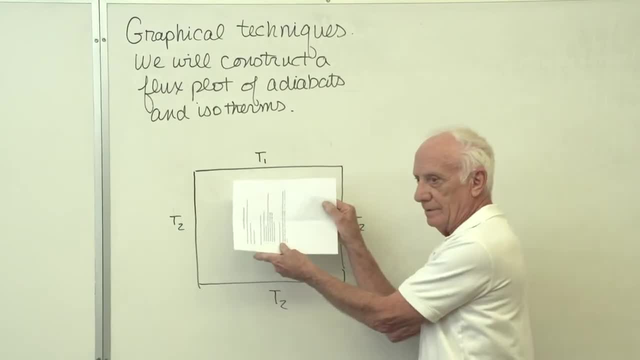 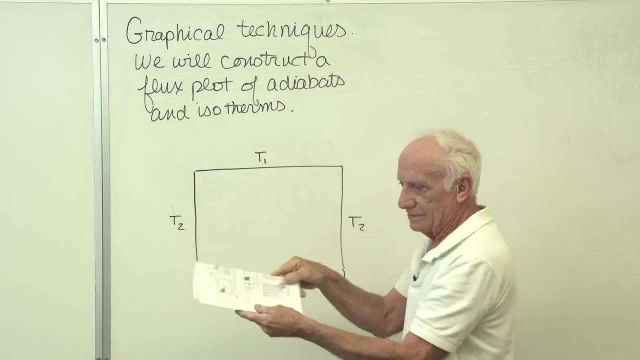 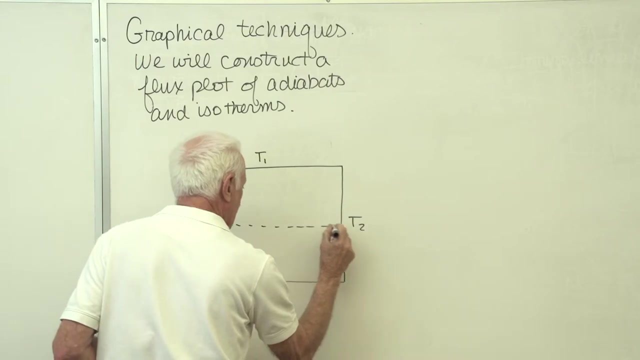 Let's do the geometric. Here's a plate. This is a plate like that plate over there. Here's a plate. If I fold it this way is geometrically symmetrical. So I know one possible line goes through the middle like this: 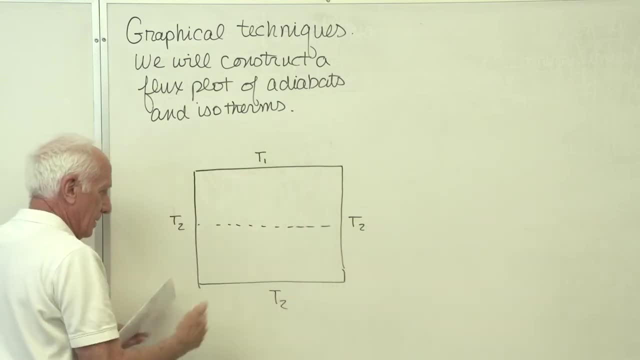 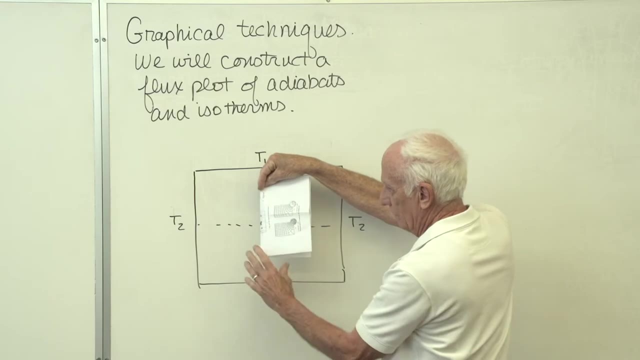 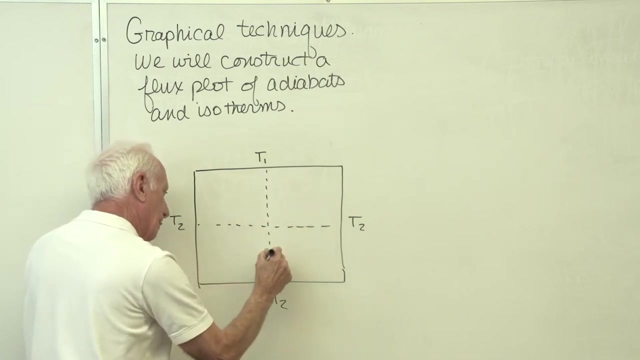 That's geometrically symmetrical. I know that I can take this and fold it about the side, left to right. That middle line is a line of geometric symmetry, Okay, So now I'm going to do this. Don't try and fold it corner to corner. 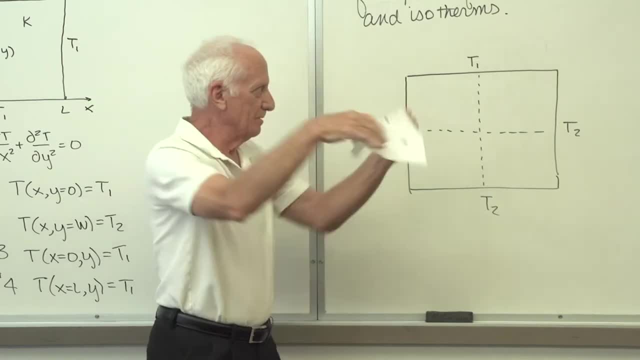 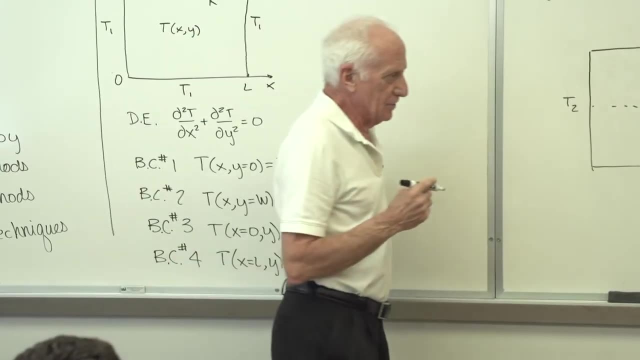 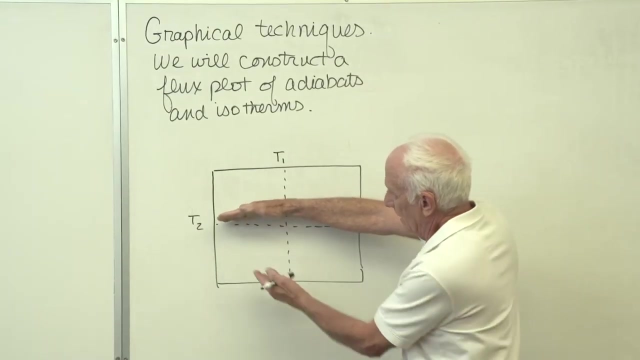 No, that doesn't work, Not symmetrical corner to corner. There they are the only two. Now find the lines which have thermal symmetry. Okay, Take him, fold him about top to bottom. T2 down here, T2 up here. check. 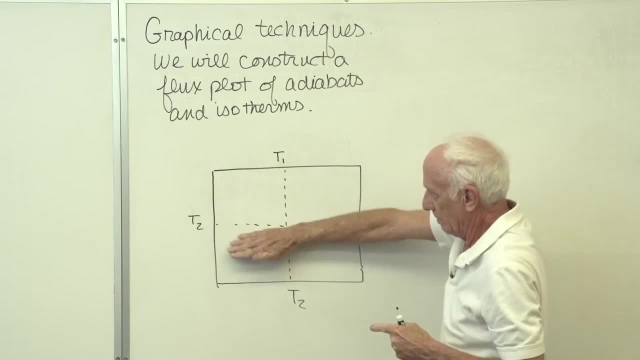 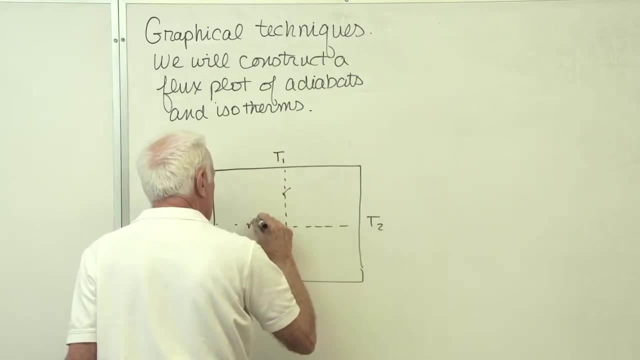 T2 over here, T2 over here. check, And I fold it: T2 at the bottom, T1 at the top. nope, This is geometric symmetry. This is a no-go. It's not thermally symmetrical. 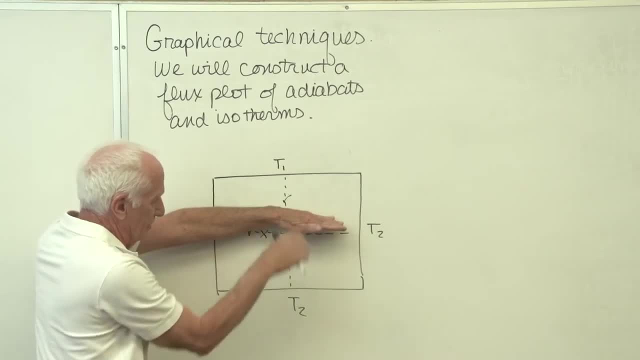 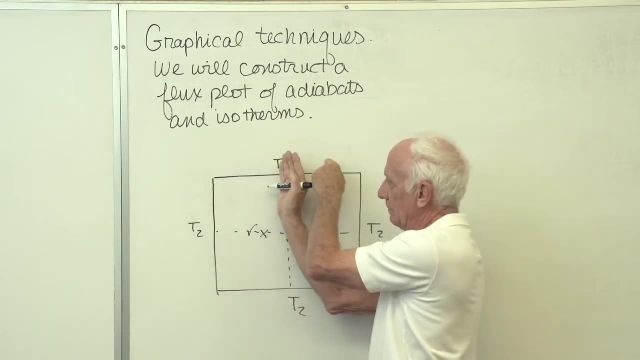 Fold about here. This side comes up to the top. T2, T1,. no, it won't be it. Take this guy here. T2, T2, check. T1, T1, check. T2, T2, check. 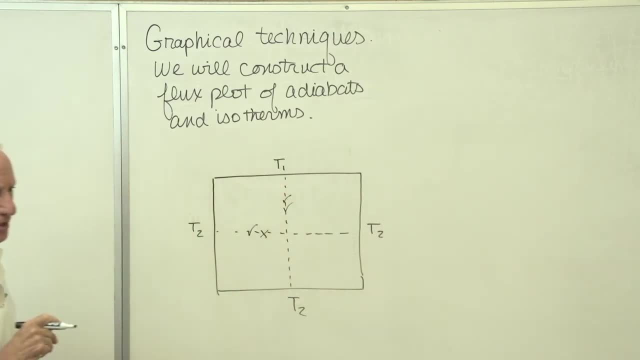 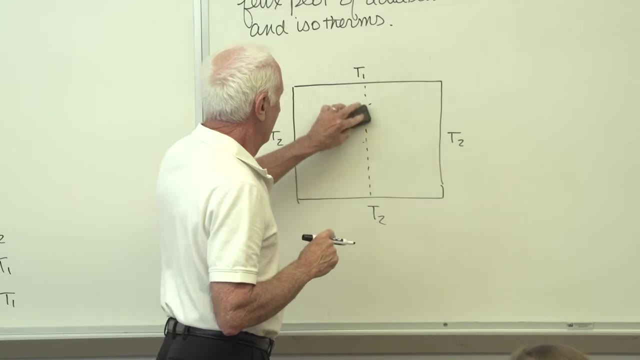 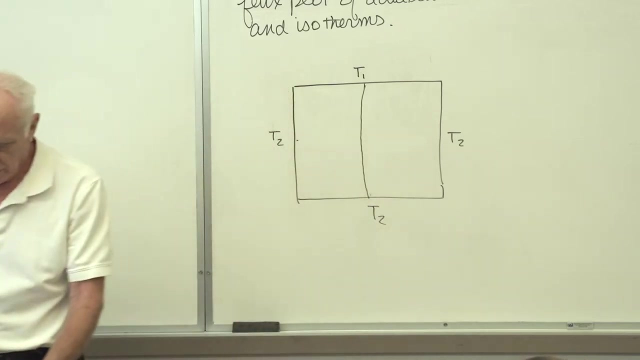 Yep, This guy is a line of both geometric and thermal symmetry, So get rid of him. He's a no-go. He qualifies, So rule number 2. If you found lines of both geometric and thermally symmetrical, 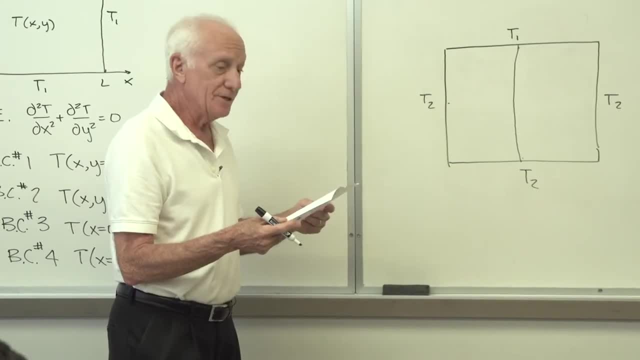 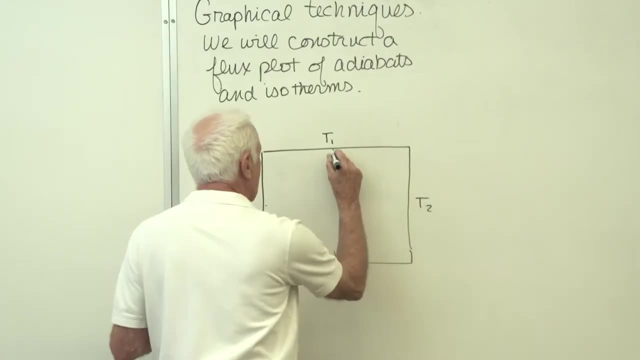 about the part: these are adiabats. Okay, We've found our first adiabat. What's an adiabat? An adiabat is a heat flow line. Does that make common sense? Of course it does. 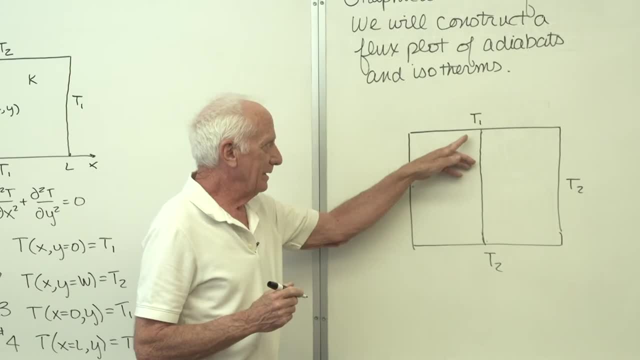 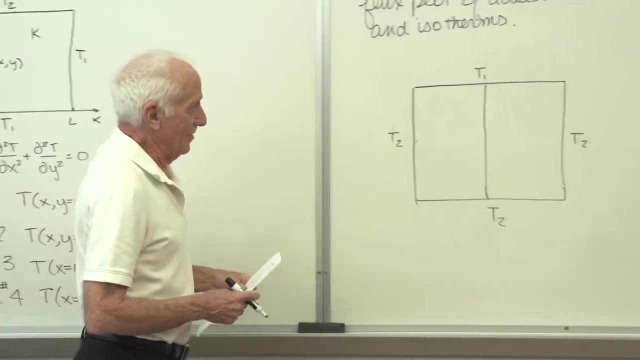 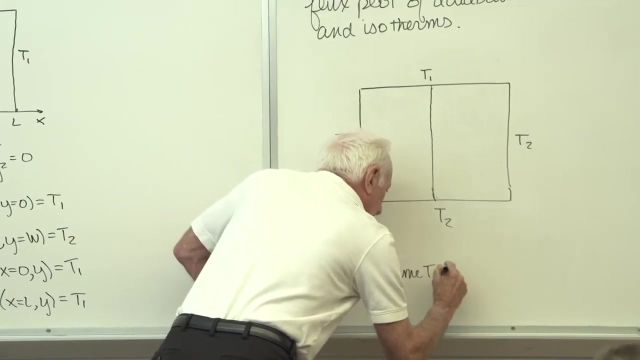 I know. if T1 is hot and T2 is cold, heat in the middle heat's going to go straight down to the bottom. That makes sense to me. All right Now I'm going to assume that T1 is greater than T2.. 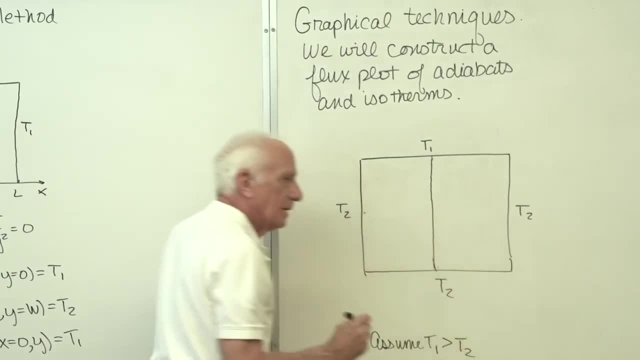 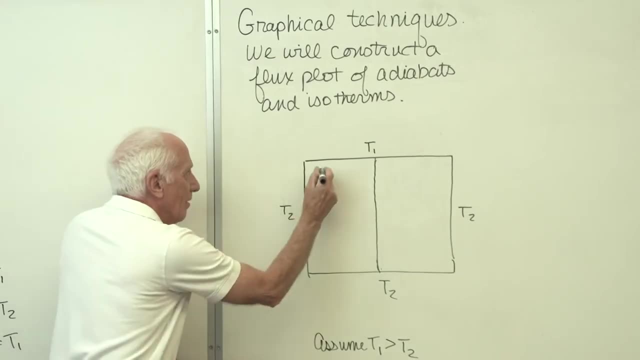 T1 greater than T2.. So in this corner over here upper left-hand corner, if T1 is hot and T2 is cold, I think it's going to go right around that corner. Now don't do this. No, that's wrong. 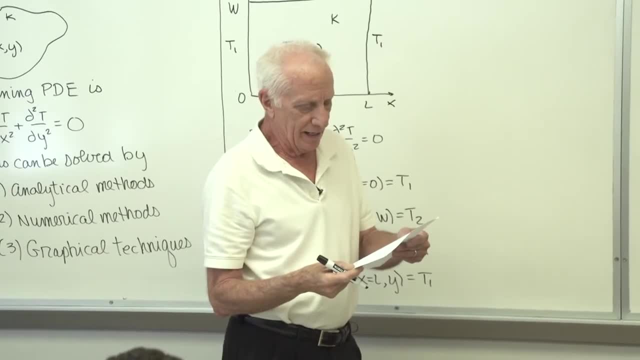 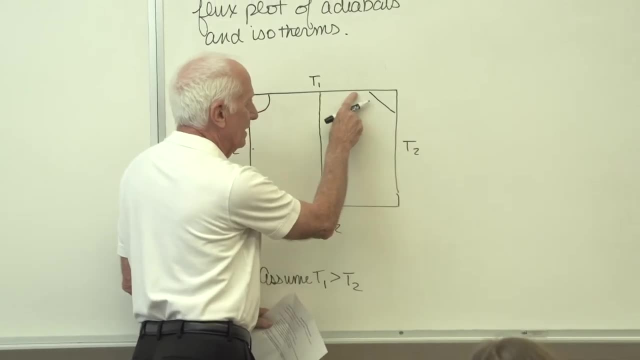 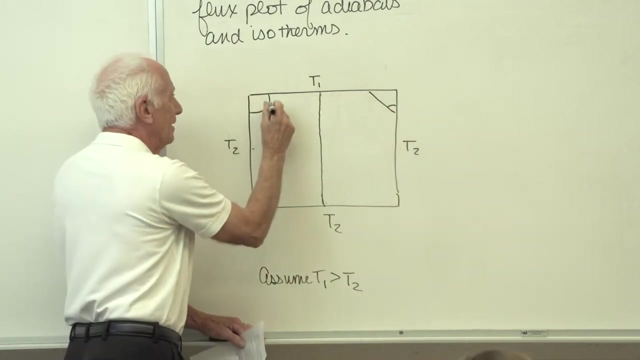 Rule 4. Adiabats intersect isothermal boundaries at right angles. That's an adiabat, That's an isotherm. That's an isotherm boundary. That's not a right angle. No, it doesn't go in like that. 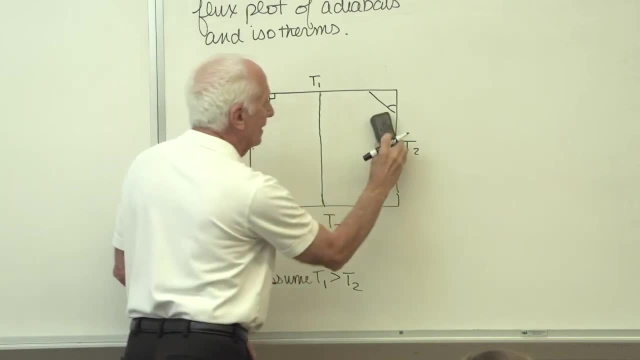 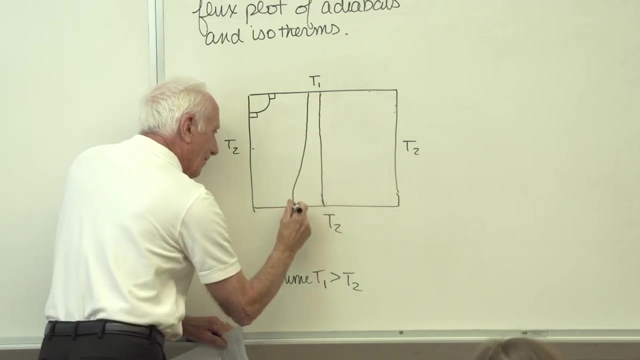 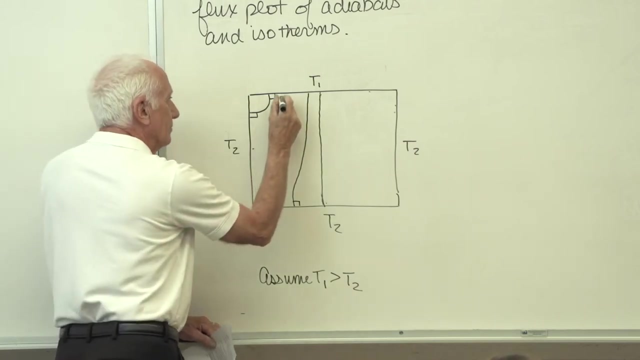 It goes in like that around the corner. Get rid of that line like that. Now fill in the rest. Okay, Comes out. Right angle. Every time an adiabat intersects an isothermal boundary, it does so at right angles. 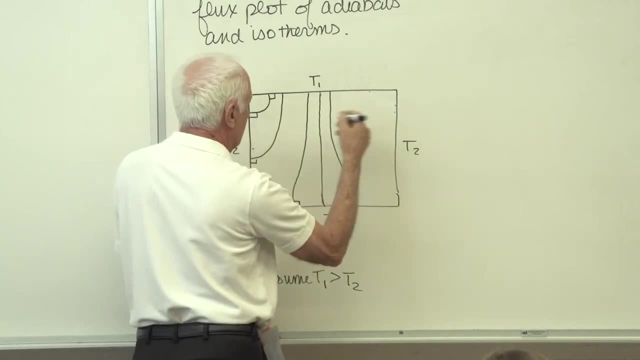 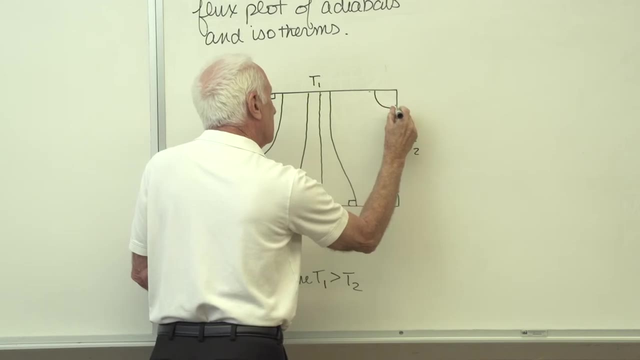 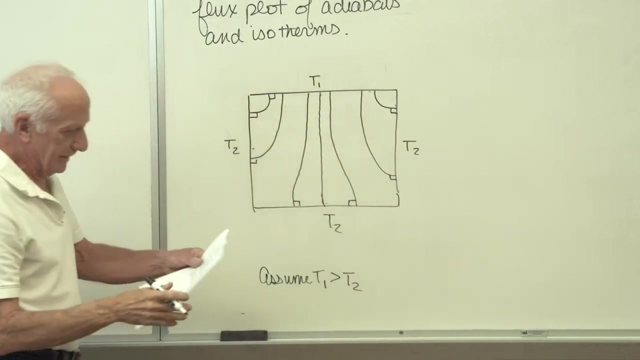 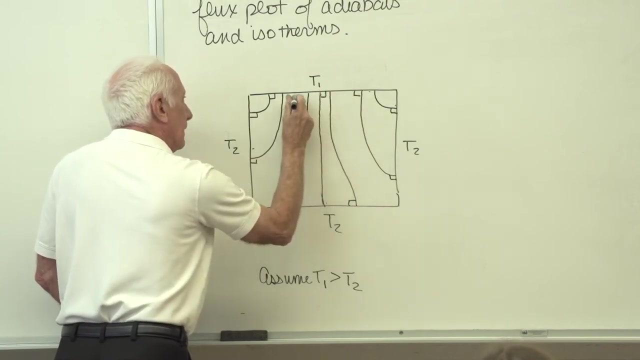 Because it's symmetrical. you wouldn't have to draw both sides, but I normally do, because it gives me a complete feel for the problem, but you wouldn't have to. Now I come out here and now I start going down that way. 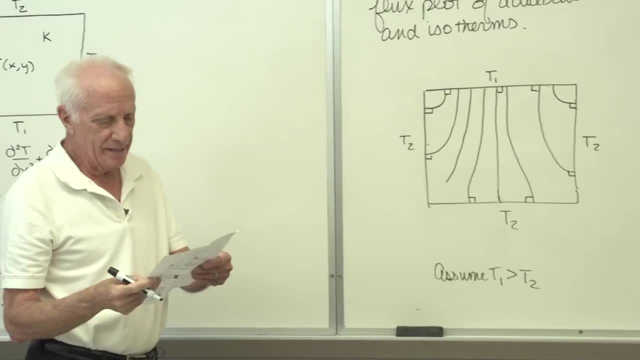 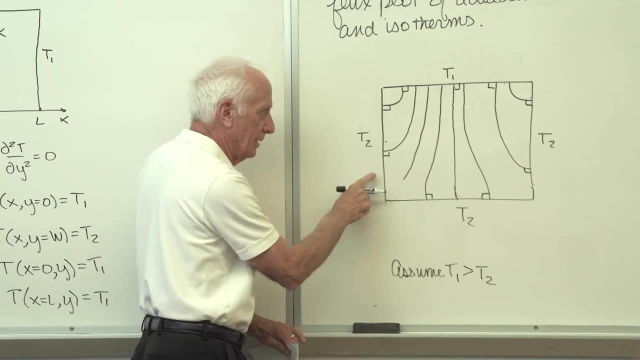 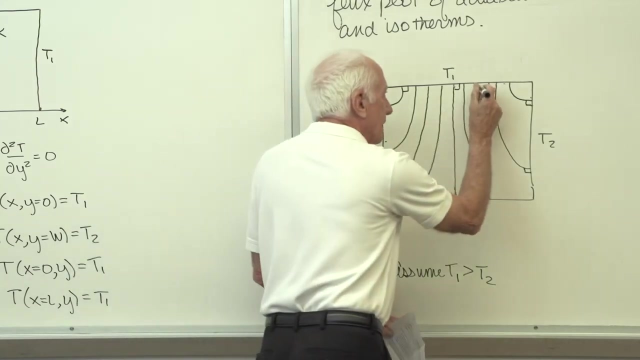 Rule number 6.. An adiabat bisects an isothermal corner. This is an isothermal corner T2,. T2 bisects Comes in 45 degrees equal angles. There it is. This guy comes down here. 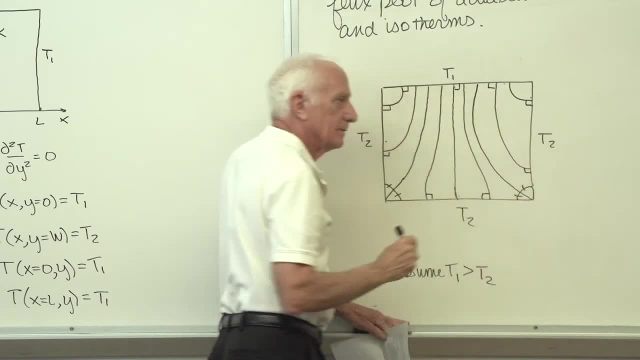 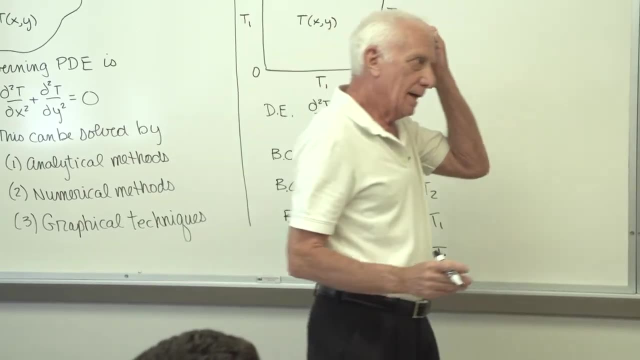 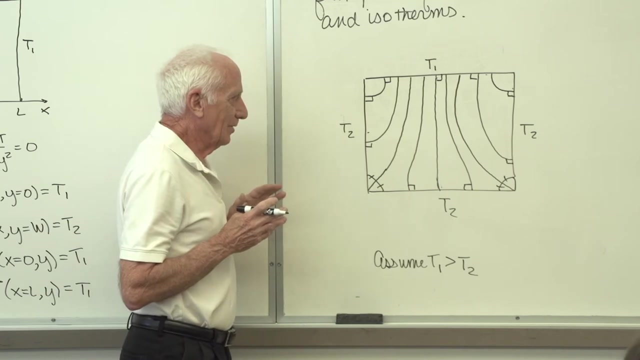 goes into that corner, isothermal corner, bisects it. There's my heat flow lines called adiabats. I call that the adiabats. Now I'm going to draw The constant temperature lines. So I know one is the top surface here. 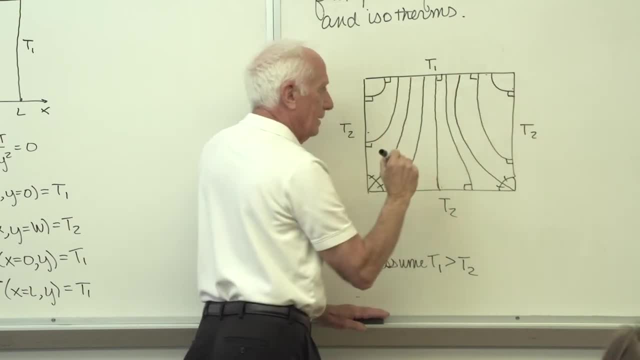 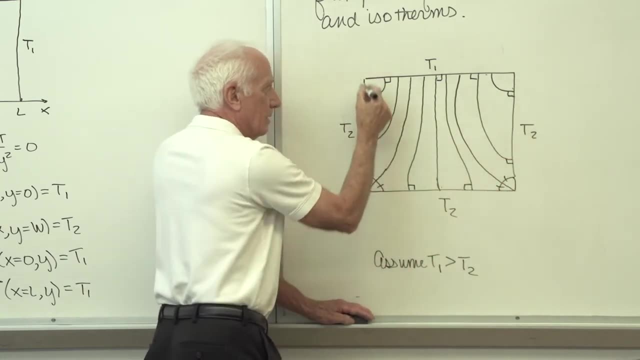 That's T1.. That's an isothermal line. I know the two sides of the bottom T2.. That's an isothermal line. It's U-shaped, The top's horizontal. So now I draw the constant temperature lines coming out. 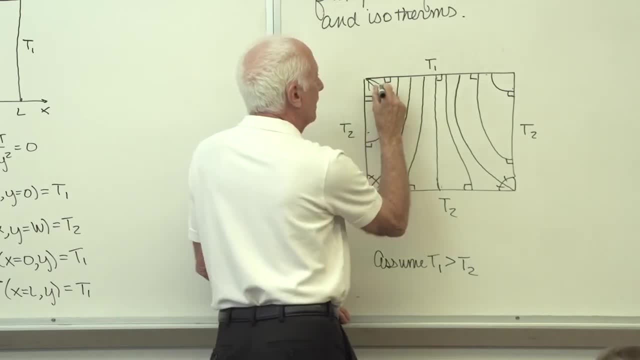 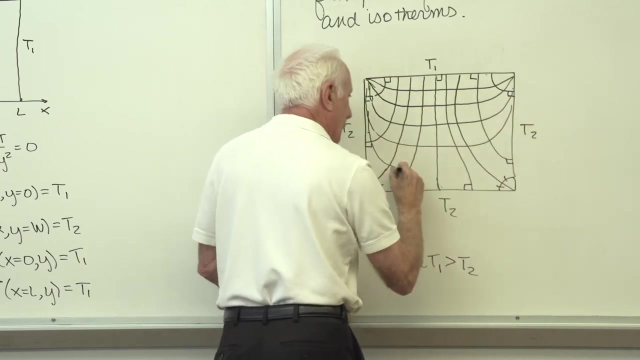 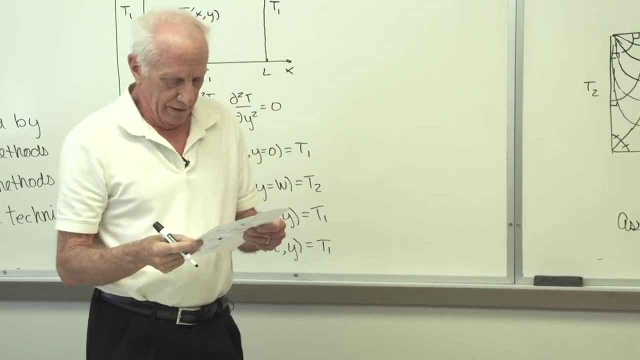 They come out of the corner in a fan pattern. They come out, they cross here, they go up there. They come out, they cross here, they go up there, and so on. Now here's the rule, Rule 3. Inside the solid boundaries. 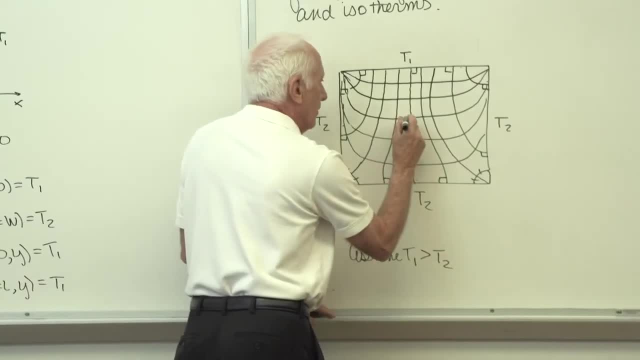 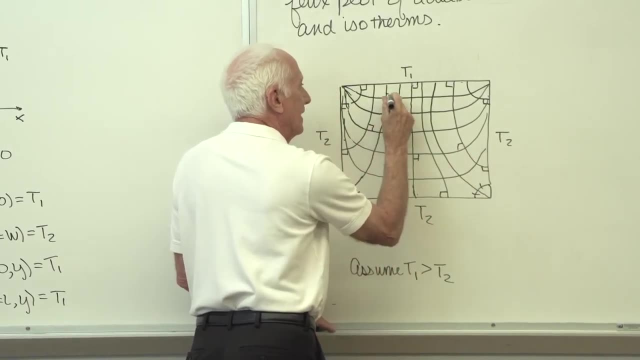 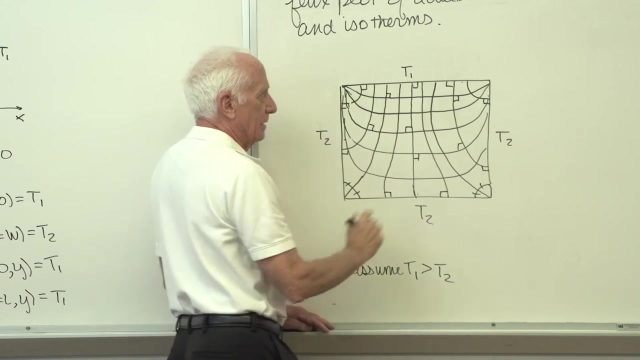 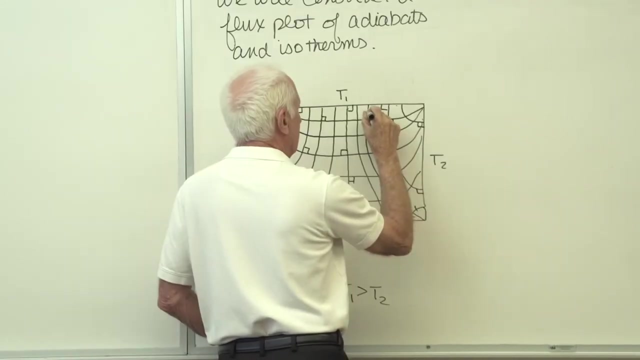 the isotherms and adiabats cross at right angles: Right angle, Right angle, As best you can draw, It's your sketching skills: Right angle, Right angle, Right angle. They fan out from the corner. These guys are the adiabats. 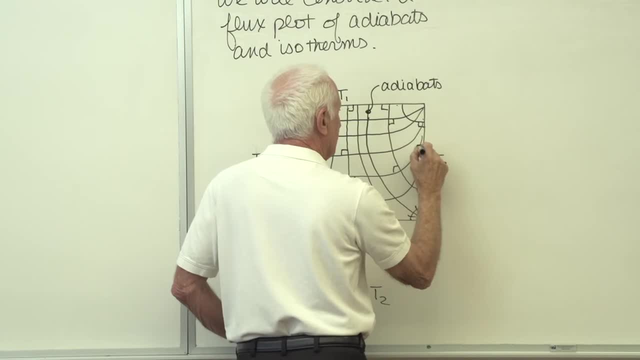 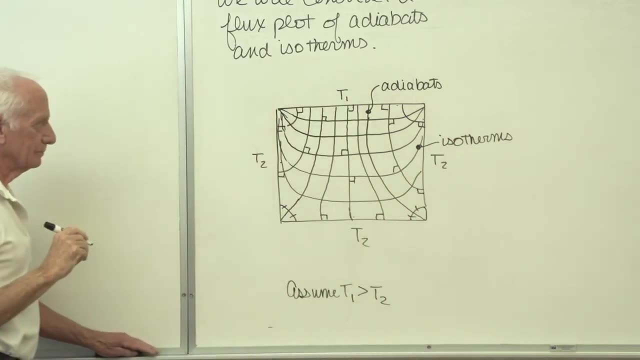 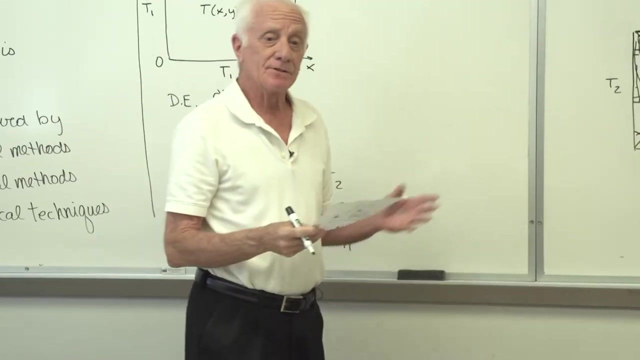 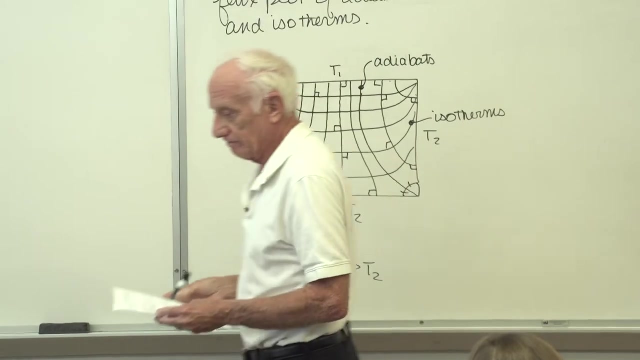 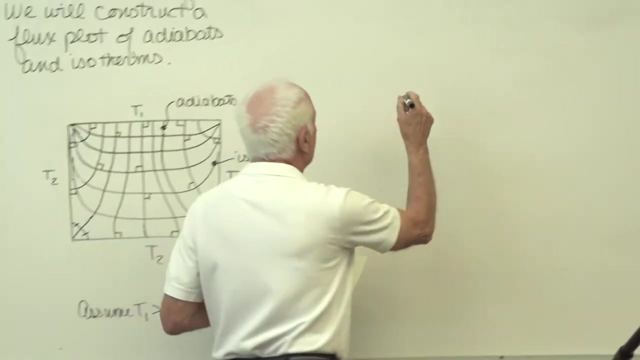 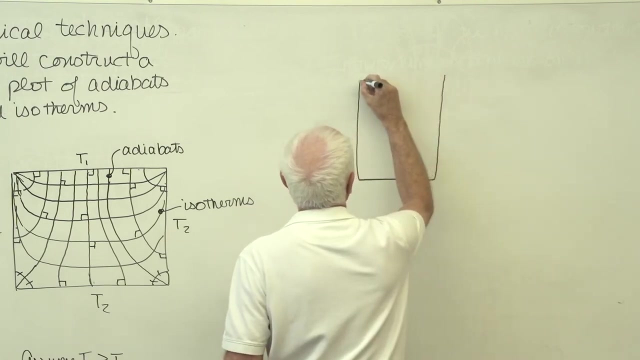 These guys are the isotherms. Okay, That's the flux plot. That's what it's called the flux plot. Now we'll take another one. This one is a rectangular portion, Then there's a semicircle. 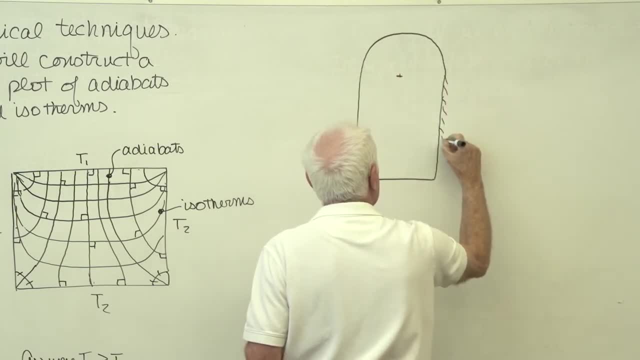 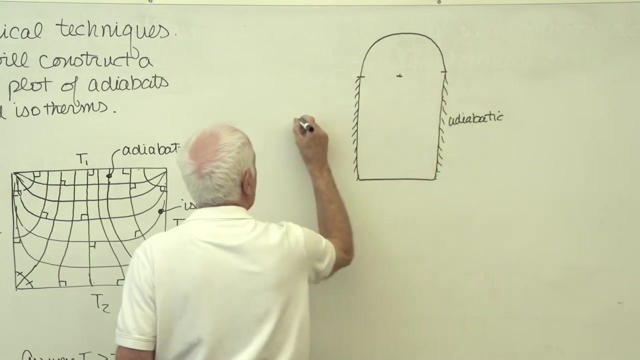 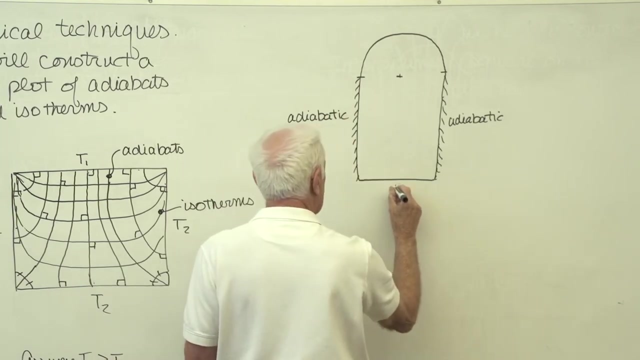 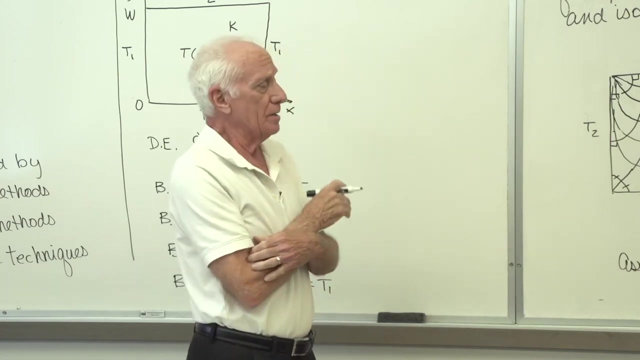 These sides here are adiabatic. This side is also adiabatic. This side's at temperature T2.. This side's at temperature T1.. Draw the flux plot, Rule number 1. Look for lines of both geometric and thermally symmetrical. 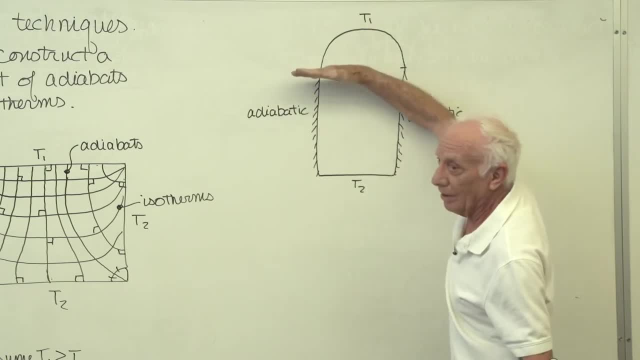 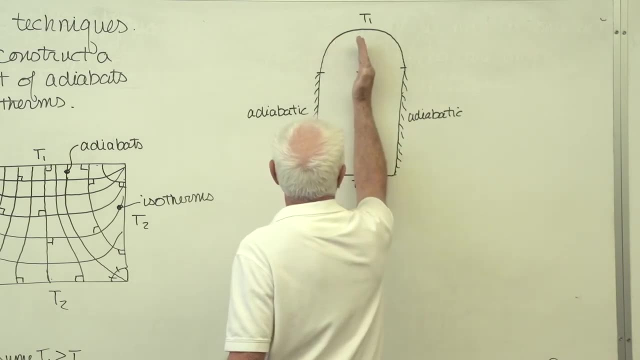 No, no, no, no, No. horizontal line qualifies Vertically. no, no, Yes. right in the middle That's a line of both geometric and thermal symmetry. Right angle, Right angle. That's my first adiabat rule 2.. 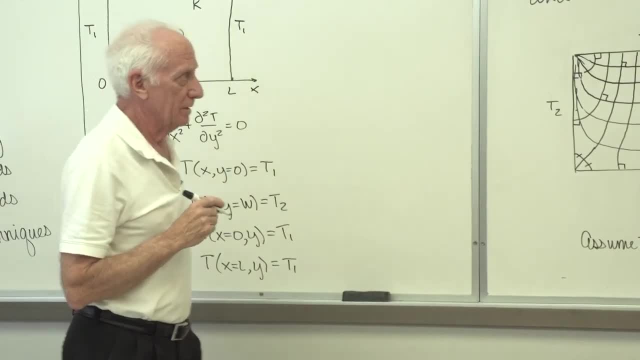 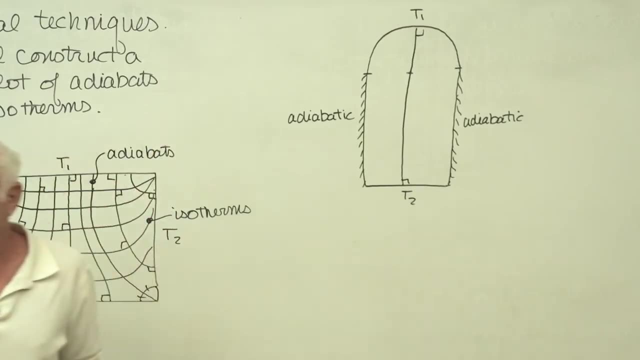 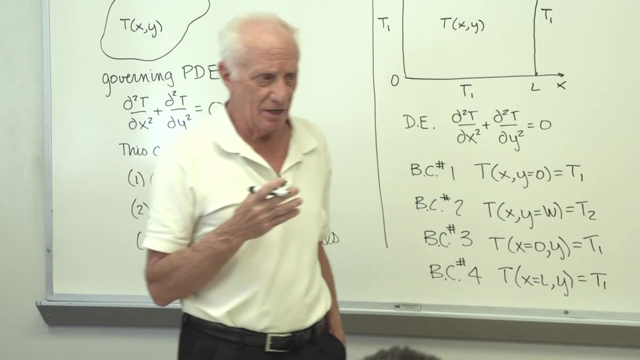 Lines of both geometric and thermal symmetry are adiabats. Now, normally you got a choice. You can draw the isotherms first or the adiabats. That's a choice. Most people have a better intuition about which way heat. 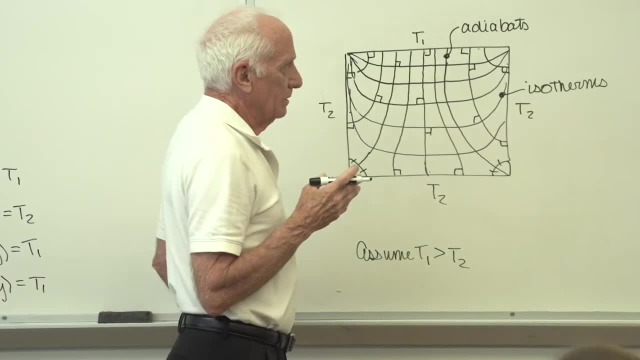 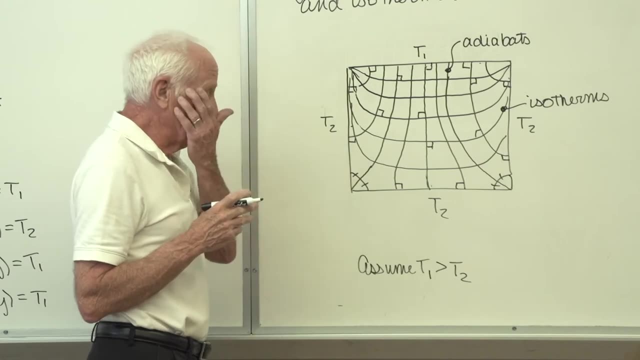 flows than they do the isotherms. So my intuition tells me, if I- oh, let me back up one minute- If I do this problem, the guy says: you know what I made a mistake. I'm sorry about that. 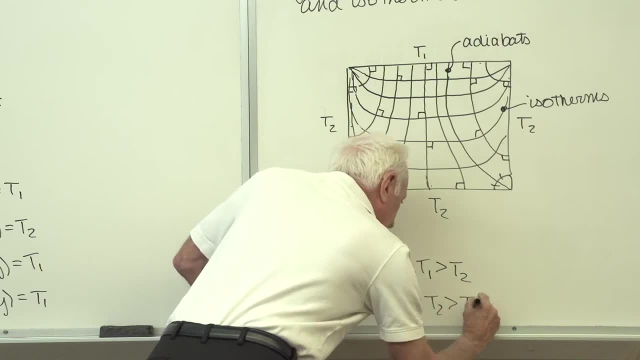 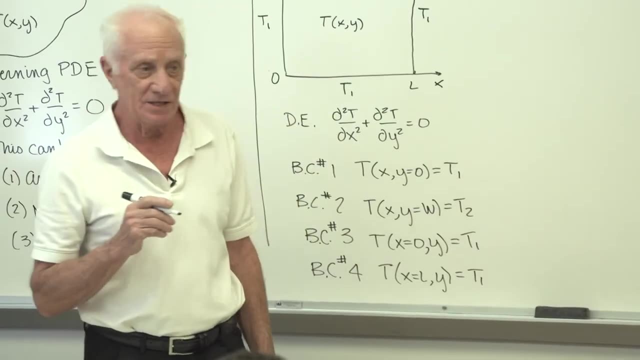 Really, T2 was greater than T1.. I say okay, by the way, there's the same picture. The guy says, oh, they're the same. I say yeah, they're the same, Doesn't matter which is hot and cold. 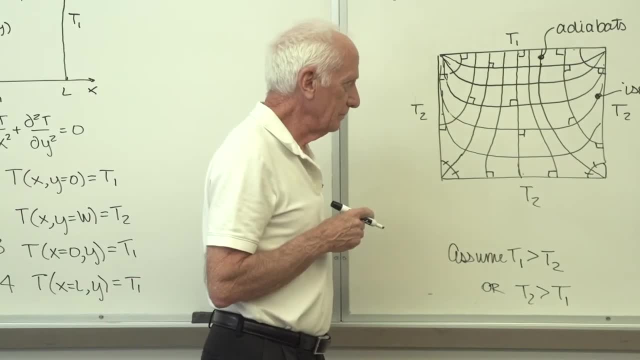 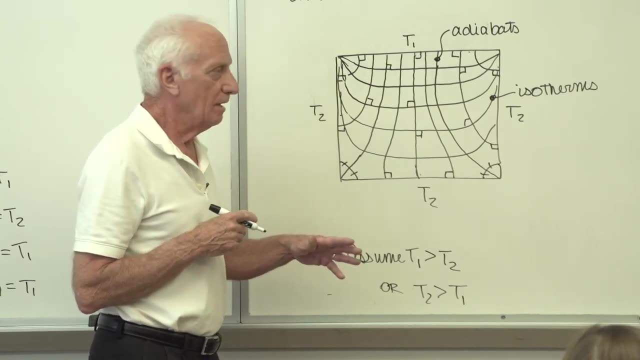 Doesn't matter which is hot and cold. Whatever helps you to visualize it. that's what it amounts to. If you want to say I'm going to pretend T1 is hot and T2 is cold, go ahead and say it over here. 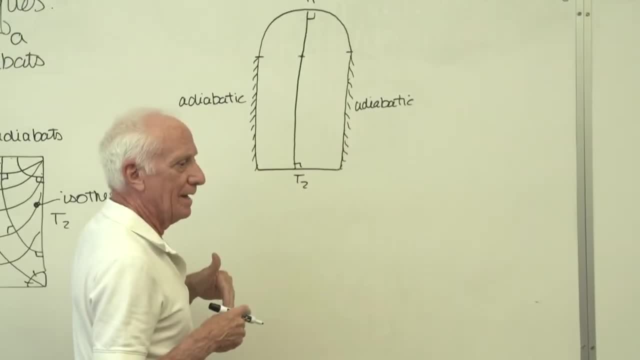 I'm going to pretend T1 is hot and T2 is cold. Good, I got a feel for that. I think heat's going to flow out of here. It can't get out the sides, so it's going to get out the bottom. 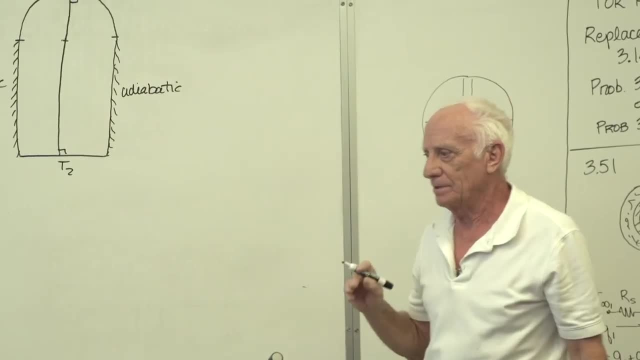 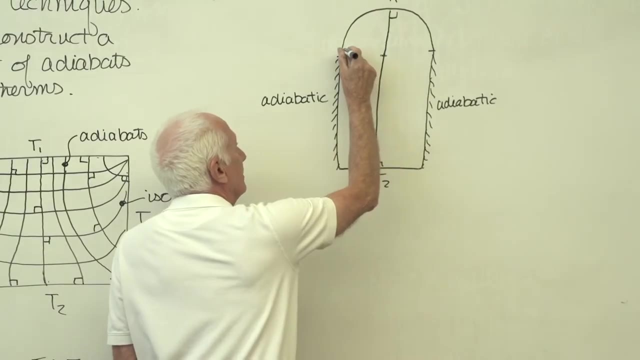 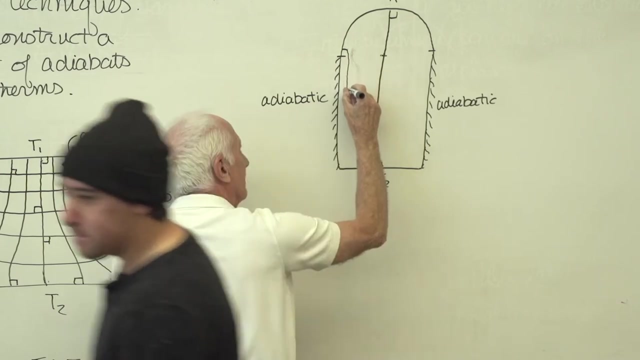 Of course. Which way does heat flow From the top to the bottom? Which way do the adiabats go From the top to the bottom? Let's take one: Makes a sharp right turn and goes out the bottom. Sharp right turn and goes out the bottom. 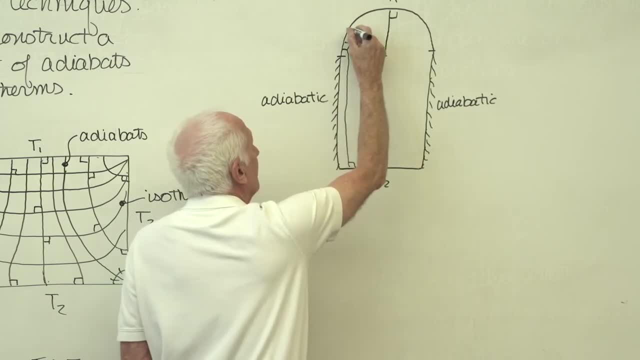 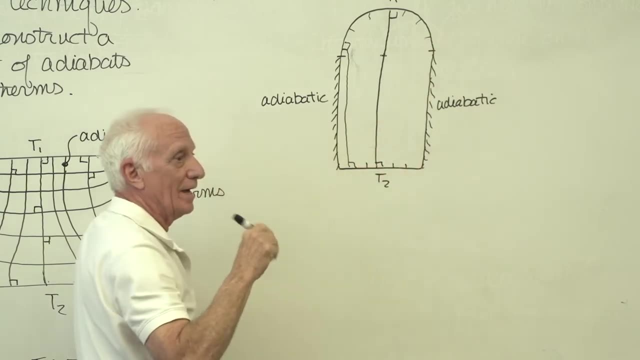 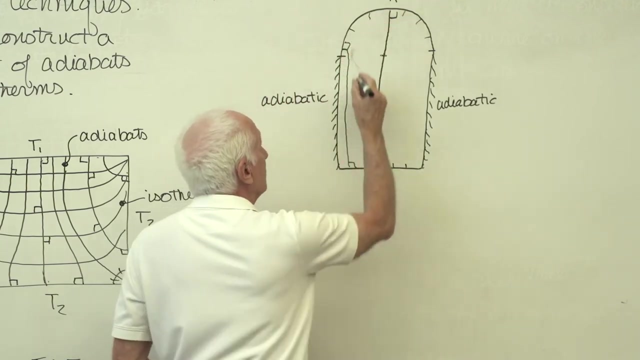 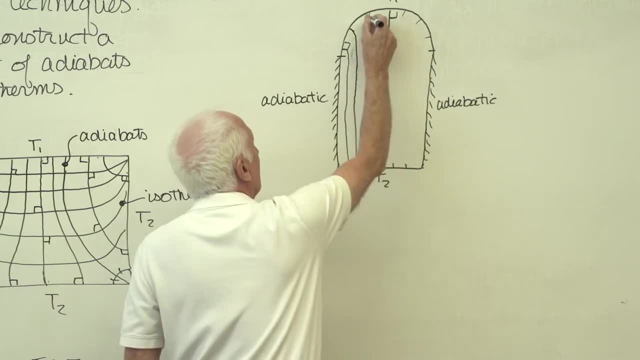 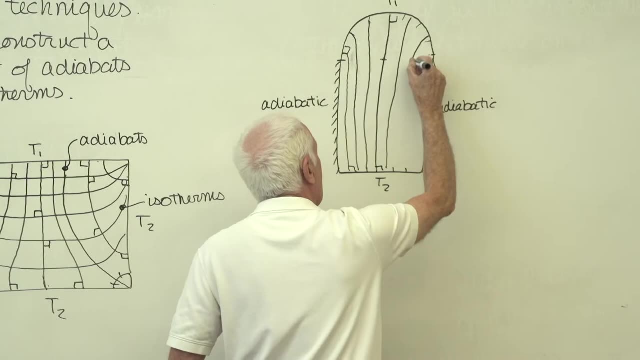 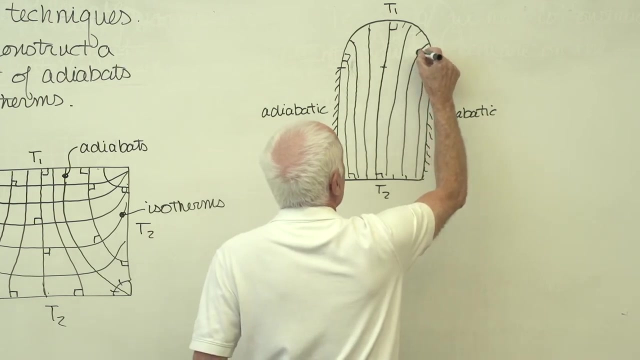 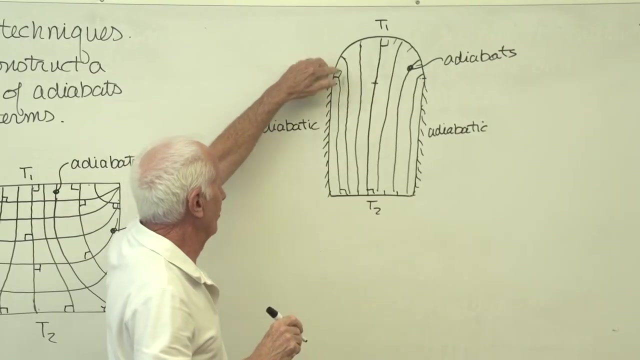 Comes out down here, Comes out down there. Comes out there, Comes out there, Comes out there. Adiabats. They can't get out the sides because of course the sides are adiabatic. So you don't want to draw a heat flow line. 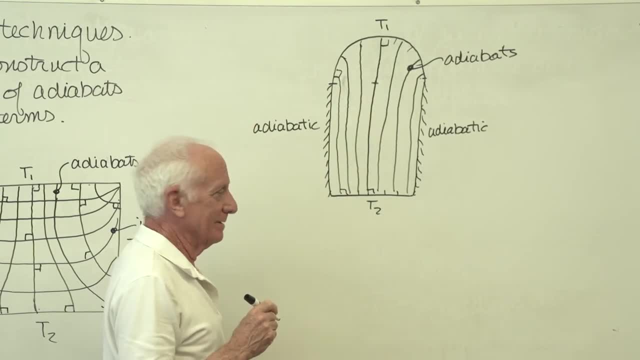 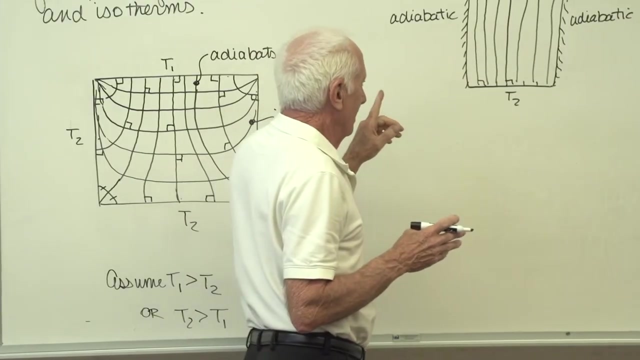 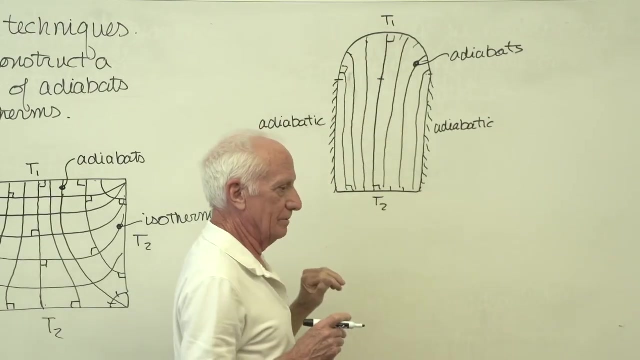 going into the sides cannot happen. Adiabatic sides means no heat gets out there. Once you've drawn that, now you can draw the isotherms. I'm going to pretend that T1 is 100 and T2 is 0.. 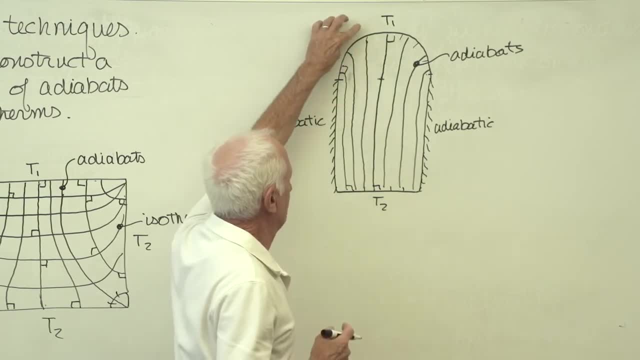 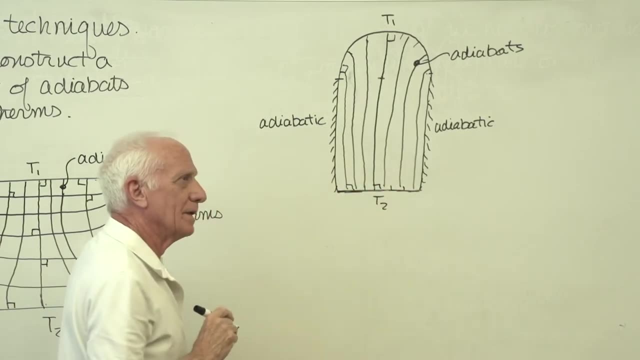 If this helps, you're fine. 100 T1, 0- T2.. Here's the temperature: T2, 0 degrees there. Where do I think the line 10 degrees is going to be? This is a line 0, 10.. 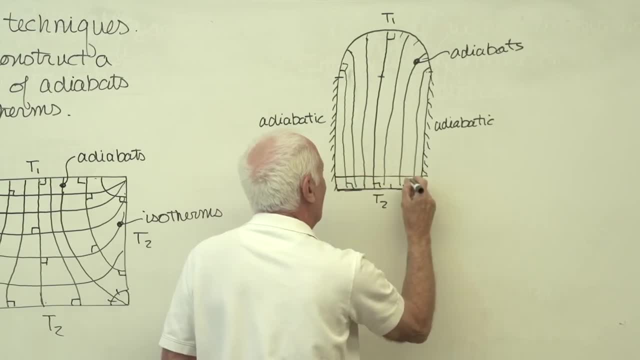 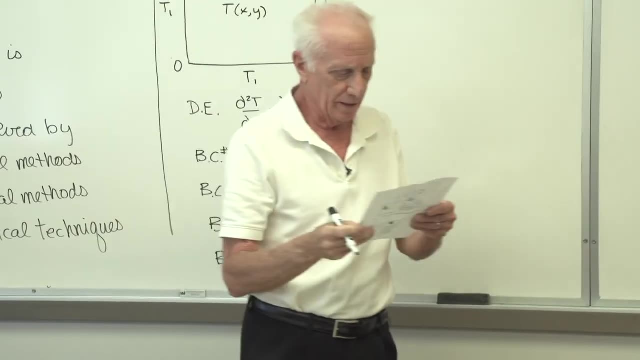 That's 100.. You know what I'm going to say? Yeah, right there, Of course, That's the line 10 degrees. But you better realize. here's the rule. Rule 5, isotherms intersect adiabatic boundaries at right angles. 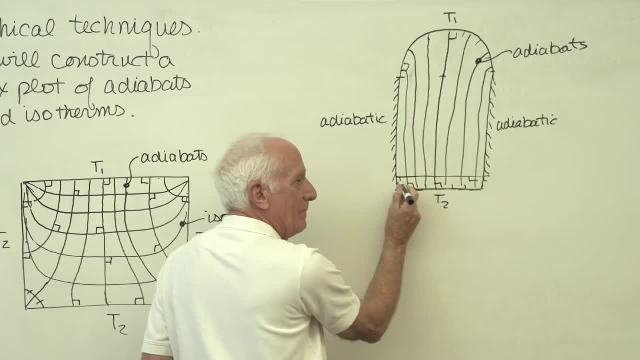 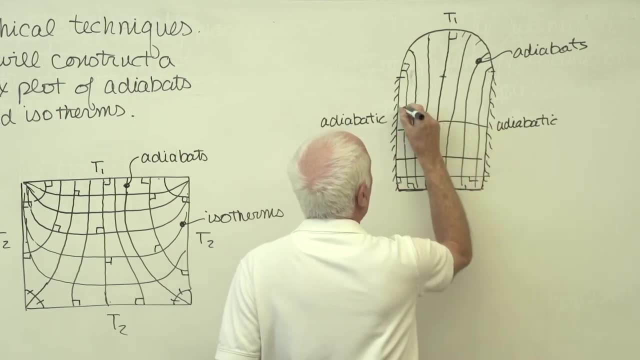 This is an isotherm. It intersects an adiabatic boundary at a right angle. Here's another one, and another one, and another one, and another one. Yeah, everywhere they must intersect at right angles. These guys are the isotherms. 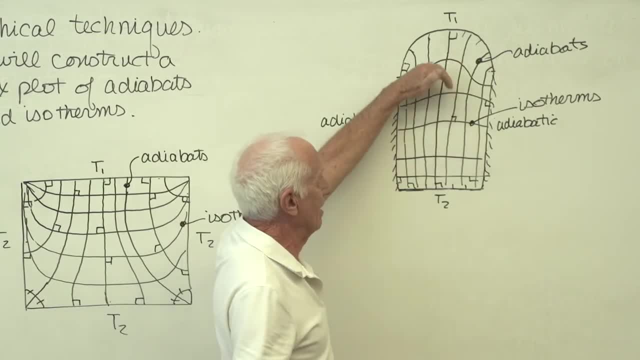 They bulge out near the top. They bulge out because you end up at the top it's a semicircle, At the bottom it's a horizontal line. So they change horizontal line. they start to bow up until they get way up here. 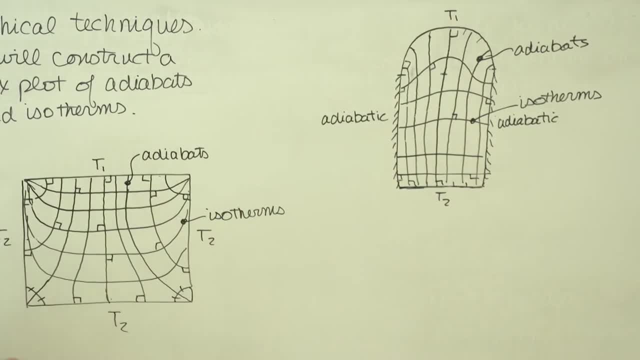 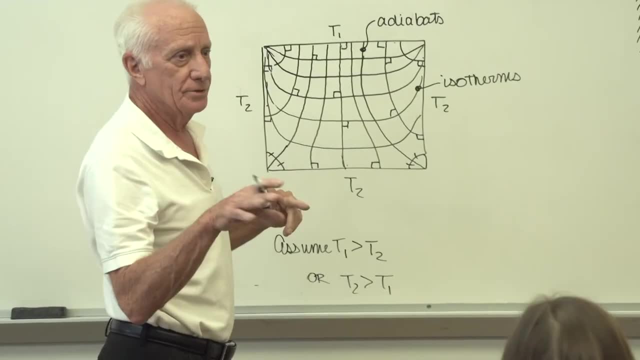 and then they're a semicircle. That's why I like to draw the heat flow lines first. I have more intuition for that than I do the isotherms. What's your question, By the way? yeah, we use that rule, so we know that. 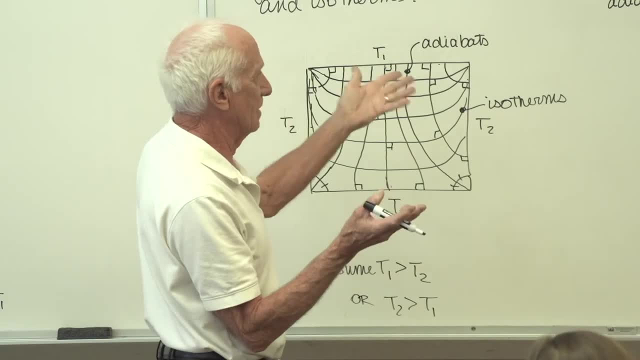 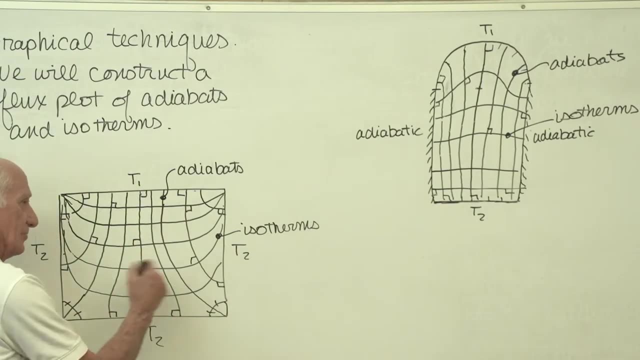 Let's see: was there anything else? It doesn't matter which one's hot and cold Say T2 is bigger than T1 or vice versa, doesn't matter. Why are they cross at right angles in the middle? The math tells us they do. Laplace equation. 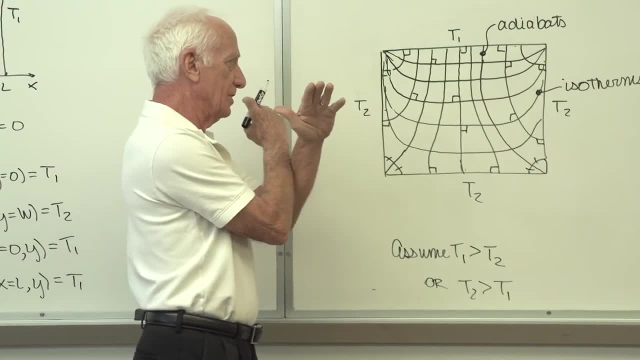 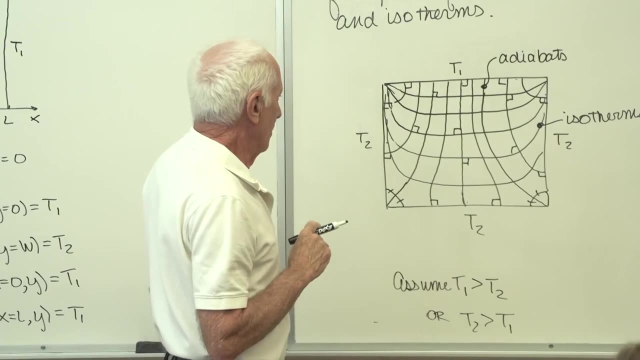 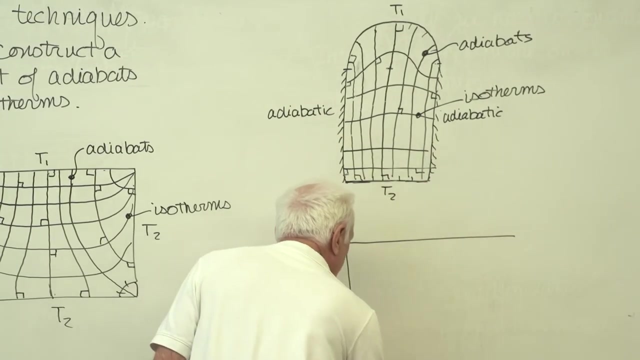 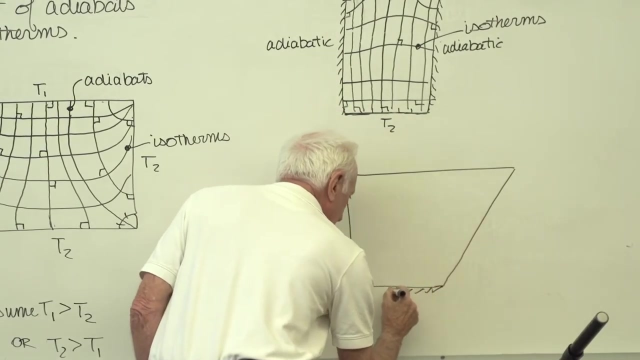 Those two functions cross at right angles. They're normal to each other within the boundaries of the solid. That conclusion comes from that math over there. Okay, So now we'll take this one. Let's see the bottom on. this one is adiabatic. 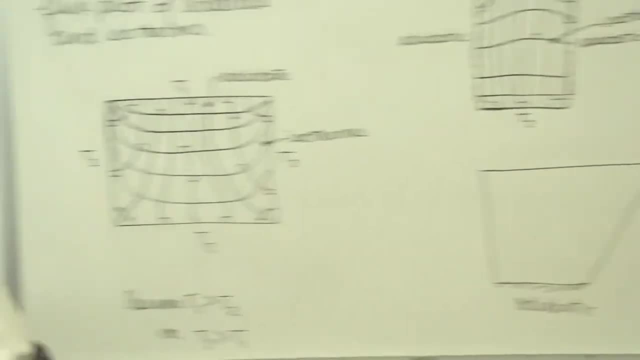 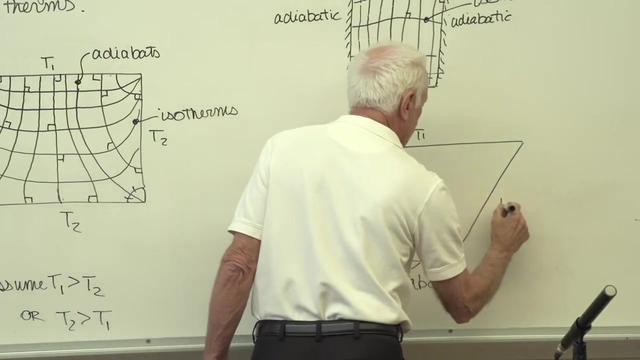 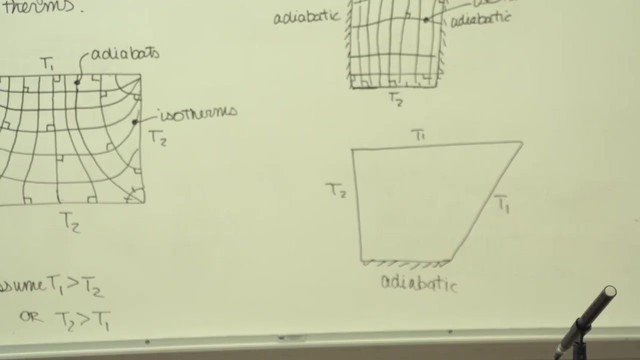 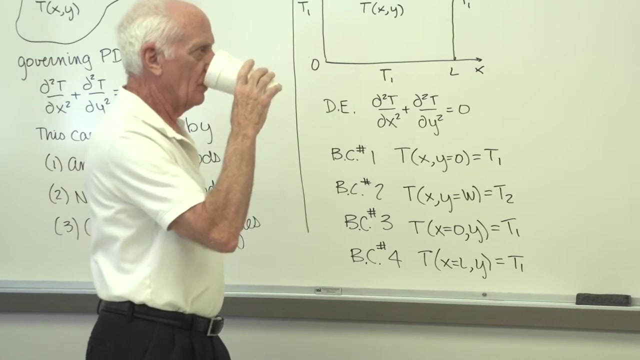 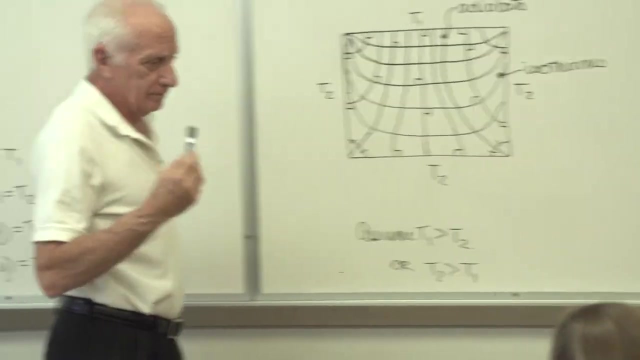 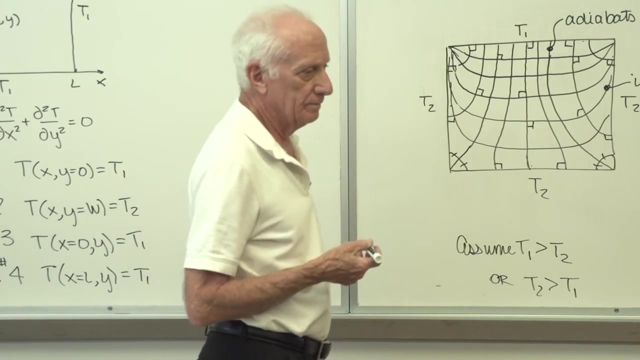 and one side is at T2, the other sides are at T1.. Draw the flux plot, Rule 1, find lines of both geometric and thermal symmetry. There are none, Didn't help me. What am I going to do now? 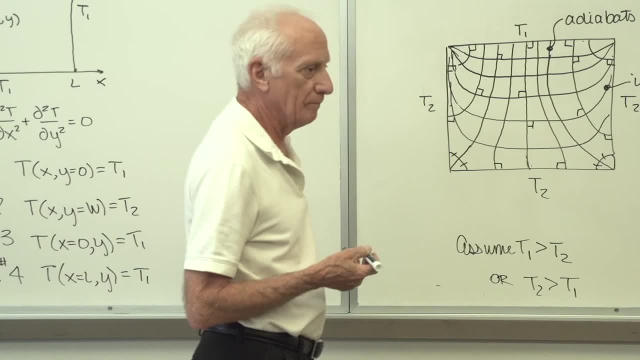 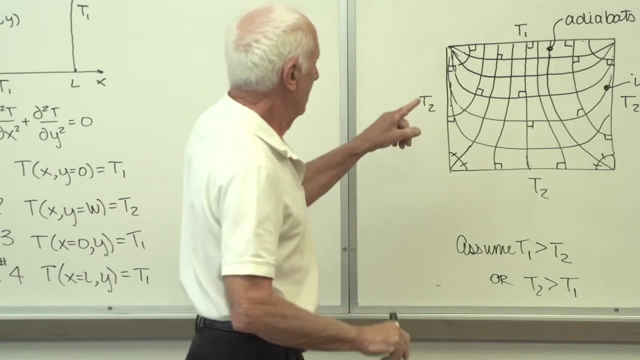 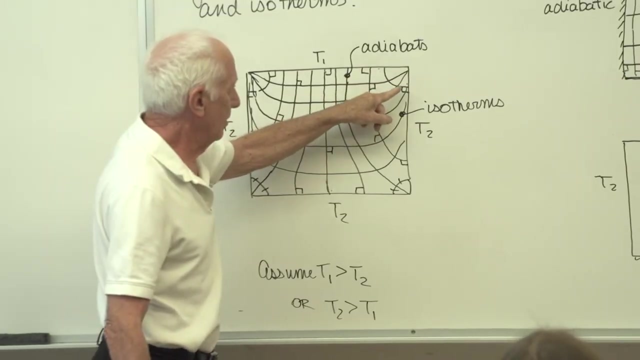 Well, I'm going to assume T2 is bigger than T1.. In a corner where T1 and T2 come together, how does the heat flow? Here we are: T1 on top, T2 on the right, the heat flow line. 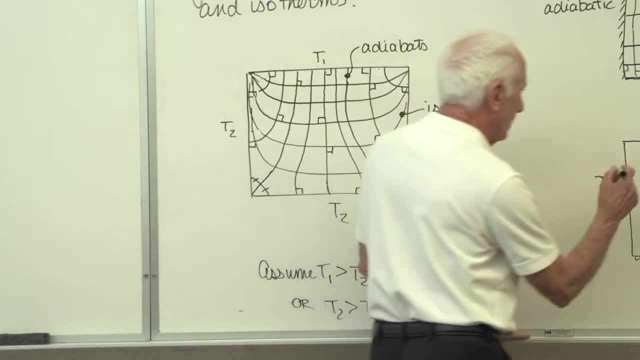 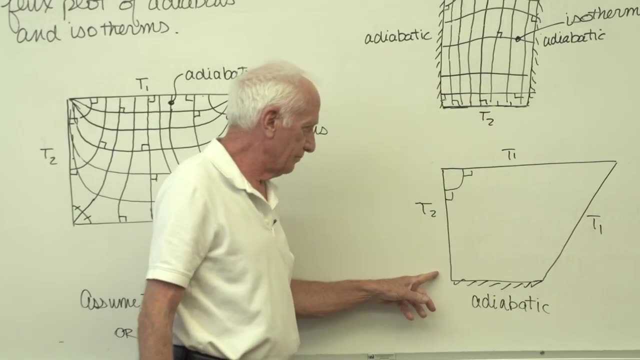 almost looks like a quarter circle right there. Fine, draw it T2 to T1.. Got it? Let's take the bottom. Go near the bottom. Heat comes in from T2, it's hot. It's going to go out T1 where it's cold. 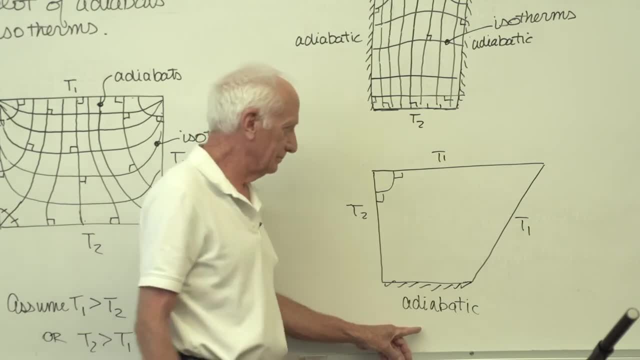 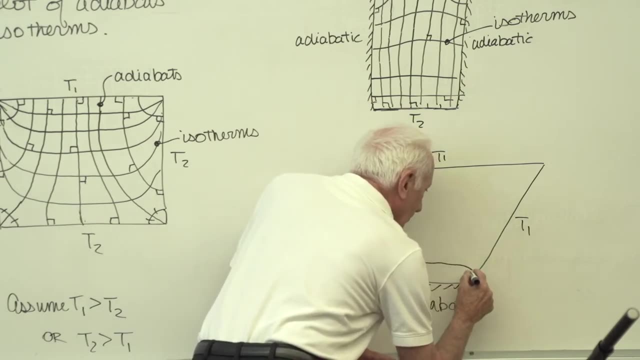 but it can't get out the bottom adiabatic. Guess what it's going to do. Well, you know what it's going to do. Go straight until here. but where it intersects the isothermal boundary, the adiabats intersect at a right angle. 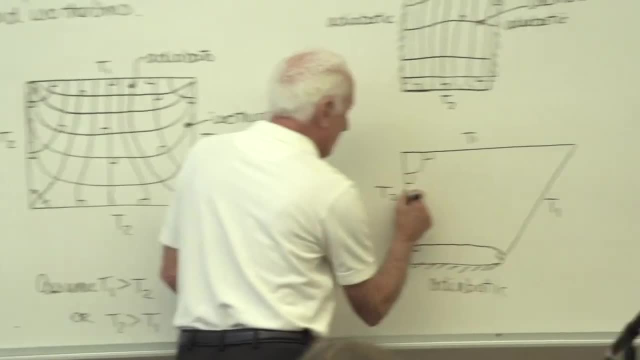 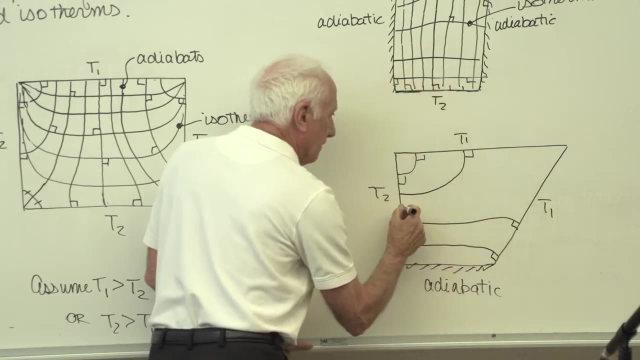 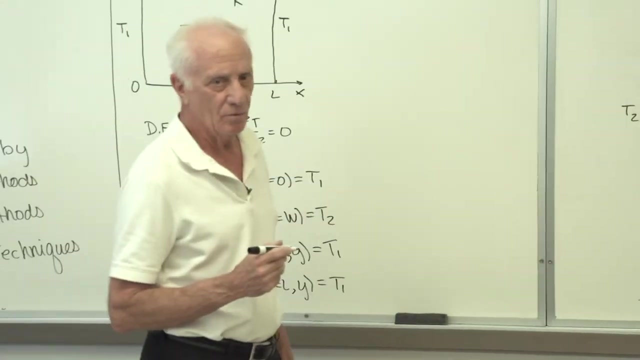 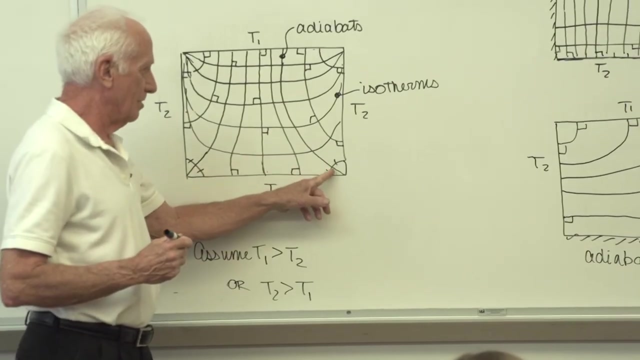 Okay, Draw some more Over here, Draw some more. Uh-oh, I'm approaching an isothermal corner- T1, T1.. Down here, I'm approaching an isothermal corner T2, T2.. Guess what it does. 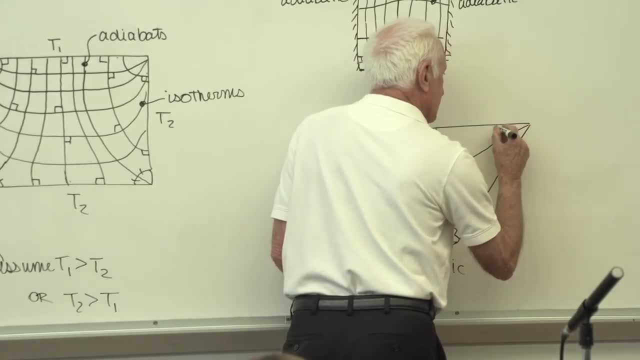 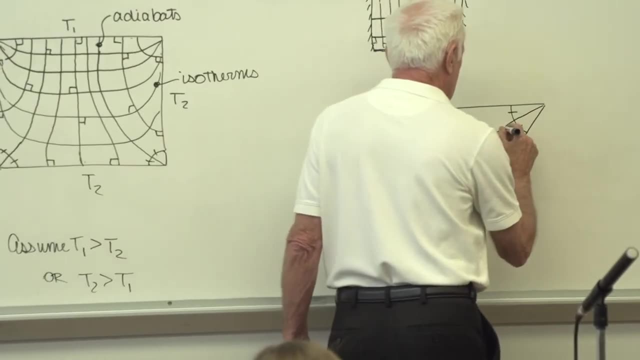 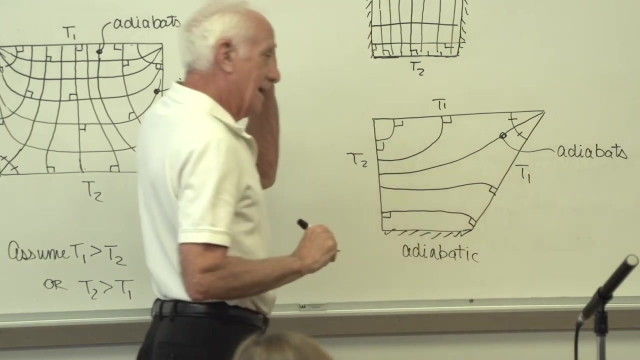 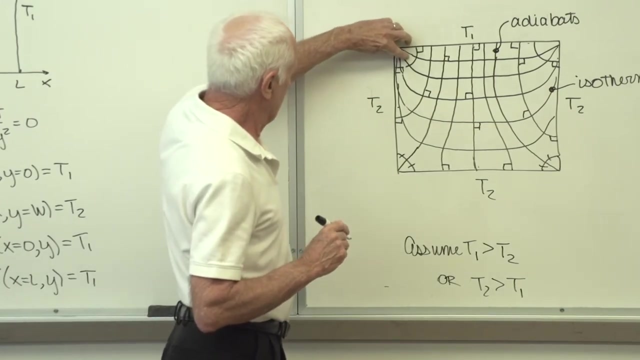 Rule says the adiabat bisects the isothermal corner. Okay, There they are. Those are the adiabats. Now the isotherms. Look at the picture here When they come out of the corner. 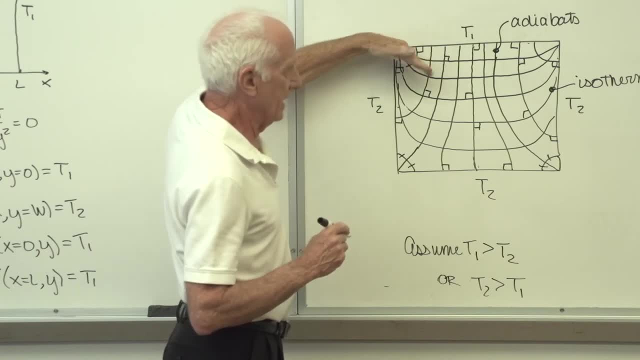 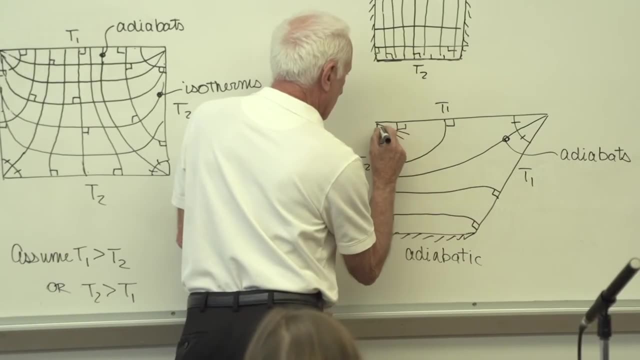 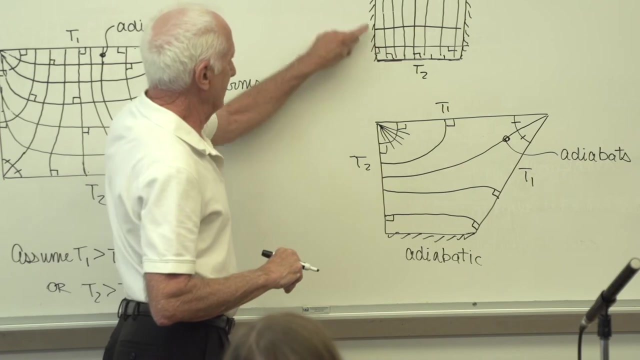 the isotherms come out. different temperatures in a fan pattern, fan pattern They come out and they look like this: When they get to an adiabatic boundary, the rule says adiabatic boundary- isotherms- right angle. 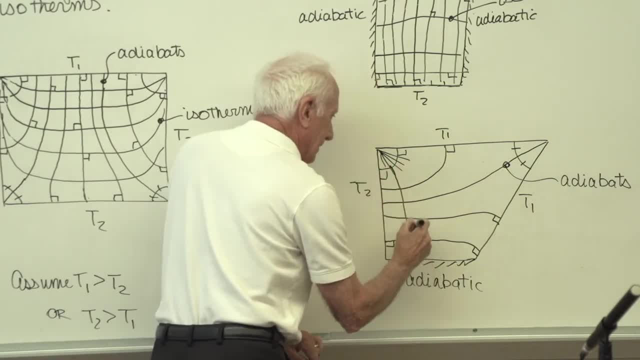 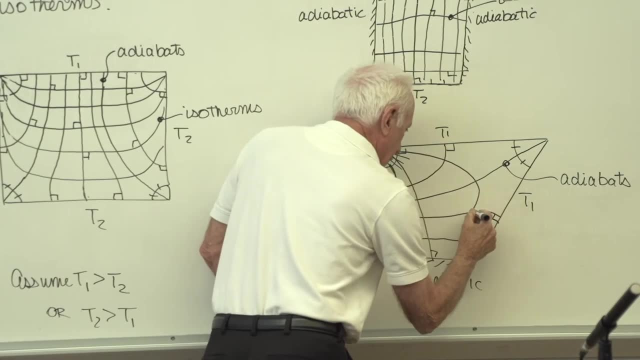 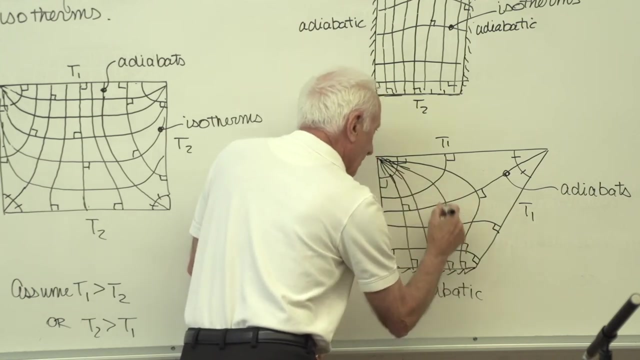 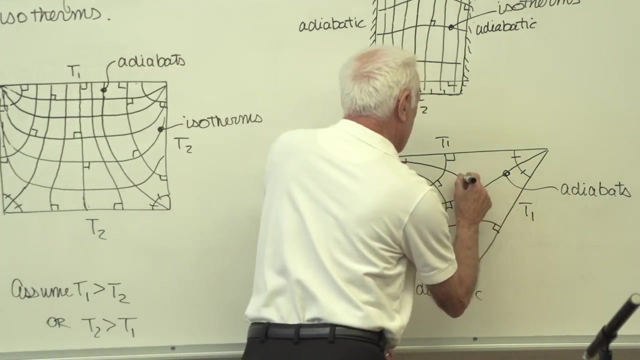 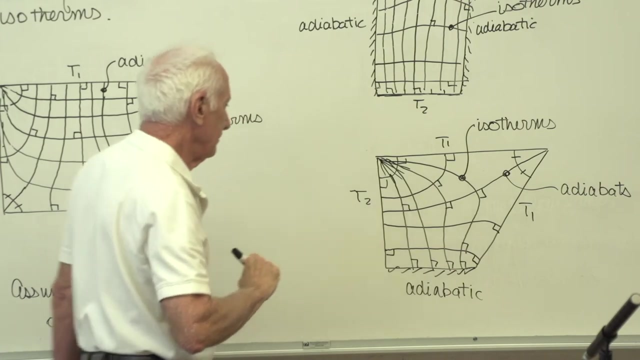 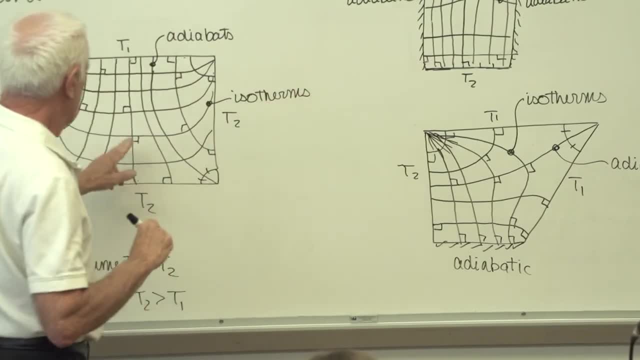 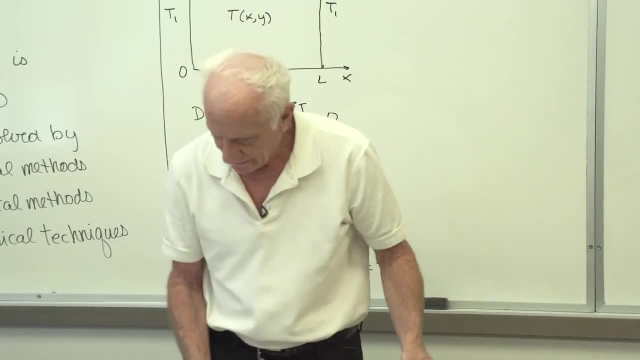 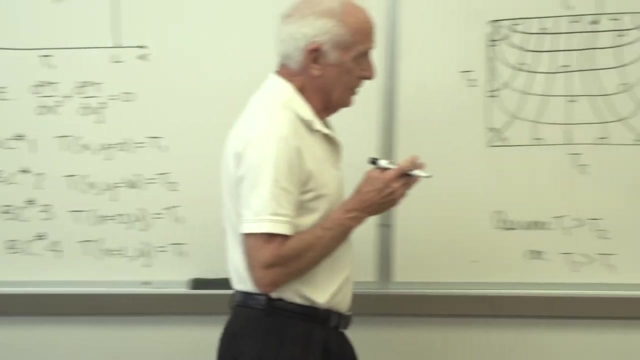 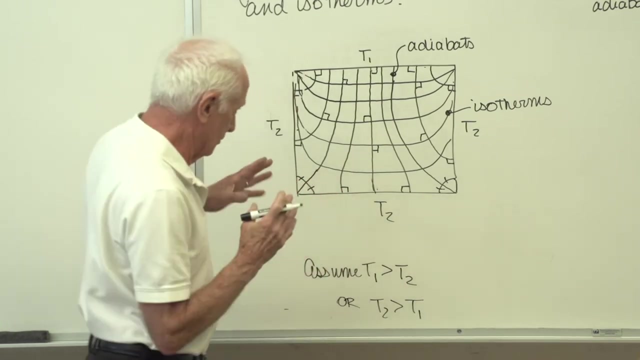 This guy symmetry, this guy symmetry. Now that's drawing the flux plot. Now we can also say: well, does it help us get the heat flow? Yeah, it can. It depends how much patience you got You've got to construct this thing. clearly. 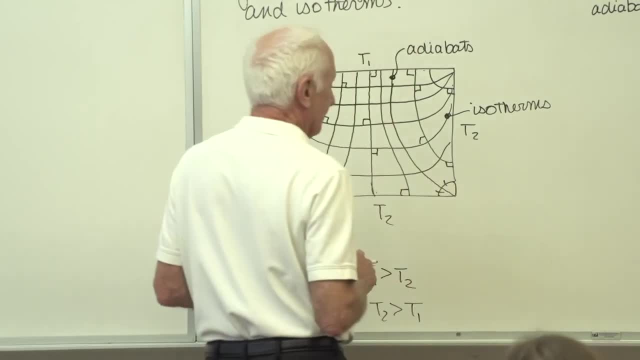 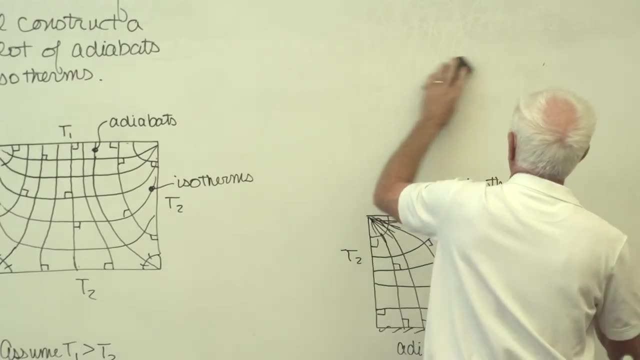 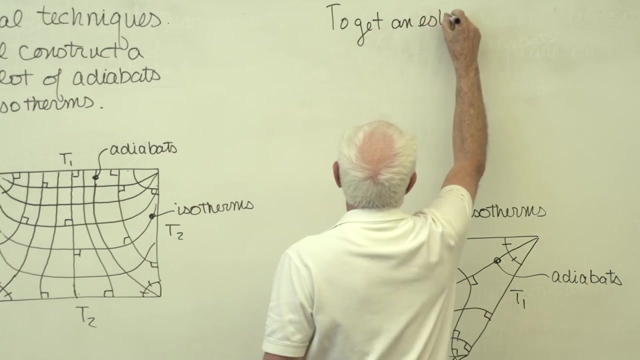 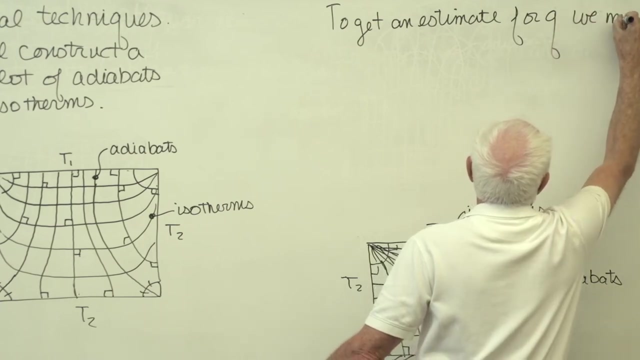 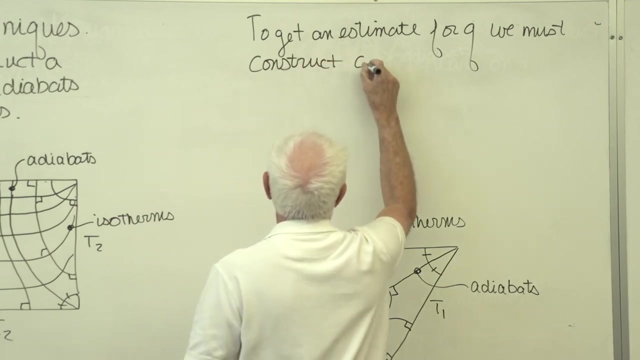 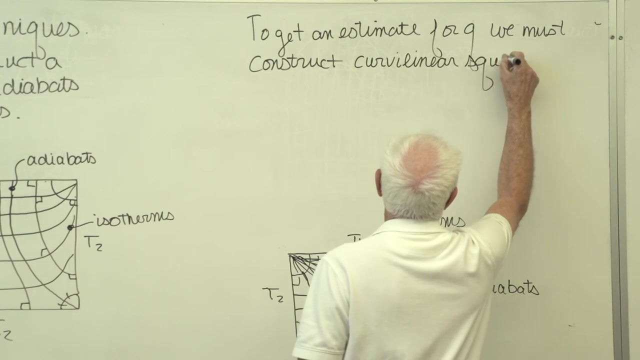 I think. I think I'll put this here. We don't need this anymore. We'll use that guy To get an estimate for Q we must construct. we call curvilinear squares, So here's a curvilinear square. 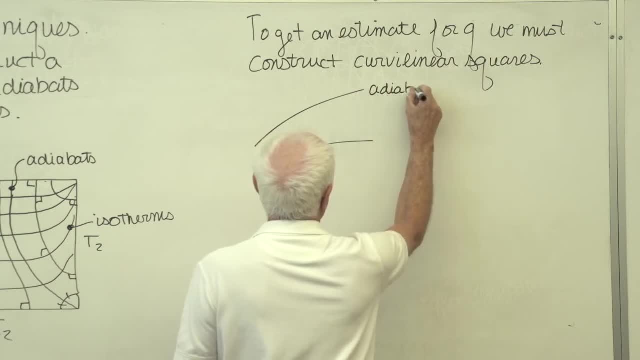 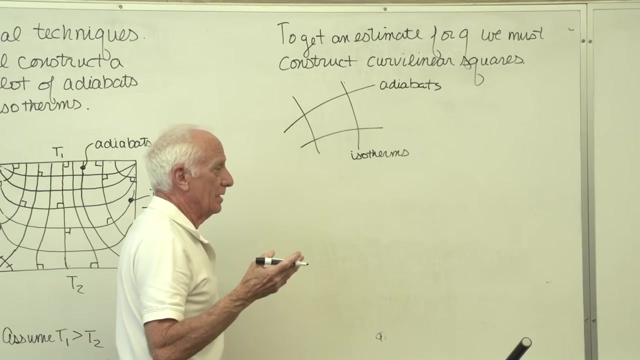 Here's the adiabat, Here's the isotherms. Of course, they're called curvilinear squares because the sides are curves- Curvilinear square. How do I know when I've drawn a good curvilinear square? 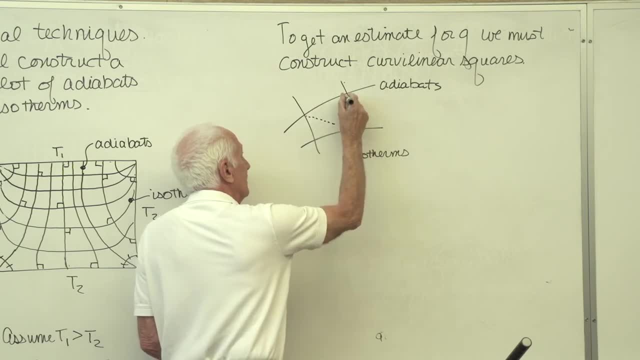 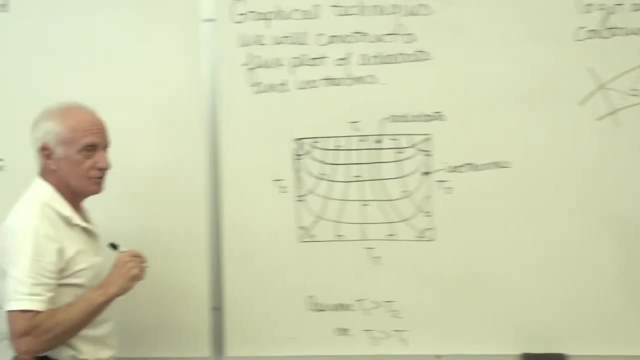 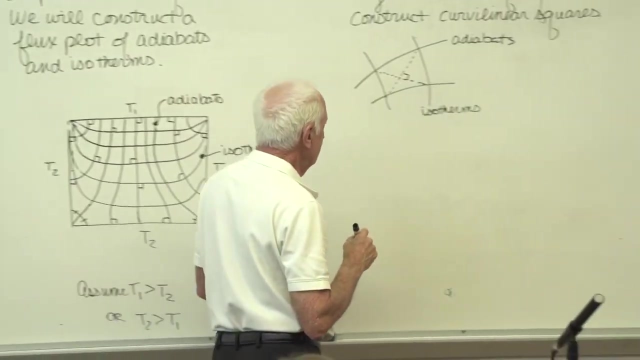 When you have draw two diagonal lines. If those lines cross at a right angle, you've got, by definition, a good curvilinear square. Curvilinear square is the diagonals cross at right angles. If you do that with those curvilinear squares, 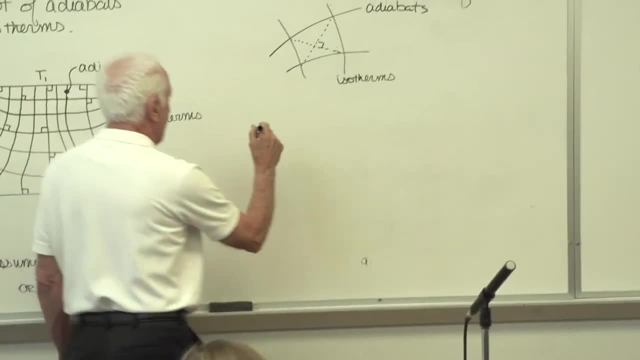 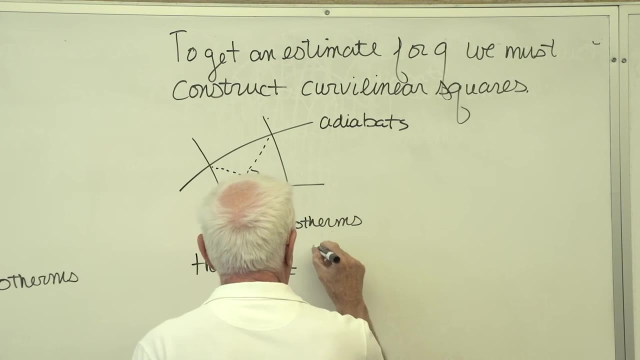 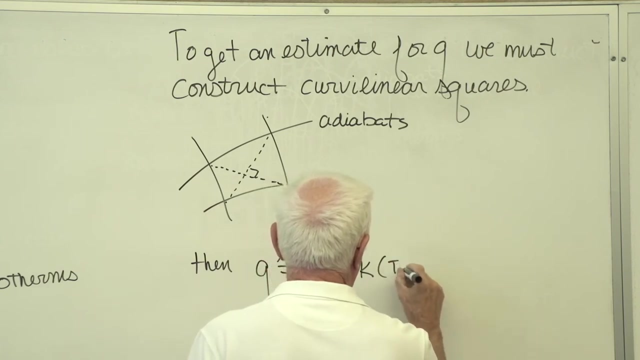 then we can get an estimate for Q. Now, in this case, we're going to use the right angles. We're going to use the right angles. We're going to use the right angles Now, in this equation I'll mention in just a minute. 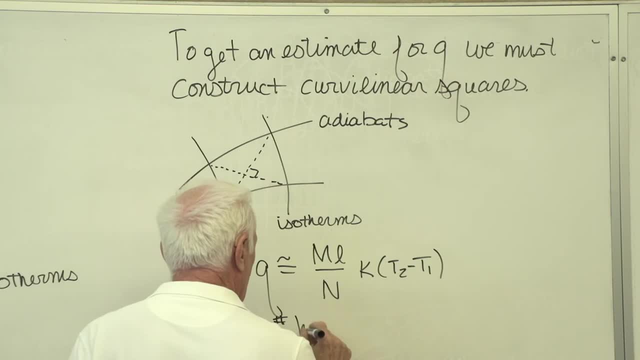 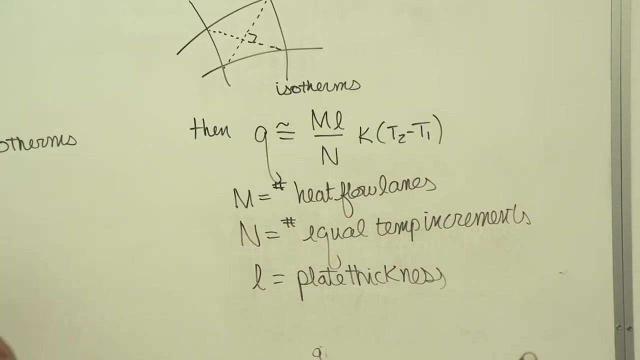 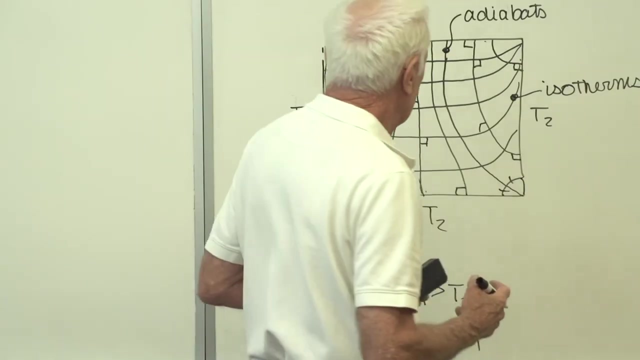 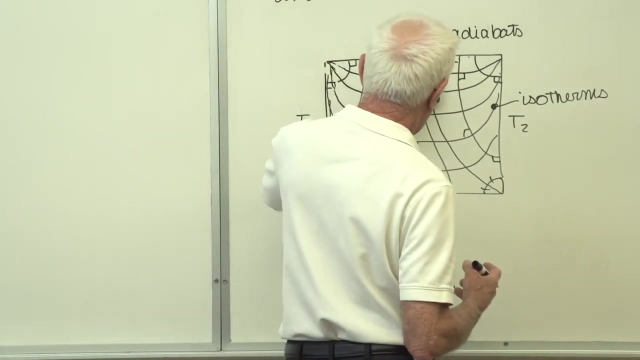 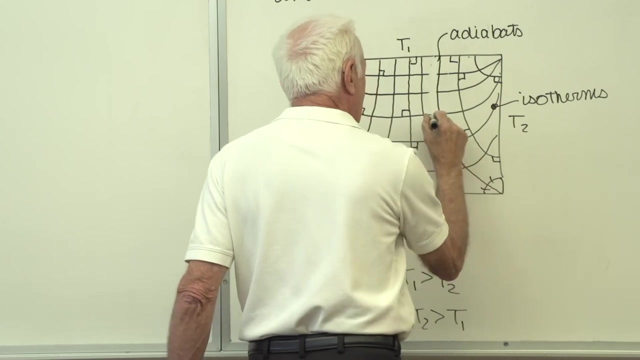 but M equal the number of heat flow lanes, N is the number of equal temperature increments and L is the plate thickness. So, but it's only true if you've drawn reasonable curvilinear squares. So here's my picture. I have to have on my desk a big fat eraser. 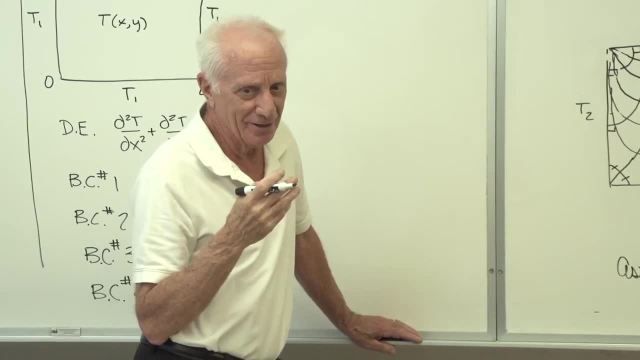 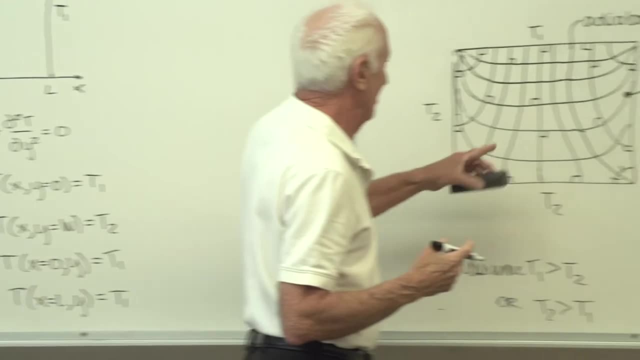 Because I know the first time I use a pencil, never a pen, of course, the first time I draw, this is not going to be right. So I take my eraser. I say, oh, that line didn't work, I erase it and redo it again. 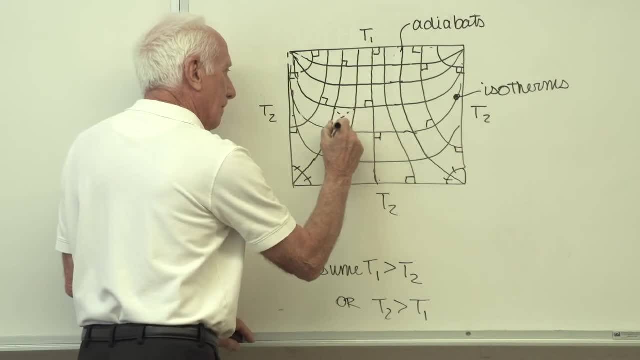 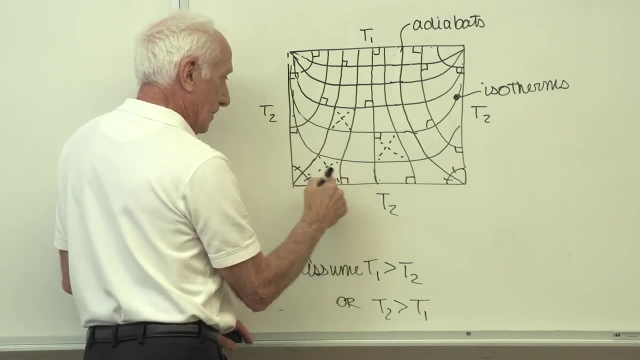 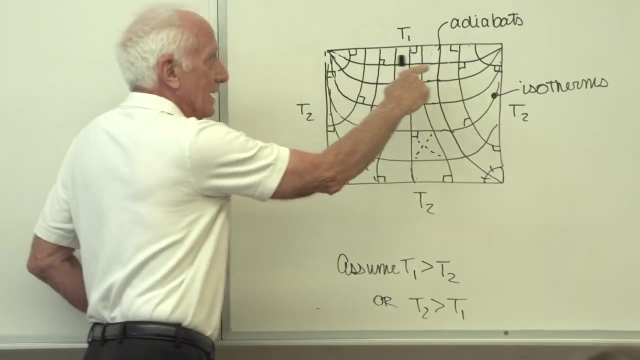 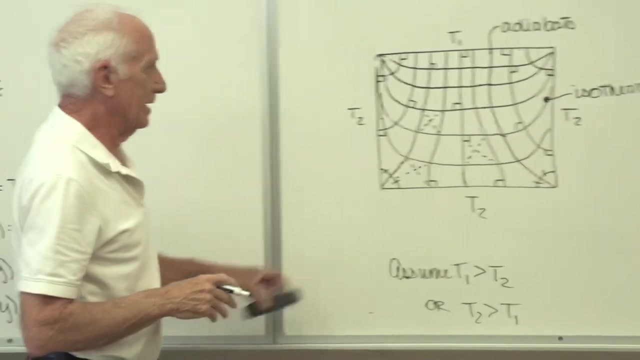 and check for curvilinear squares. Good, I check for curvilinear squares. You're never going to get up in that corner, so don't worry about that corner. Close to that corner. So you check several places. If you're not happy, get out your big eraser. 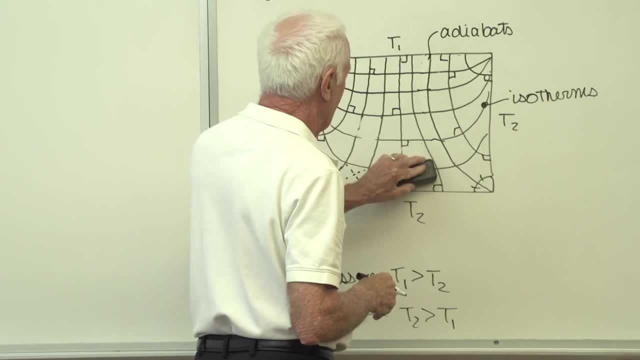 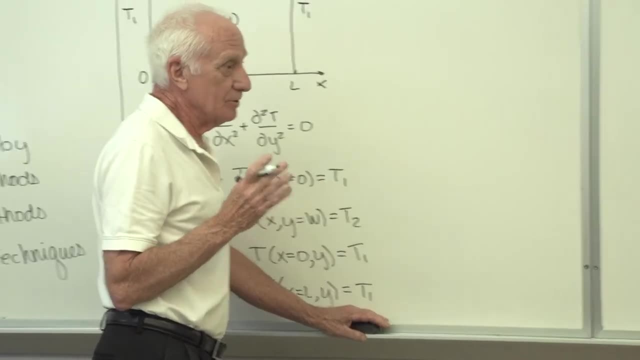 erase it and try again until you say: oh gosh, I worked off for 10 minutes, I'm tired, It's pretty good, I'm going to stop here. I understand, Do your best job, though The closer you get to drawing curvilinear squares. 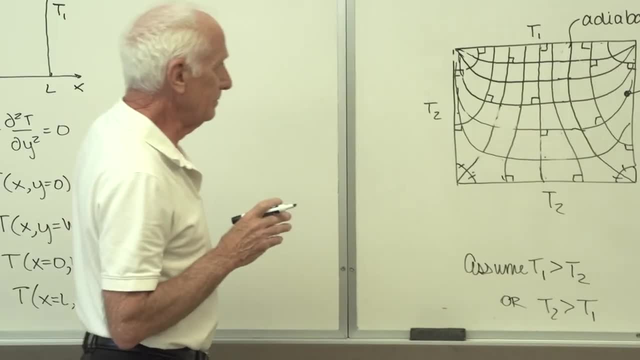 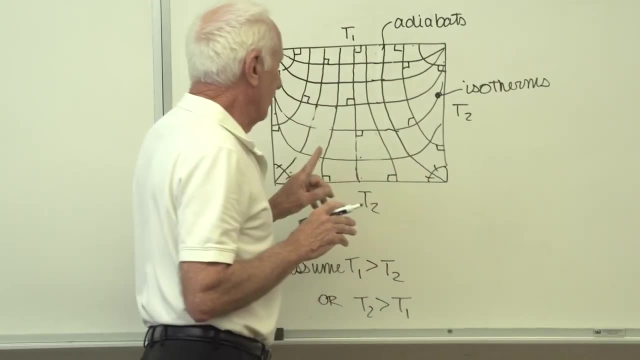 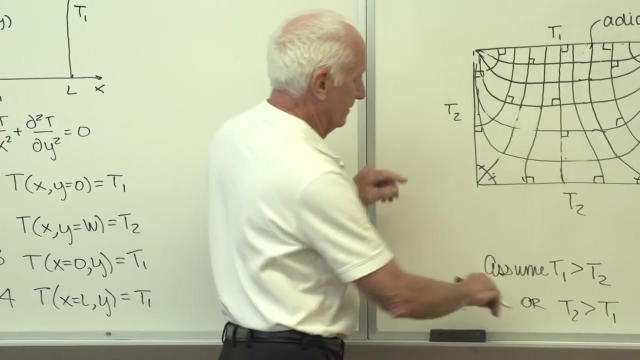 the better that Q will agree with the exact answer. So for this picture here, number of heat flow lanes. A heat flow lane is like a heat flow highway, heat flow road, whatever you call it. Here's the deal. Heat comes in here at the hot temperature T1.. 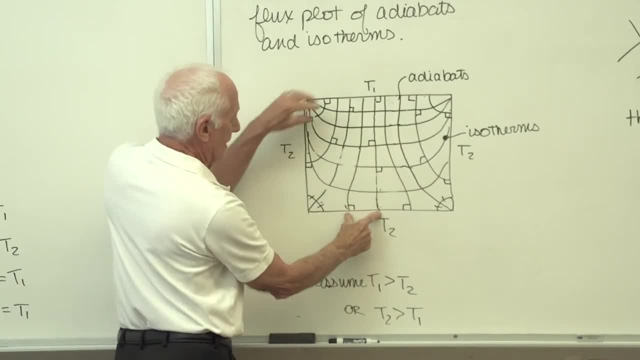 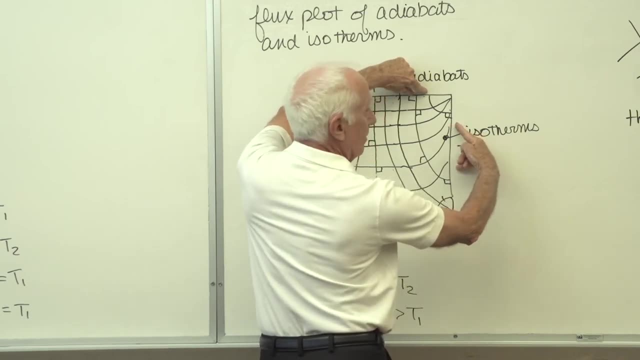 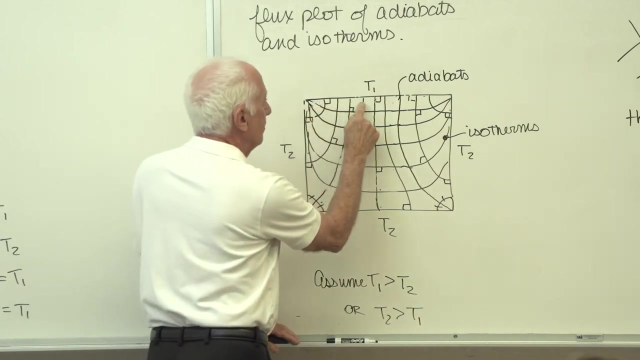 Where does it go out Down there at T2.. That's a heat flow lane. Heat flow comes in here. Where does it go out? Way over here on the right side It goes like that: Count how many there are: 1,, 2,, 3,, 4,, 5,, 6,, 7,, 8,, 9,, 10.. 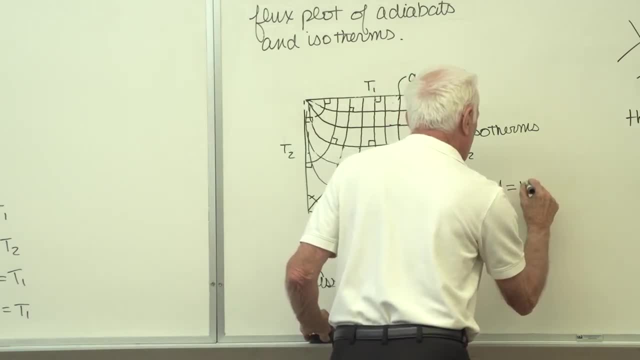 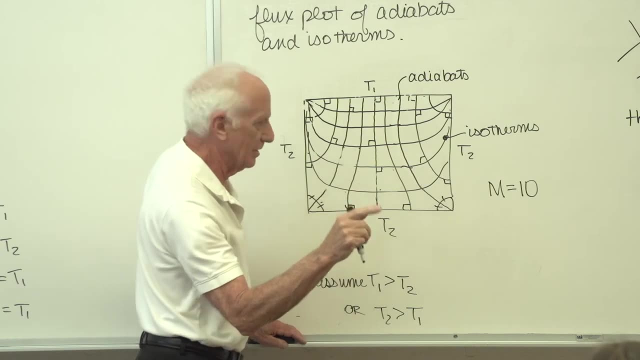 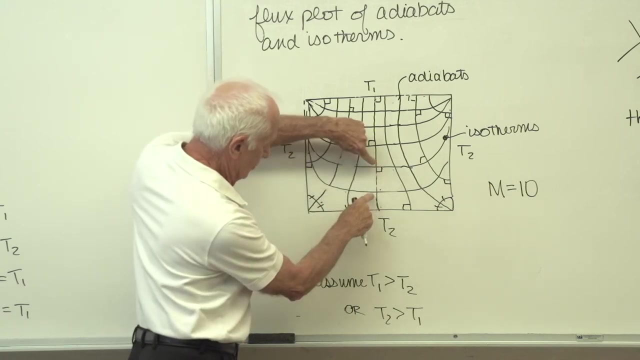 For that picture M equal 10.. 1,, 2,, 3,, 4,, 5,, 6,, 6 increments Equal temperature increments. Don't say lines, don't count lines, count increments. One increment: 2,, 3,, 4,, 5,, 6.. 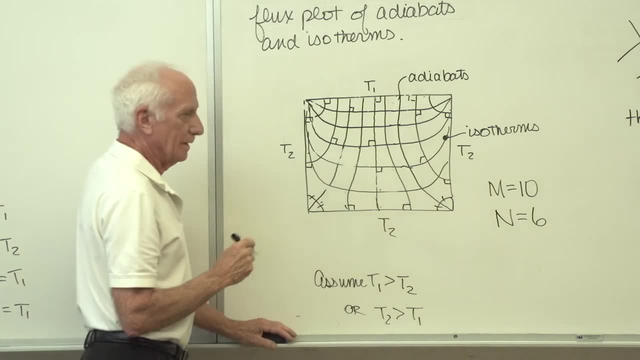 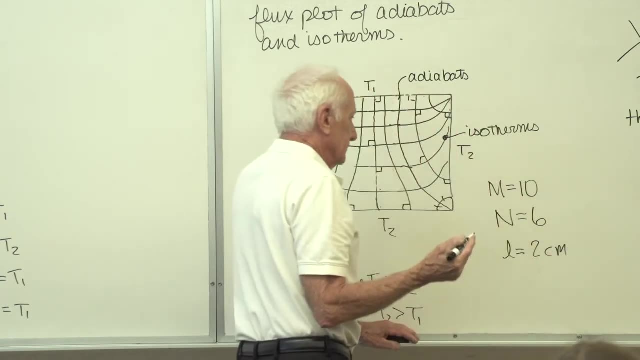 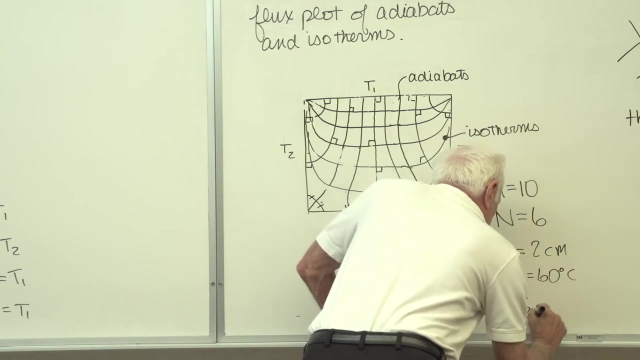 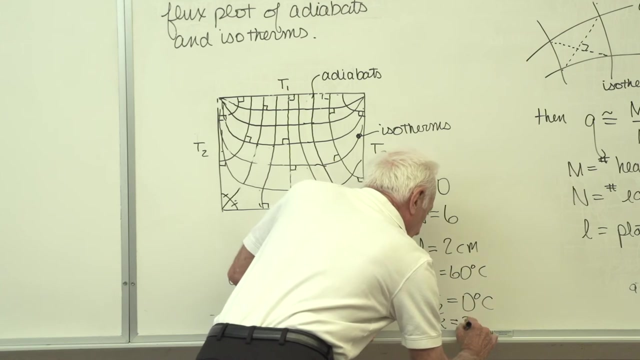 I don't know. Maybe we'll call the plate thickness. you might call it two centimeters. for instance, You might call T1 equals 60 degrees C, T2 equal zero degrees C, I don't know. You might say K equal 200 watts per meter degrees C. 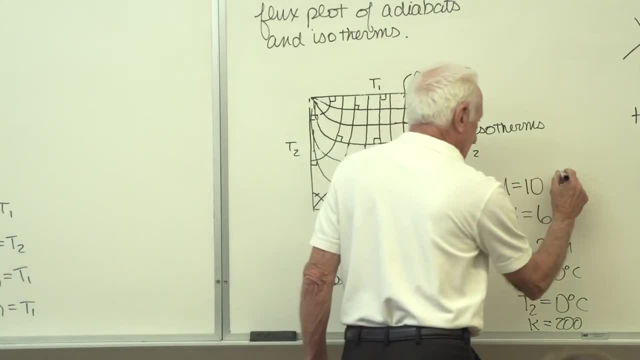 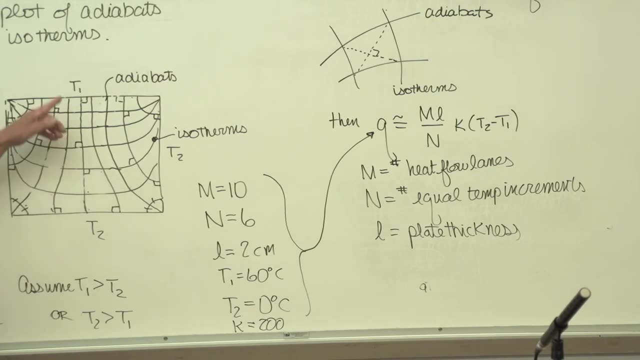 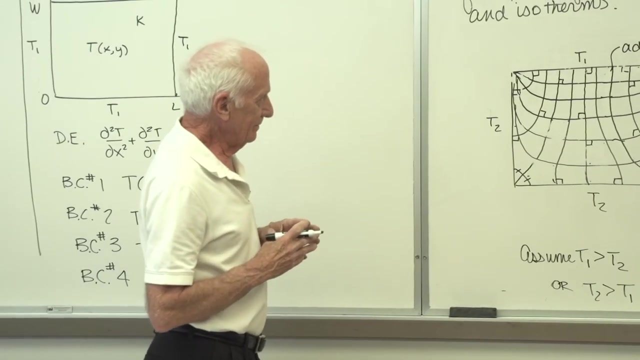 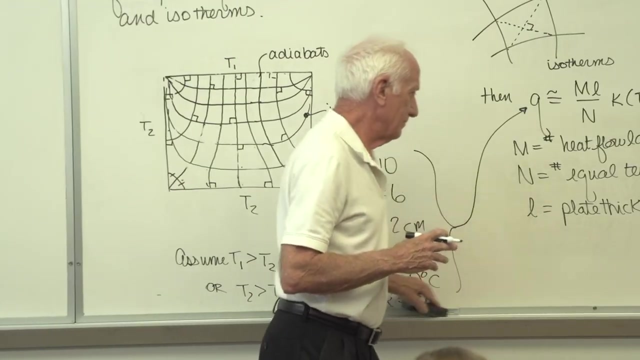 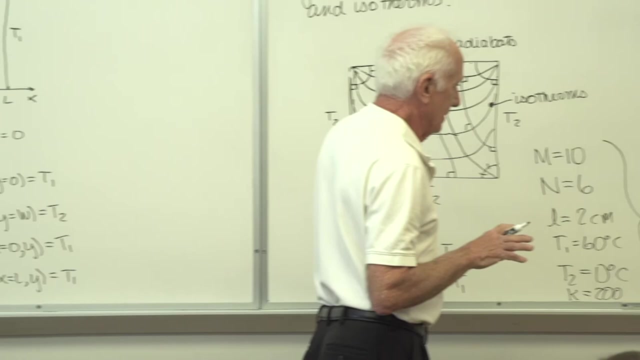 You've got the quasi conditions there. You put all those stuff into that Q and you've got an estimate of how much heat is transferred from the hot surface at 60 to the cold surface at zero. We get an estimate of that, also a way to get an estimate of temperature. 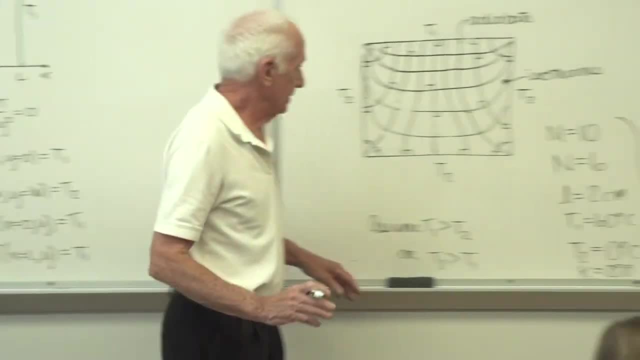 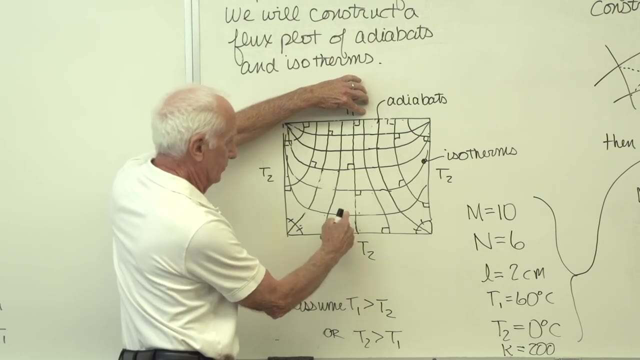 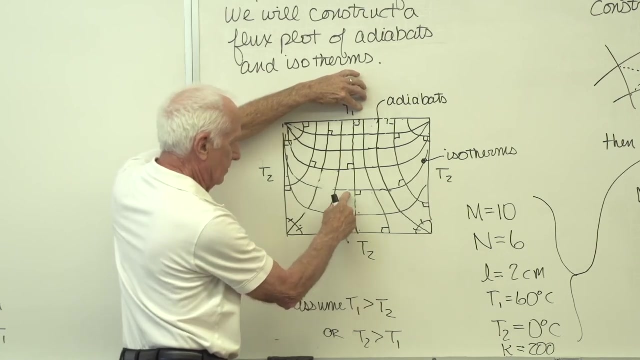 So this is 0,, this is 60.. Count the intervals 1,, 2,, 3,, 4,, 5, 6.. If that's 0 and that's 60, here's 0,, 10,, 20,, 30,, 40,, 50,, 60.. 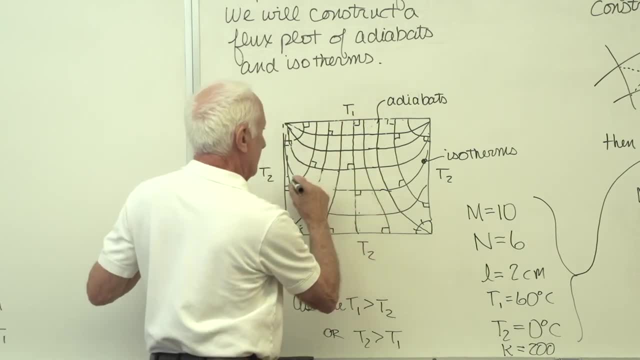 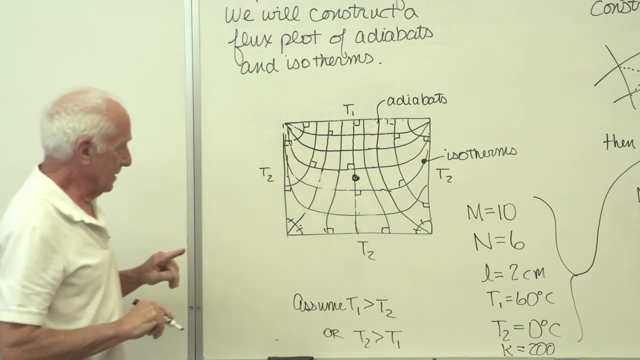 If somebody asked me what's the temperature in the middle of the plate, Middle of the plate, If I'm a good sketcher, I say okay, let's count again: 0,, 10,, 20,, 30.. 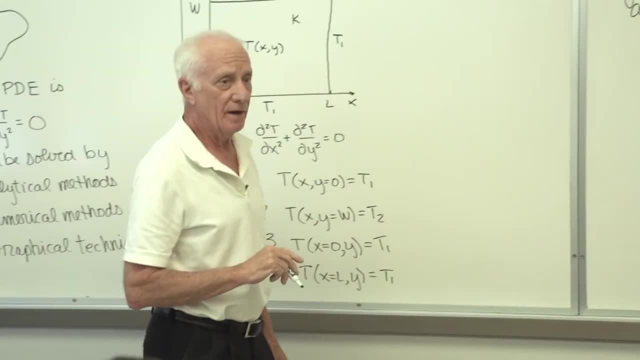 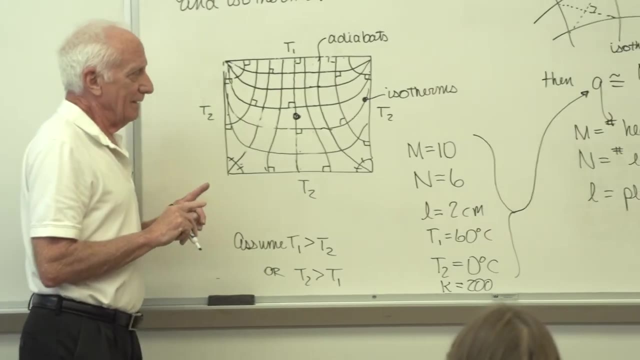 I say 26 degrees right there. Good, Okay, fine, That's an estimate of the temperature in the plate at that point. So it allows you also to get an estimate of the temperature. Say, well, okay, that's good. 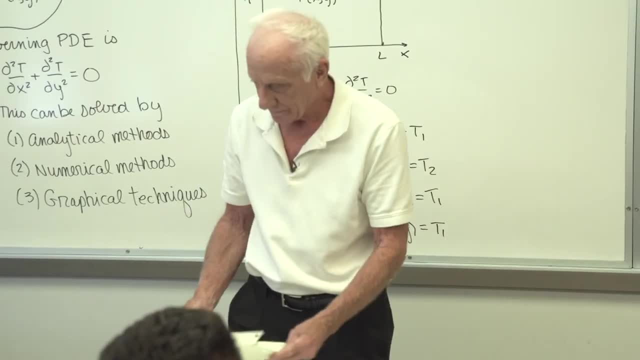 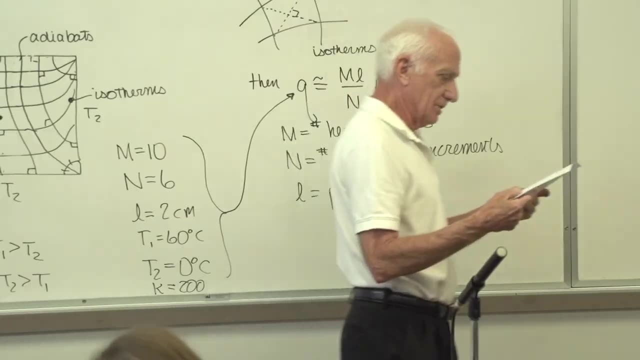 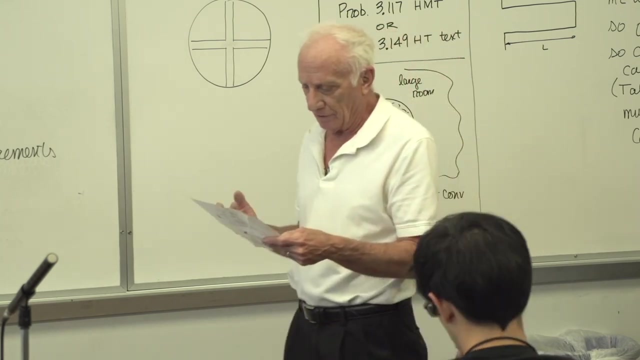 but like: so what? Well the? so what's at the bottom of the page here? It says the graphical approach has two important uses. Number 1, it develops an engineering intuition for the temperature field and heat flow in many 2D conduction problems. 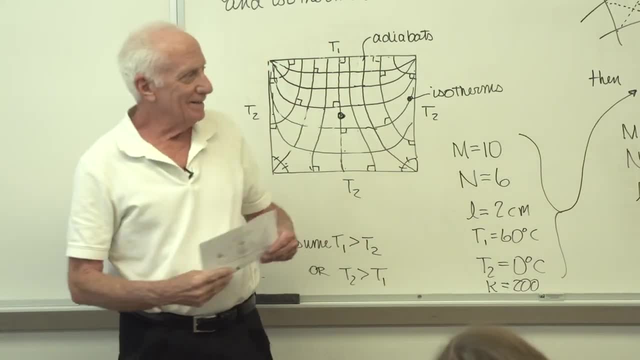 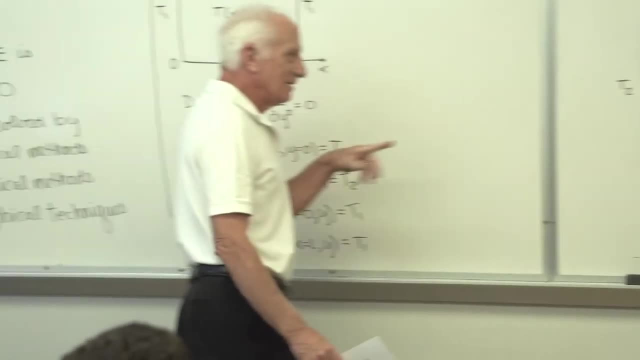 I don't need to solve the PDE to make that really good drawing. I don't need to get the estimate of 26 degrees here to solve this guy. No, no, If I can sketch this reasonably, I can give you a good estimate of. 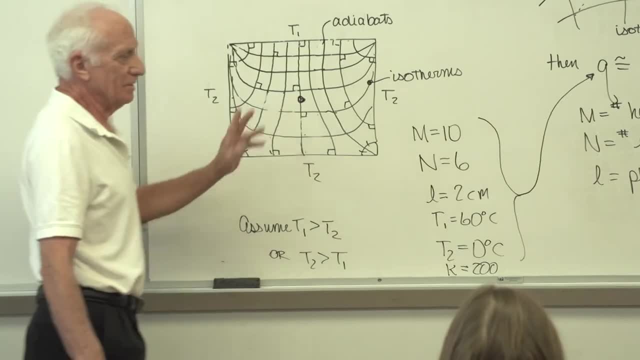 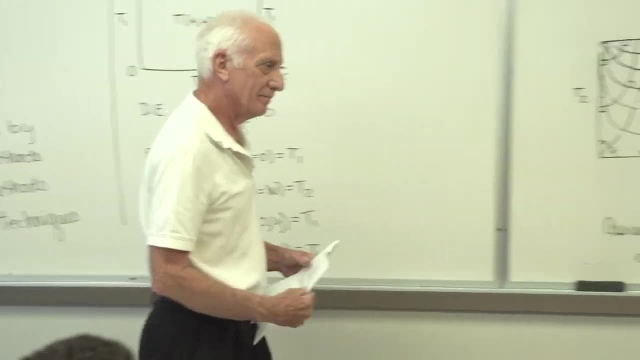 that temperature or that heat flow. Q. You could be sitting with coffee at a coffee shop on a napkin and sketch that thing out. I don't need Excel to do that. No, you don't. It gives you a good engineering intuitive field. 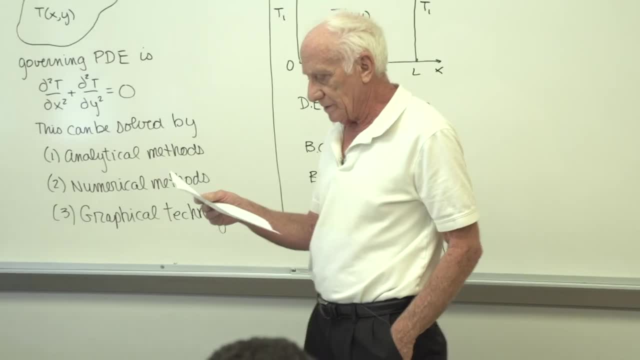 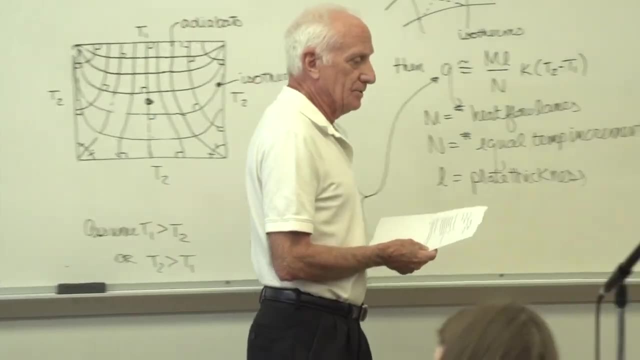 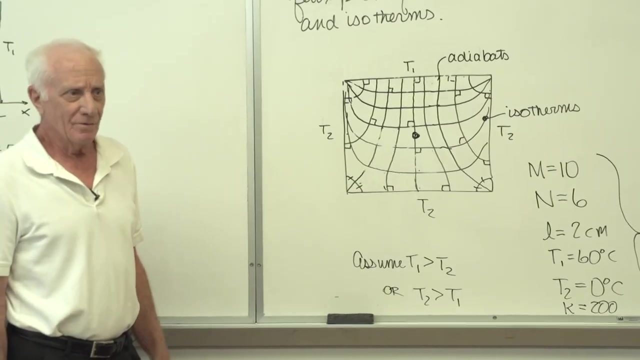 Number 2,. it allows a first estimate of the temperature distribution as a check on the numerical solutions. You program something, it spits out the answers. It tells you the temperature in the middle plate is 59 degrees. You say what? When I sketch it it was 26.. 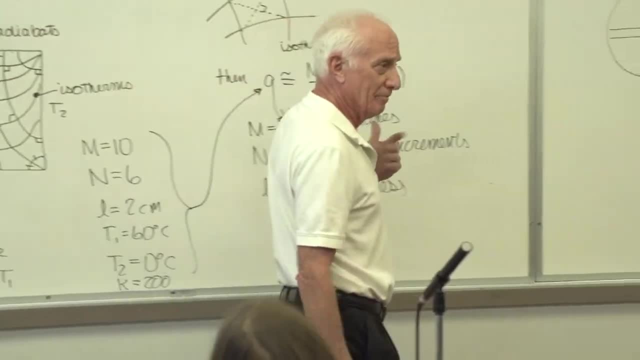 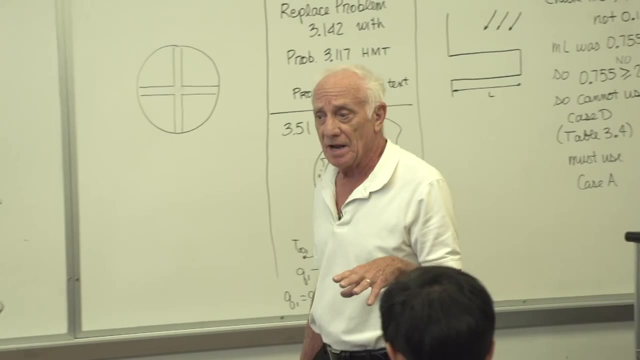 I wonder if my sketching is wrong or if I have a code error in my coding. Oh, you got a code error. believe me, Sometimes you don't know what the computer spits out, if it's accurate or not. on a big, complex case. 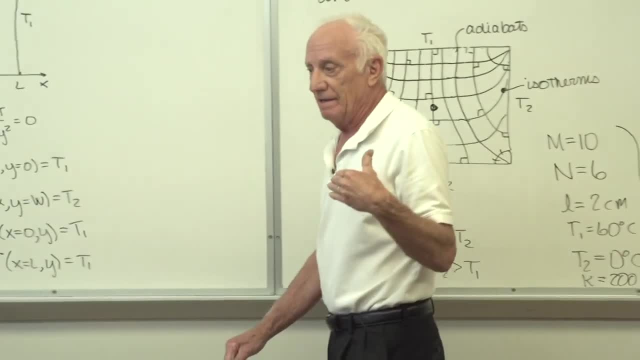 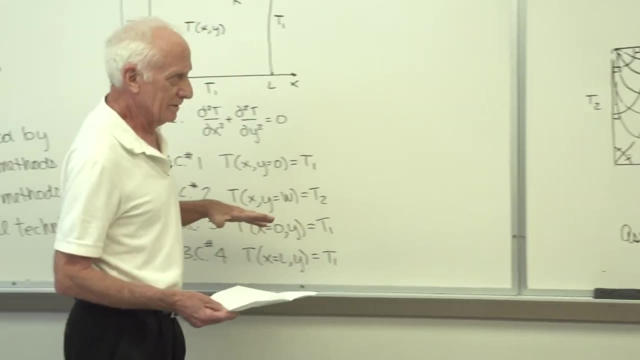 You don't know if it's accurate. So maybe by sketching you can see if your number agrees with what the computer coding spits out. So it has those uses. Very important, not too mathematical, So it has its uses If you want the exact answers. 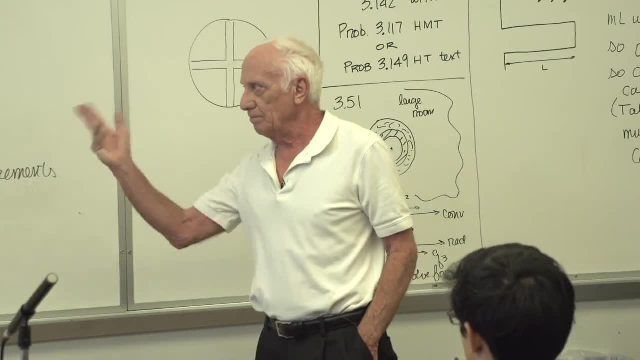 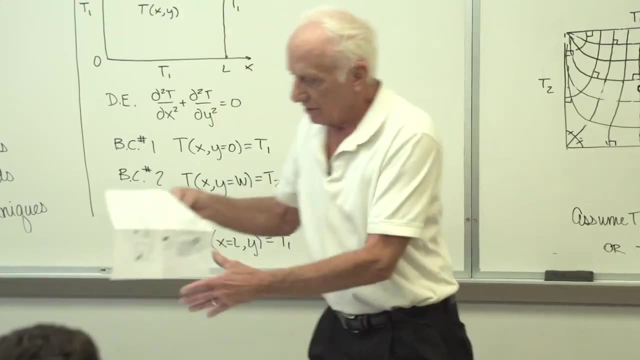 you do it numerically, But you can check those answers with a simple sketch like this to see if you're in the right ballpark, Whether I drew two more here and there's two more given on the back of the page. Here's a square plate with 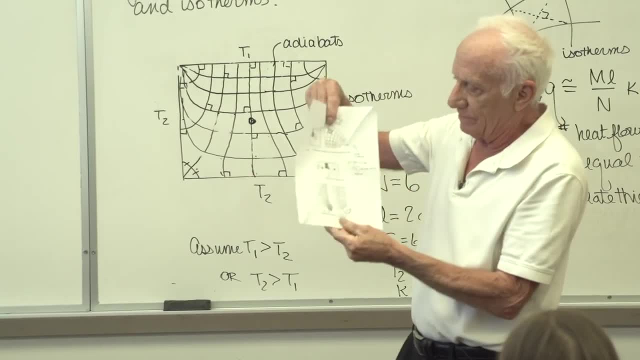 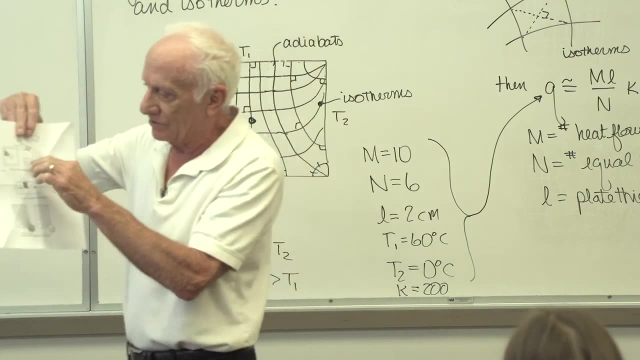 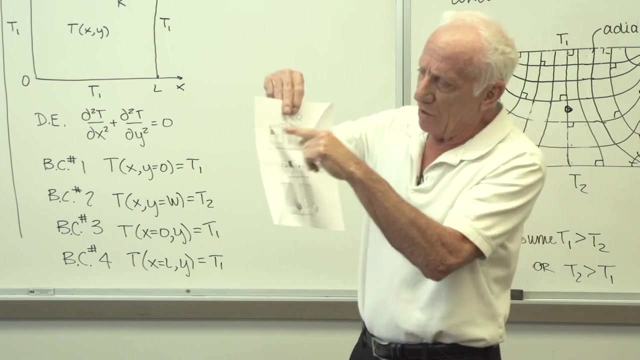 a square hole at 45 degree off from the square plate. You can see he checked for. do we have curvilinear squares? Yeah, really good, You can do the whole thing, but since it's symmetrical, you can just take 1 eighth of it.